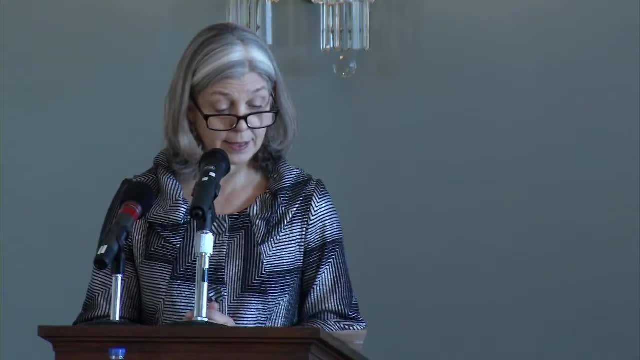 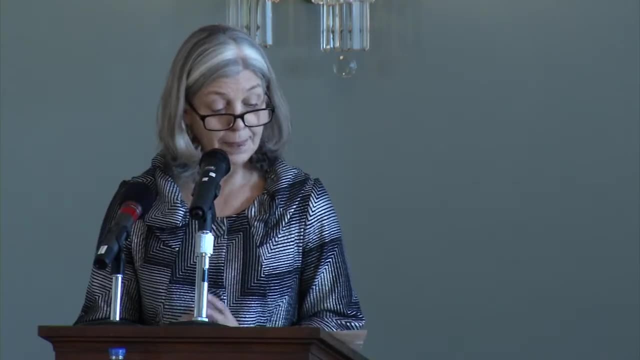 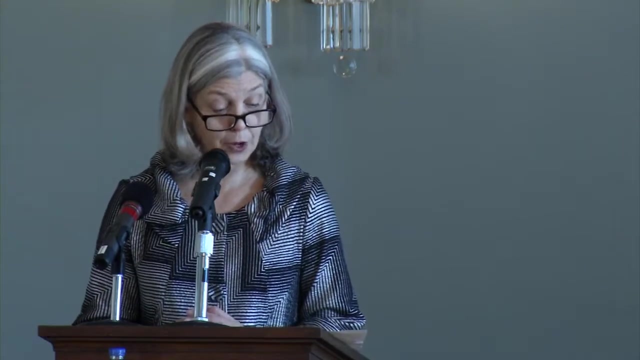 Sellers of Iowa College of Liberal Arts and Sciences. the National Foundation's Iowa Experimental Program to Stimulate Competitive Research. the Ida Cordelia Beam Distinguished Visiting Professorship Program. the University of Iowa Provost Office. the Center for Global and Regional Environmental. 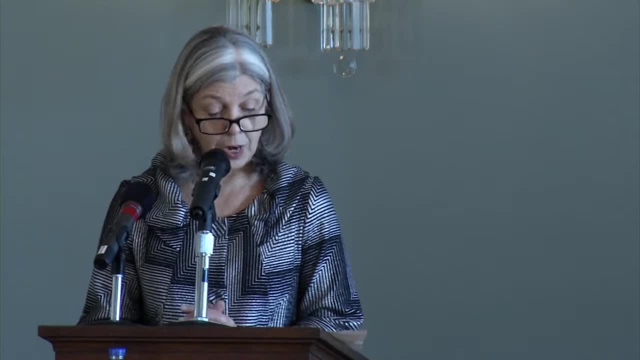 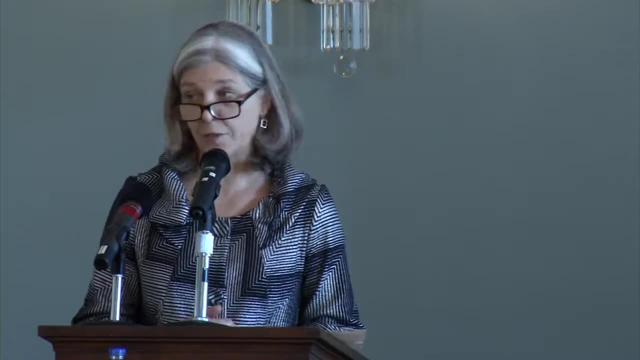 Research here and the College of Public Health and Environment and Health Sciences Research Center, And I hope that you will take a look at the program and the many other departments and offices who generously contributed to make this conference happen. I'll also just mention that 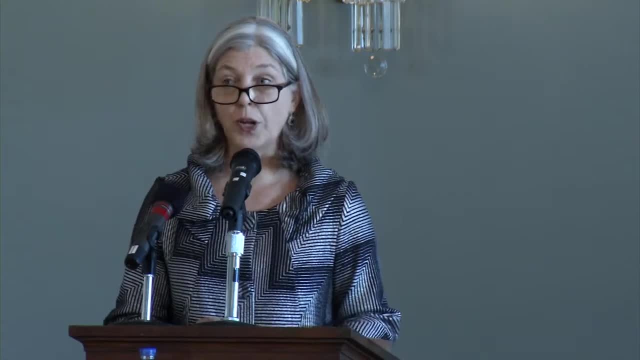 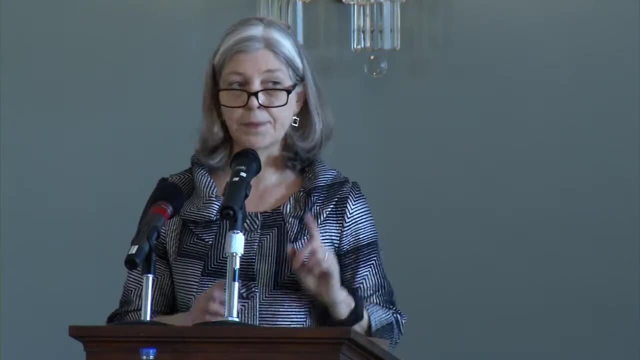 following the lecture and discussion, we are having a reception at Bricks, which is just a few blocks away on Lynn Street, and we welcome you to join us. I'm going to say two words and then turn things over to Todd to get us started. 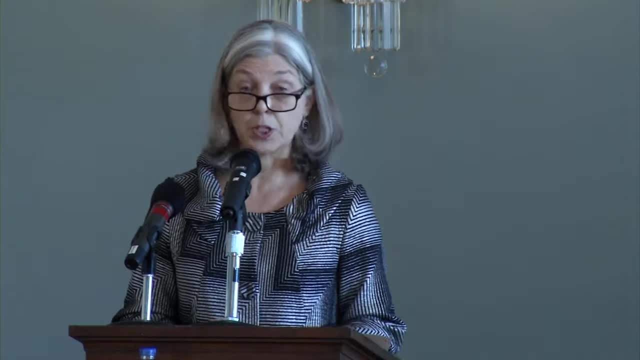 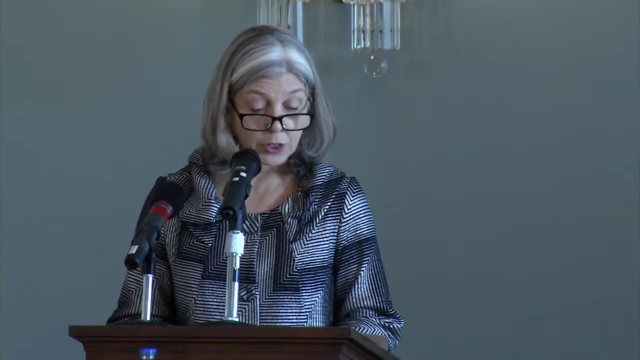 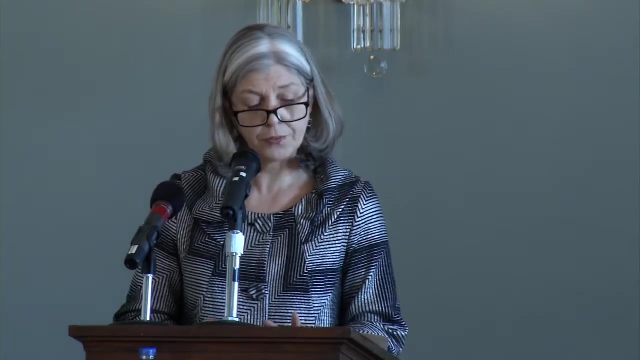 A 2012 essay in the Los Angeles Review of Books bears the title: Welcome to the Anthropocene. The author, David Biello, is the editor who oversees Environment and Energy for the journal Scientific American. In this review, Biello ponders: 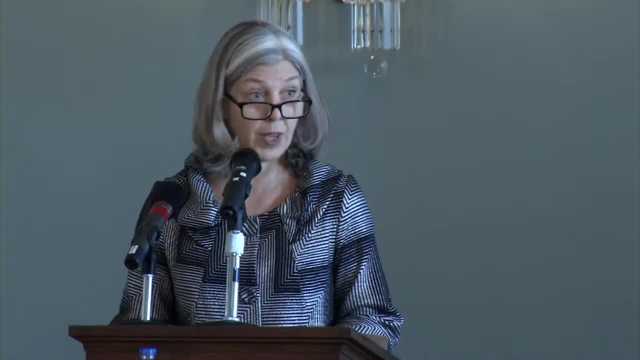 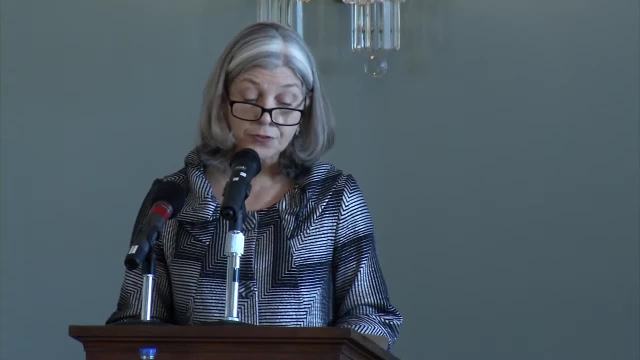 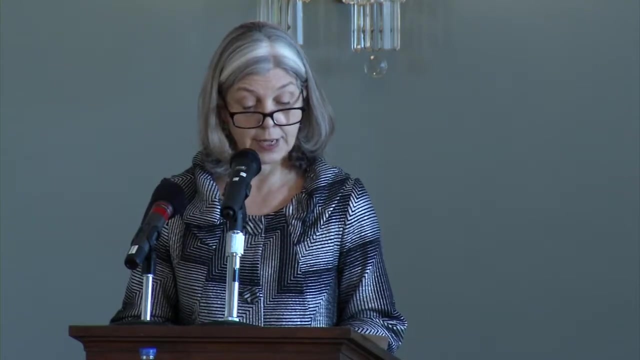 the rising sea of literature about the fate of the environment. His comments are a fitting beginning for our conference. he writes: It is far less interesting to write about all the ways the world is wrong than all the potential solutions, Even in the heart of the most cancerous. 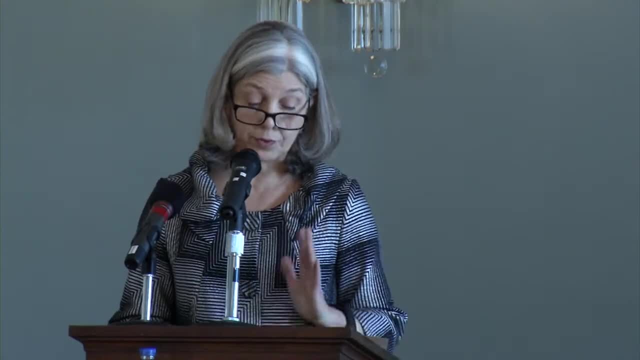 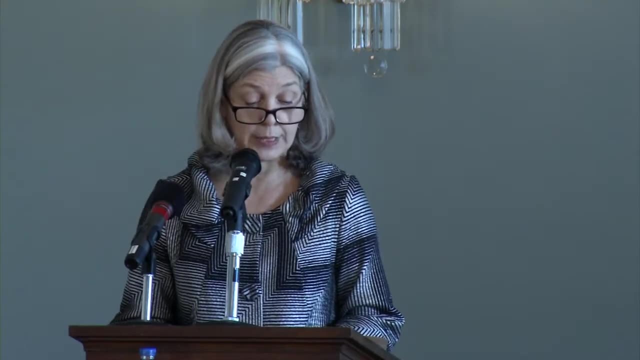 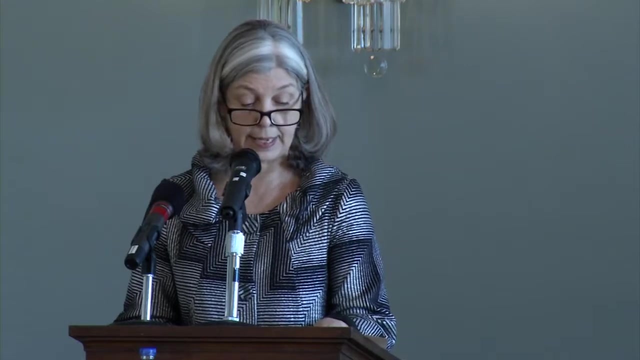 situation. the Gowanus Canal, where I live, he writes the Superfund site. there is still beauty and hope to be found. Plants carve a root hold in the canal's collapsing wooden walls, Jellyfish pulse beneath kaleidoscopic oil slicks and green algae blooms. 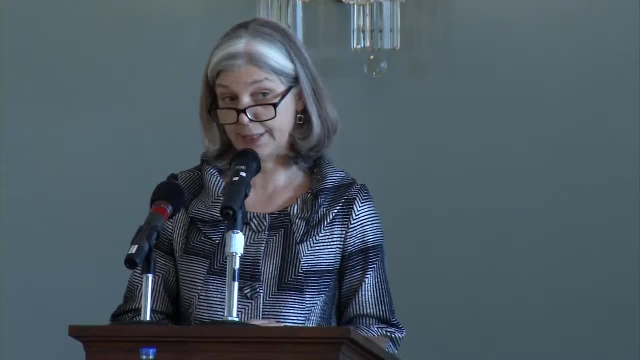 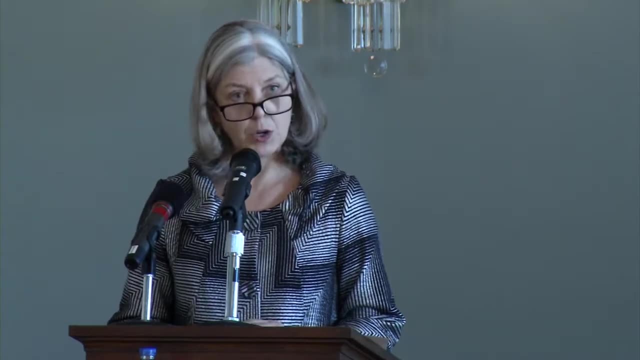 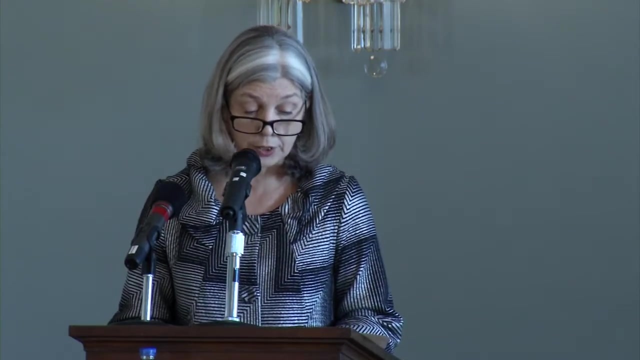 in the fecund waters. thanks to occasional pulses of sewage overflow, One day, oysters the size of dinner plates could return. He goes on gliding in a canoe through this toxic waterway, among the most polluted in the country, if not the world, affords a unique perspective on 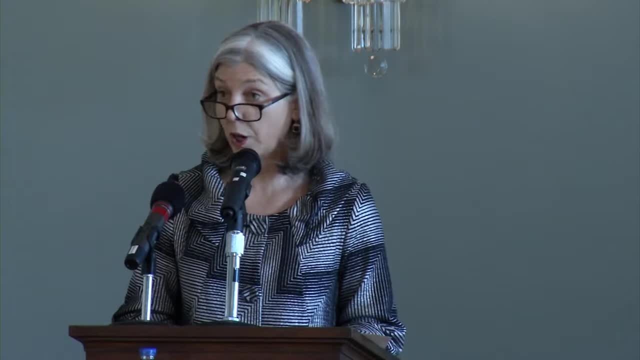 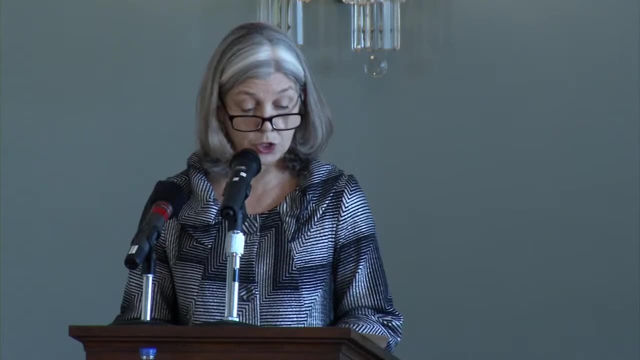 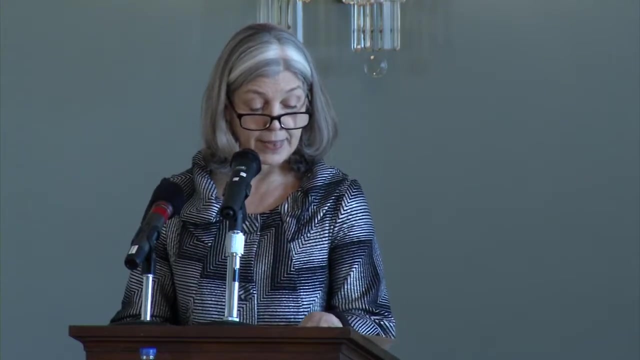 nature's resilience as well as humanity's. After all, the Gowanus would not have become a Superfund site, and therefore on the way to a cleaner future, if not for those of us who wanted to use it for something different than a flushing tunnel for waste. Things can get better. 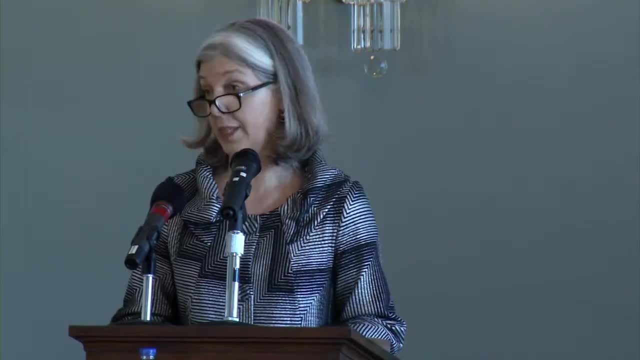 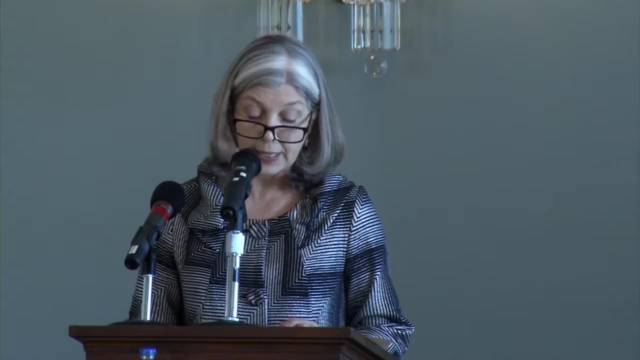 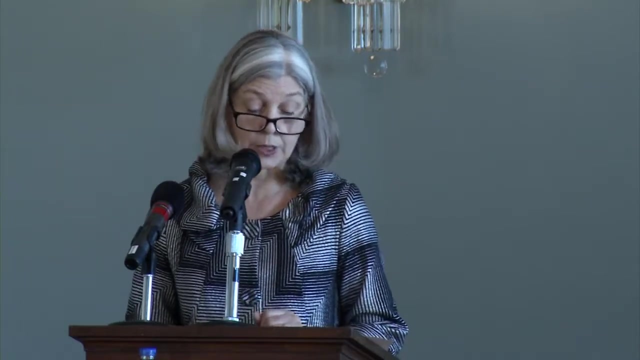 And there's a large portion of humanity working towards that these days- A global hive mind connected by the internet. In the end, science will give us clues and imagination that will light, but it is our own imagination that will light the way. And he concludes with: 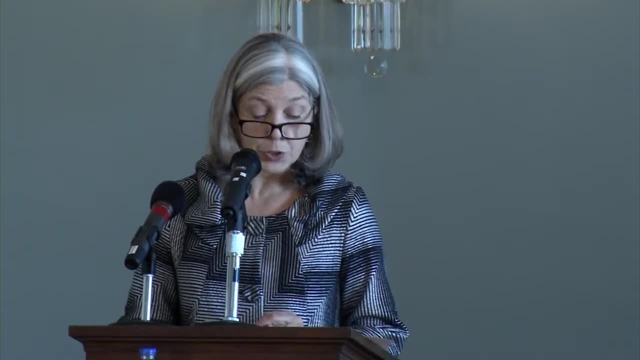 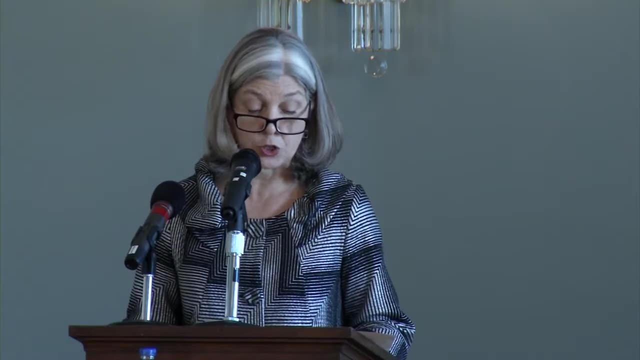 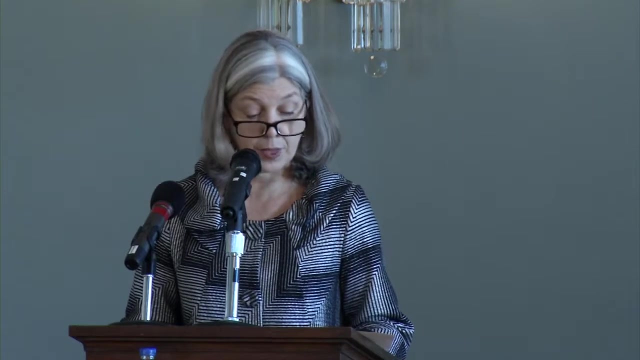 a challenge that I would pose to all of us. The most important literature we write in the Anthropocene will be the words that enable us to ensure breathable air, drinkable water, nutritious food and the persistence of the abundant life that makes it all. 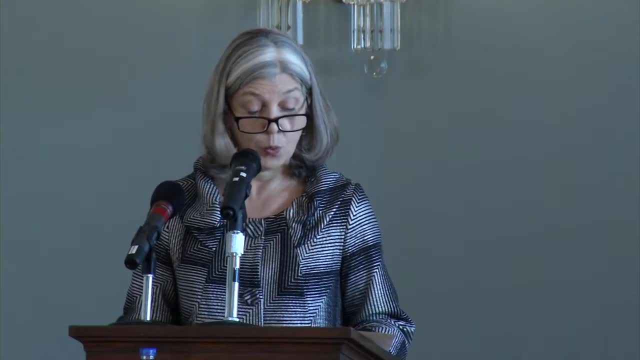 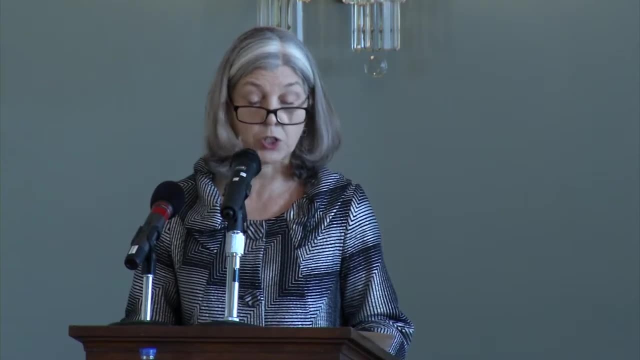 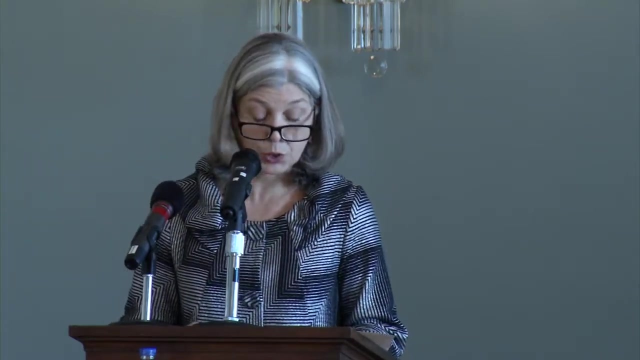 possible on this rocky mothership. We'll also need a robust history. to keep us honest, We need an enduring, resilient, hopeful literature for the Anthropocene. The organizers and my wonderful staff have spent the past two years debating, studying, fundraising, teaching and collaborating as they planned this conference. 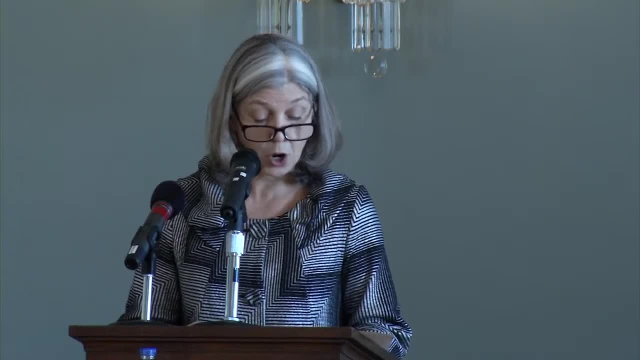 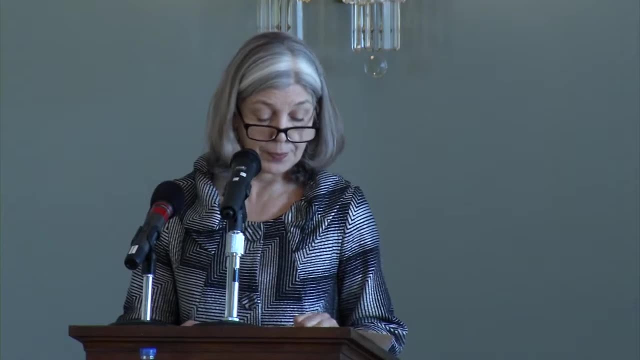 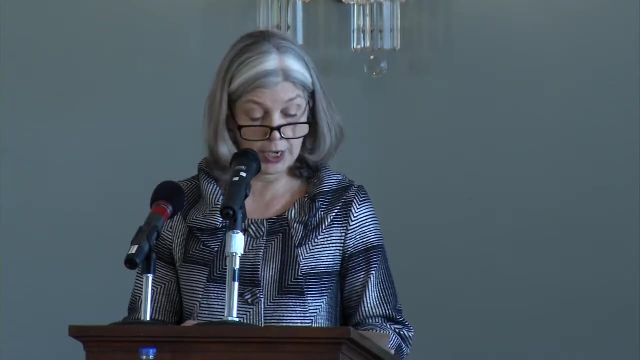 for us Now working together as artists, performers, activists and all the rest, scholars and scientists. it's our job to find those words and images and then to use them to inspire change. We're counting on our collective imagination to cast a bright light. 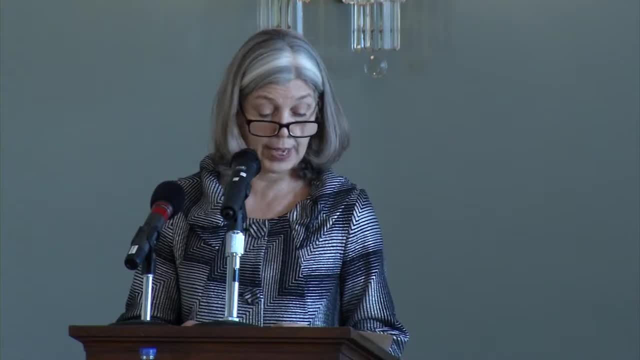 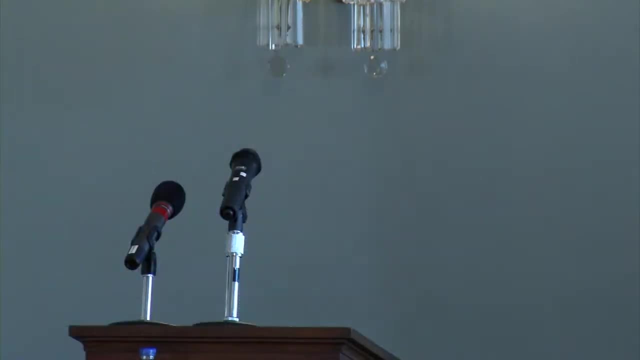 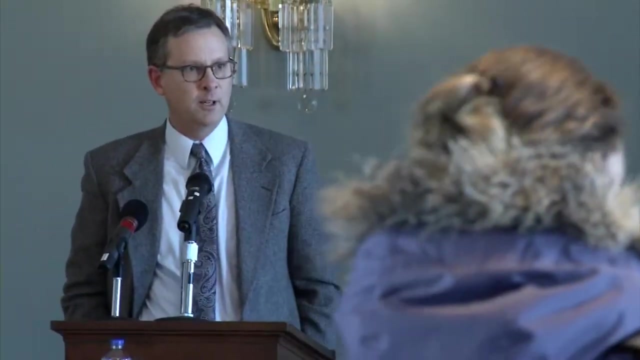 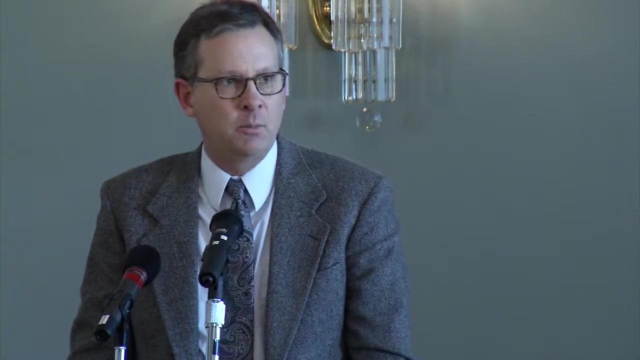 and our collective conversations over the next few days to take us farther along the way. Welcome to the Anthropocene. Good afternoon. Thank you for braving the cold to come here about global warming. We have a great program in store for you. I'm happy to see so many people show up and 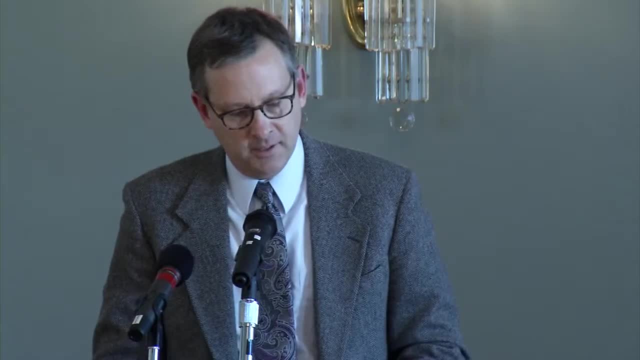 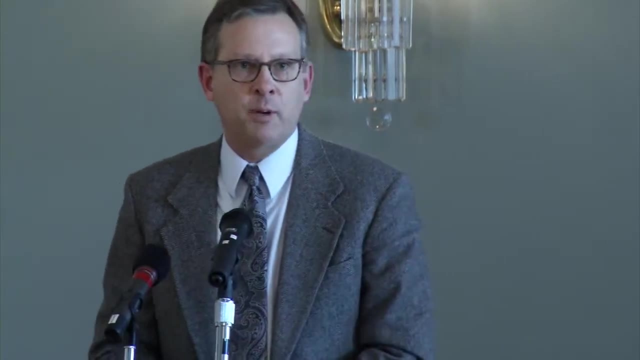 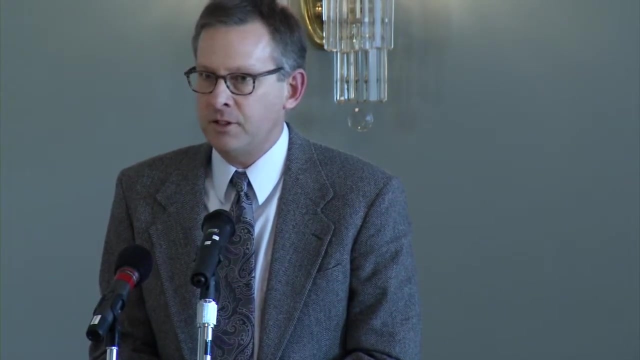 especially see so many of my students here. It's really nice to have this finally underway. Just another: Theresa mentioned some of the sponsors. I also want to pay a special thanks to Theresa and her staff at the Olbermann Center. She's a fabulous. 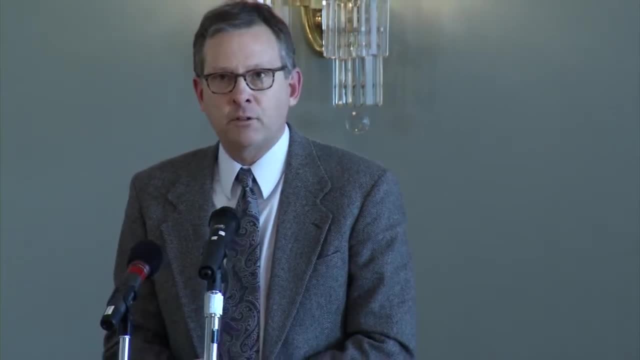 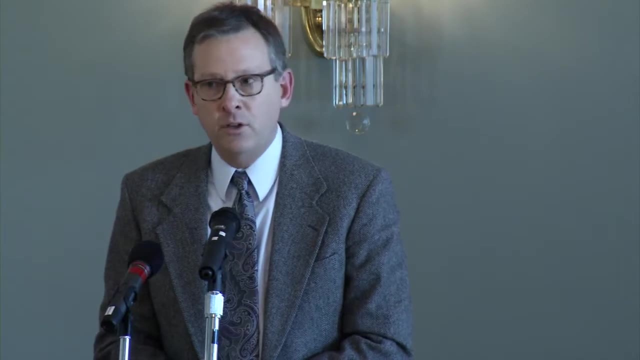 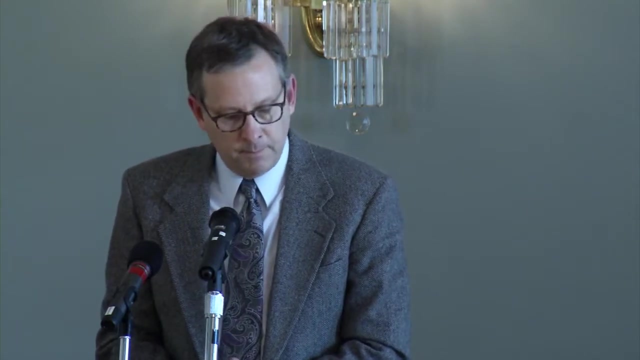 leader and gave us great counsel and direction in planning this conference. I also want to mention the assistant director of the Olbermann Center, Jennifer New, who was really one of the creative forces in planning this symposium. Erin Hackathorn, who 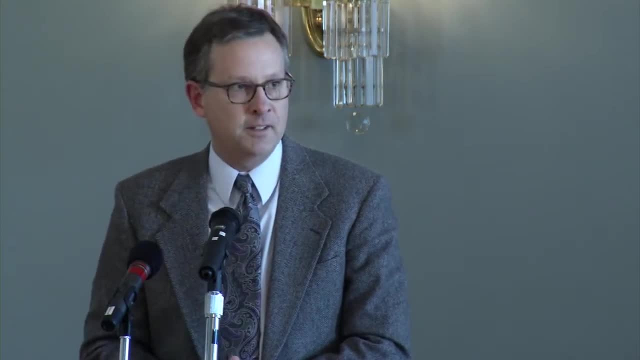 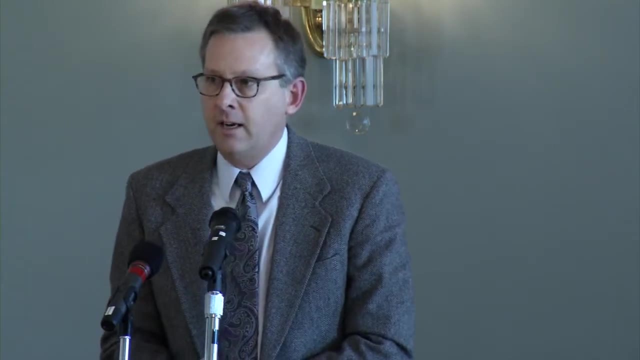 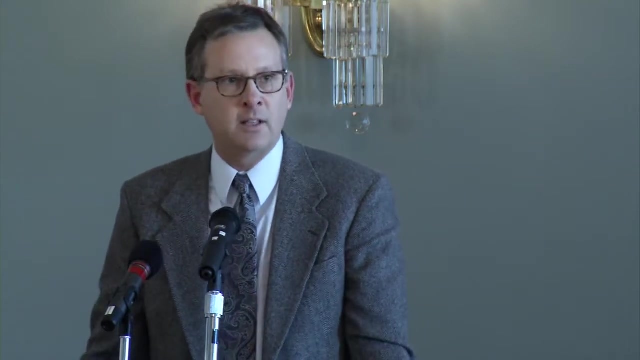 has been our field marshal and has handled all the financial and statistical details in really an exceptional way. And Miriam Janicek, who has created the digital presence, the great website. if you haven't taken a look at that, Look through the resources page and what we've created: the Twitter. 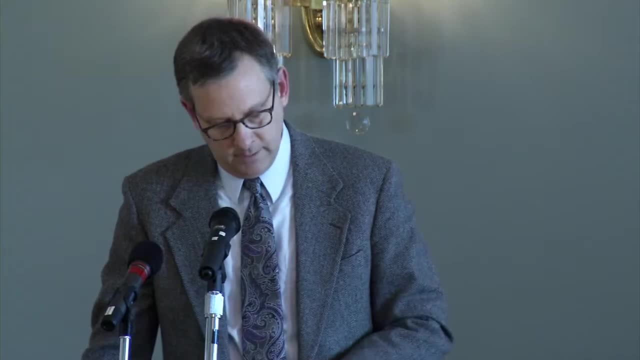 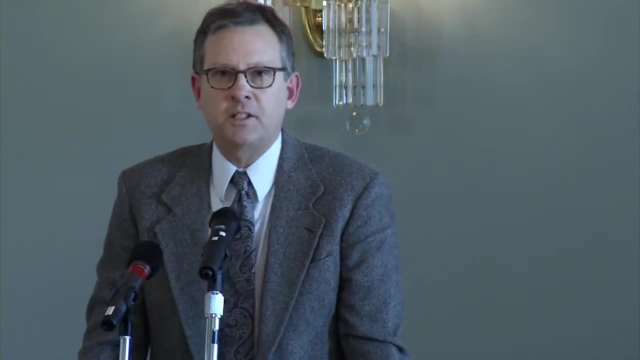 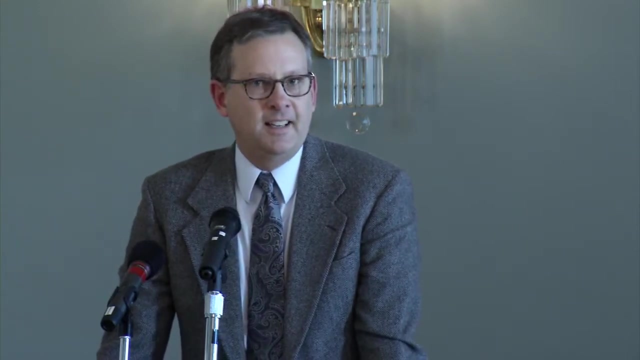 feed. It's really a nice resource that I hope will stay around for a while. I'm not going to talk about the Anthropocene so much, as I want to just say a few words, by introduction, about energy in Iowa. Many of our participants come from outside of Iowa. 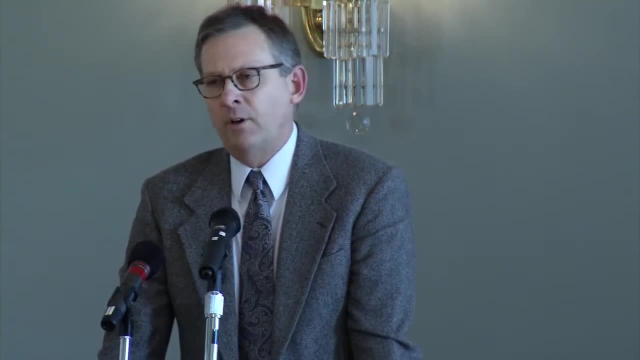 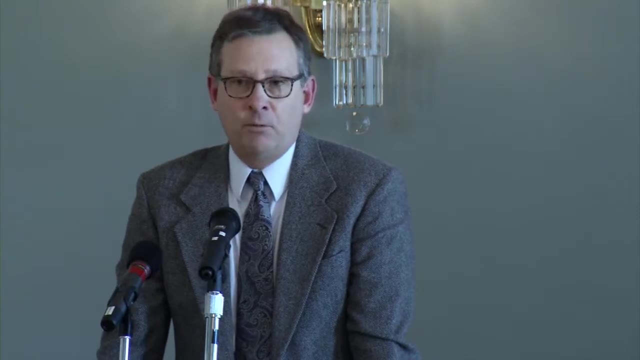 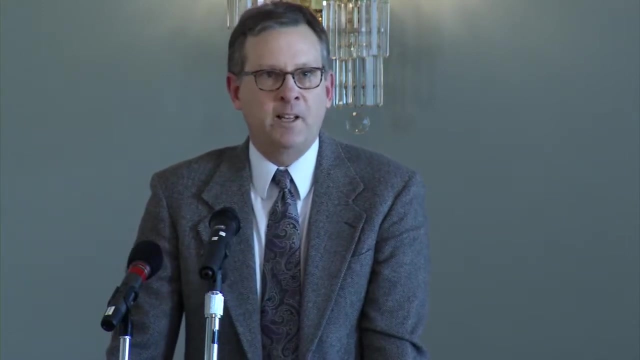 a long ways and may be wondering why we're talking about energy in Iowa, which is, for most people, is a farm state, not an energy state, but Iowa really is an energy state. I moved here a couple years ago from Houston, where you could find an energy symposium or an energy conference every day of the week. 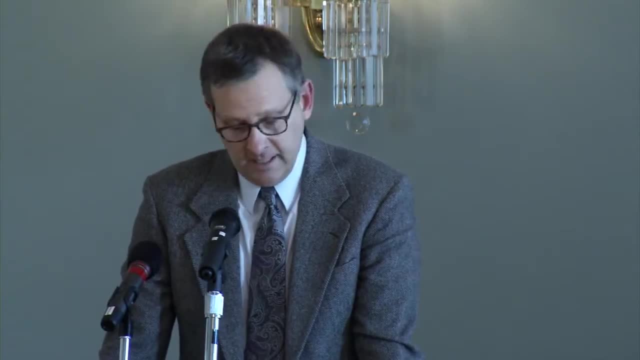 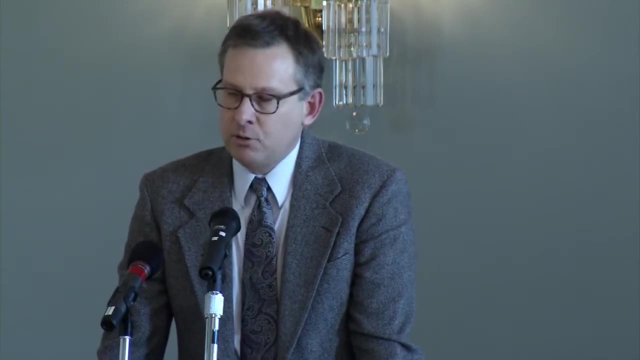 So it is a little unusual to be talking about energy in Iowa, but it probably won't be as we move forward. It is a corn and soybean state: 23 million- 36 million acres devoted to corn and soybean and, if you paid attention to, 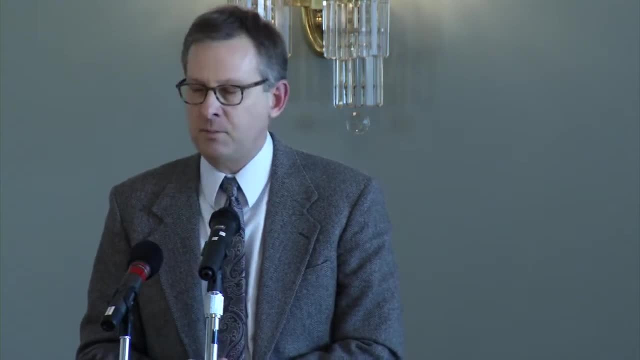 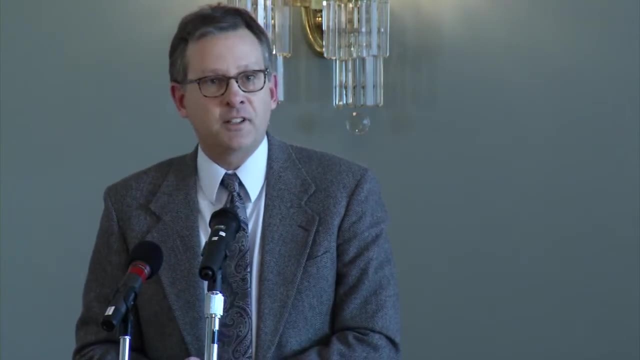 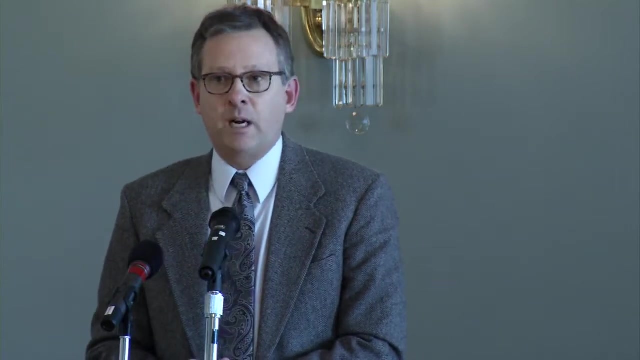 the Olbermann Factoid Fridays. you would know that this is more than all the land in the US national parks in the lower 48 states combined. But it takes a lot of energy to plant and fertilize and harvest and transport those crops and probably even more important, 47% of the corn crop in Iowa goes to the production of ethanol fuel. Iowa produces 30% of the nation's ethanol and somewhere close to 47,000 jobs are linked to the ethanol industry, regardless of what you think of it. 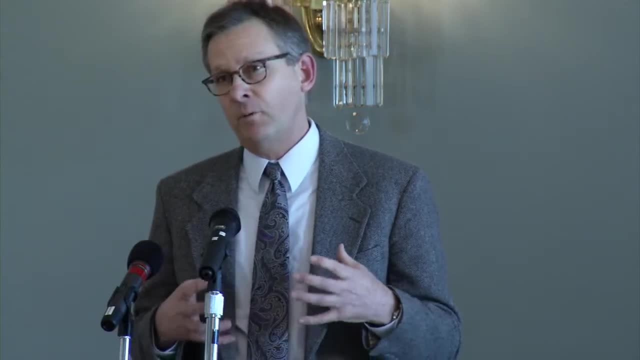 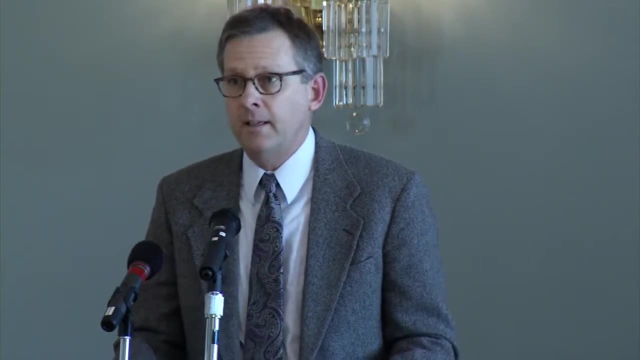 And so Iowa is an energy state, in a kind of contradictory way, Some people might. from some perspectives. It is also the third largest wind producer in the United States after Texas and California. More than 5,000 megawatts of. 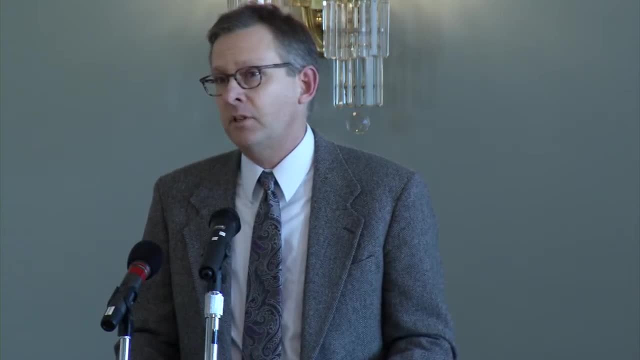 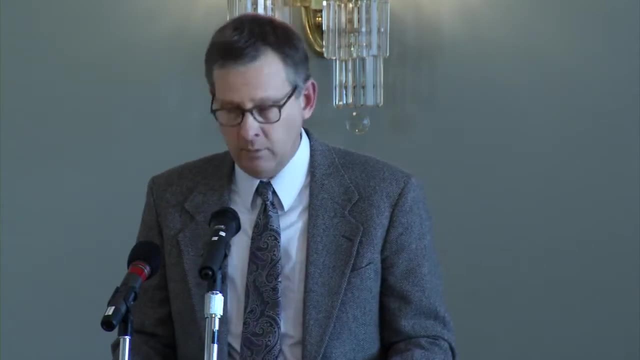 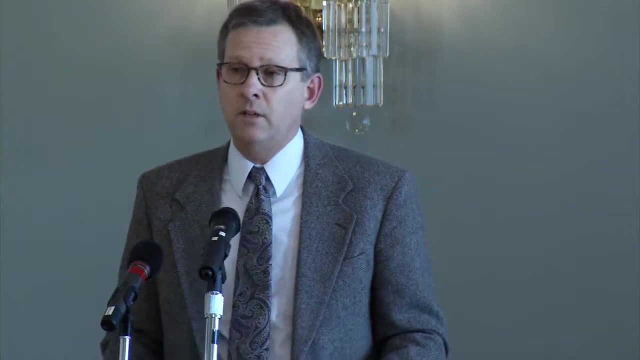 installed capacity: 3,200 utility scale turbines. 27% of the state's electricity generation comes from wind. Iowa was the first state to pass a renewable portfolio standard in 1983 that required utilities to purchase wind power, and there's something close to 8,000 jobs. 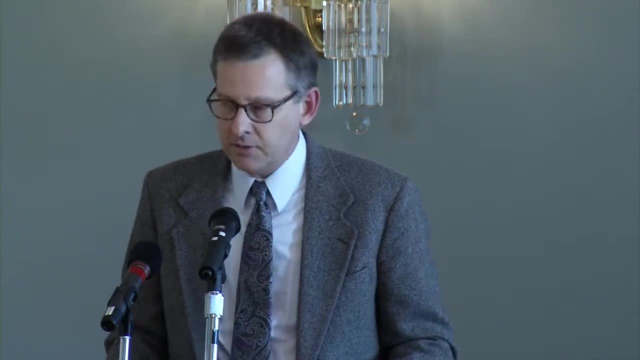 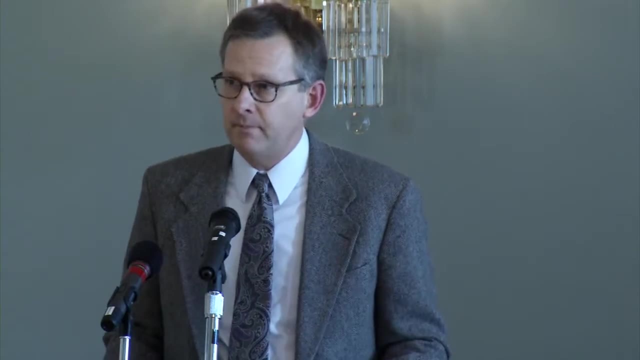 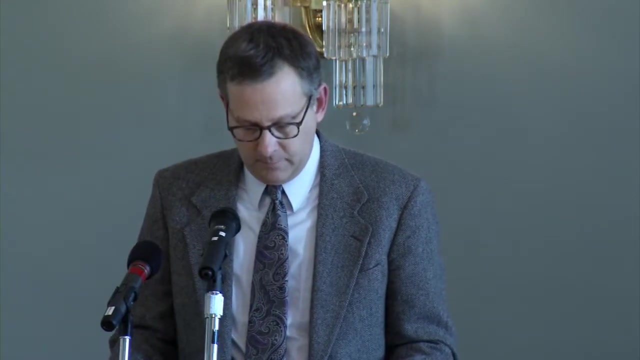 connected to the wind energy industry in the United States. Another way in which Iowa is linked to energy that may not be obvious but will become more obvious in the next several years is that North Dakota Bakken Crude rolls along the eastern and western 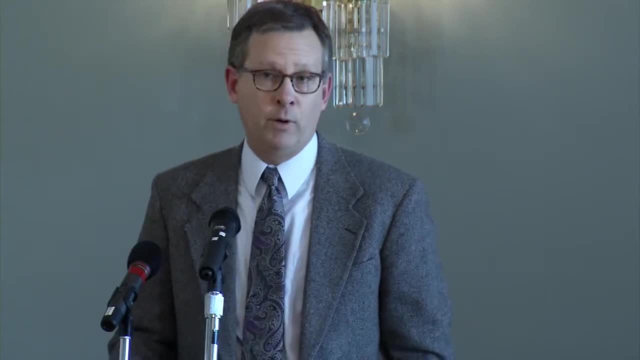 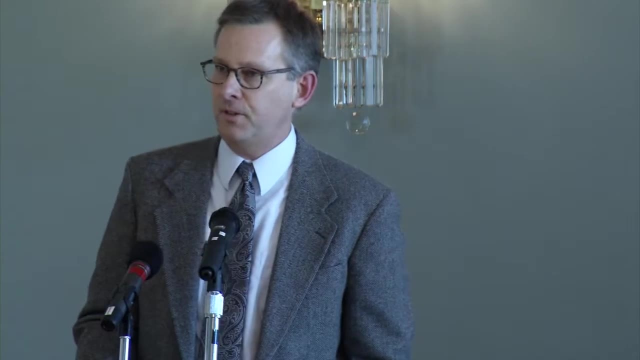 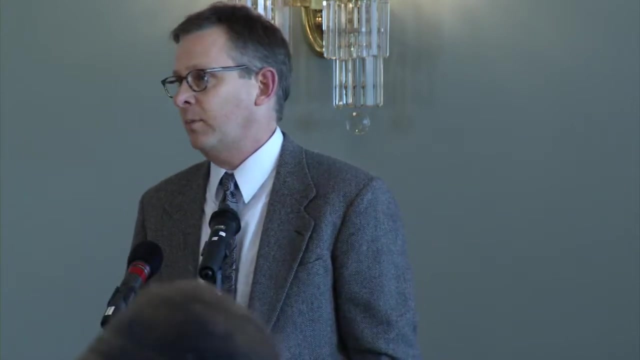 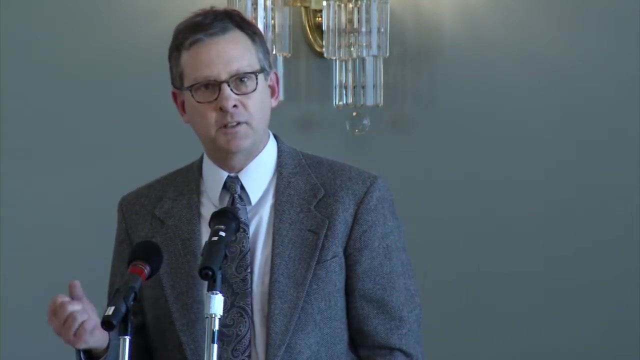 borders of the state by rail. Another way that Iowa is getting closer to the fracking industry. the hydraulic fracking industry is just across the border in Wisconsin and Minnesota we have large scale sand mines. that mine, the St Peter sandstone, which is a uniform, and 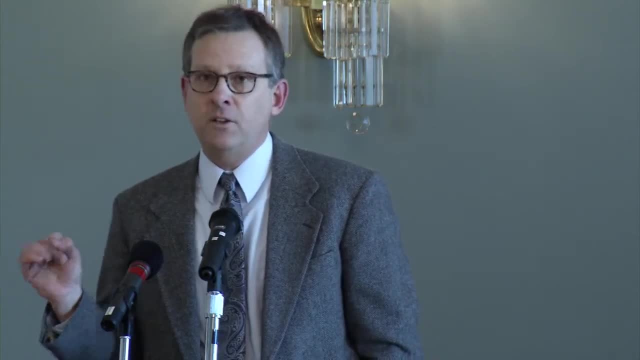 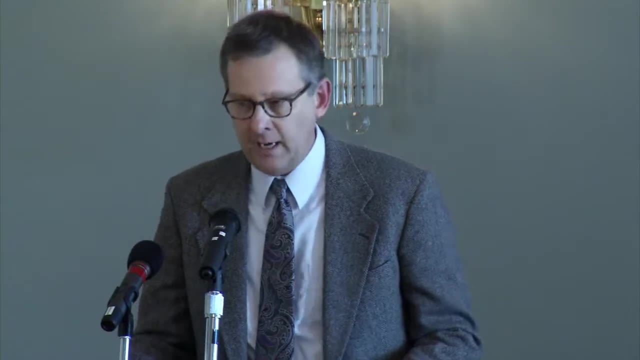 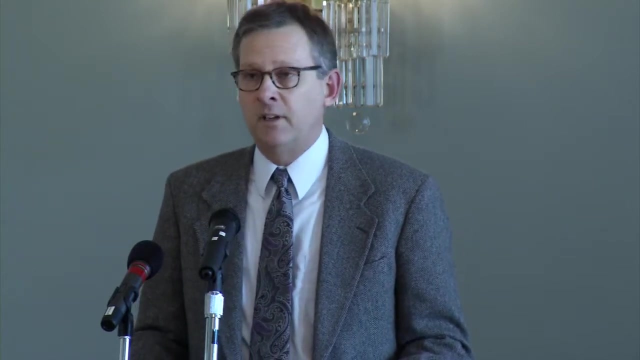 perfectly round form of sand that they use in hydraulic fracturing in Pennsylvania, and especially in the Bakken, And it's threatening to spill over into some of the northeast counties of Iowa, So fracking- even though we don't actually frack for oil and gas in Iowa- we are very closely connected to it. 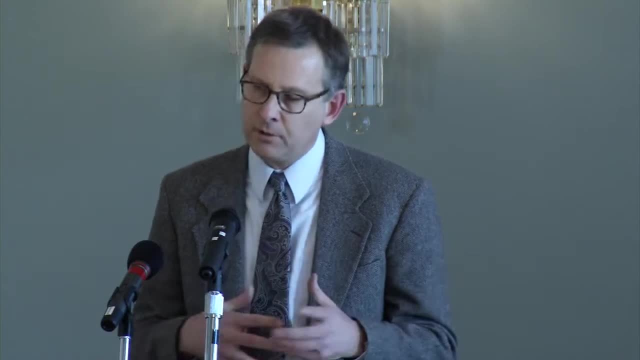 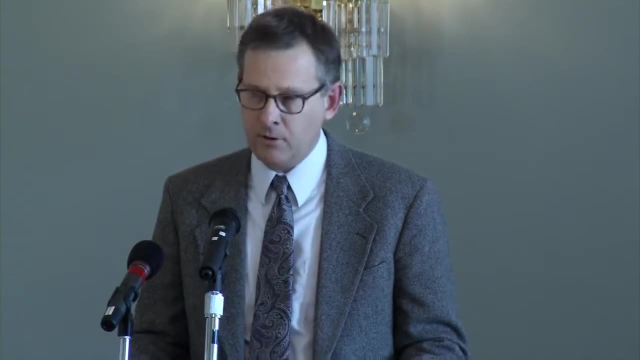 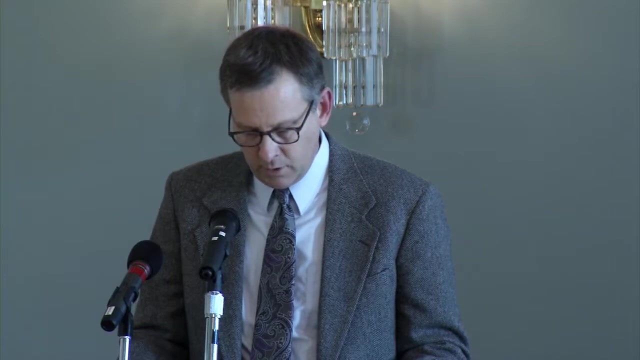 Iowa has long been a crossroads for migration and transportation, and it is becoming a crossroads for energy too. There are two controversial transportation proposals that are before the state at the moment. One is a corridor running diagonally from the northwest corner of the state to the southeast corner of the state, under study for the. 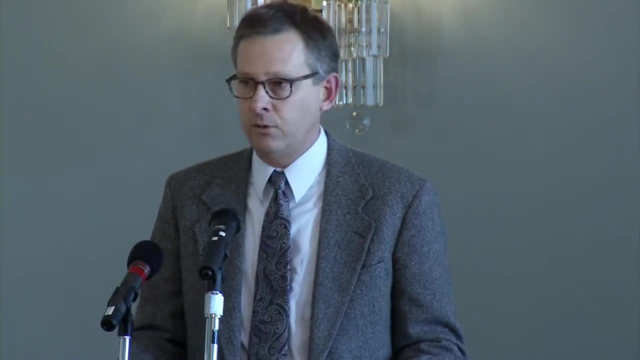 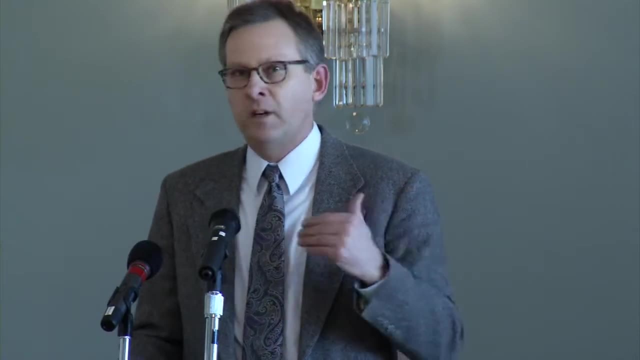 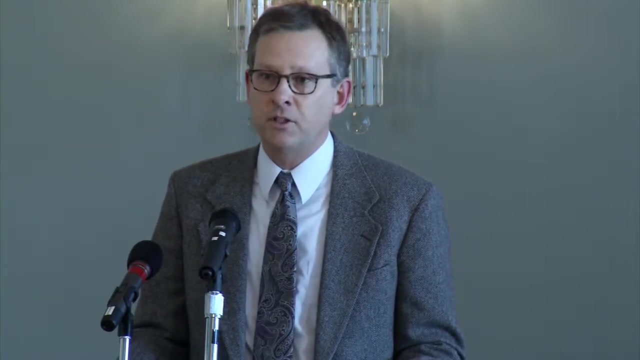 construction of a pipeline To carry Bakken crude oil to Patoka, Illinois, And along a sort of similar corridor, but a deviating corridor from the Bakken line, is a proposal for a 500 mile high voltage direct current transmission line that would bring wind power from the. 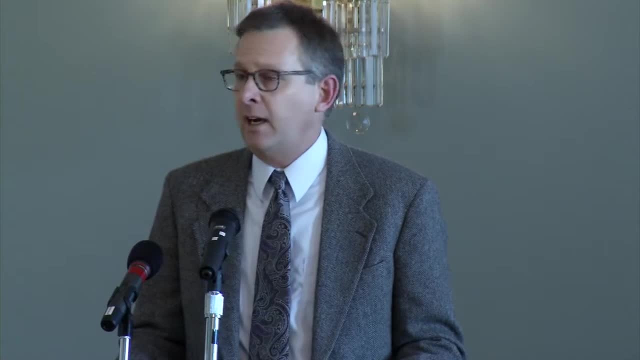 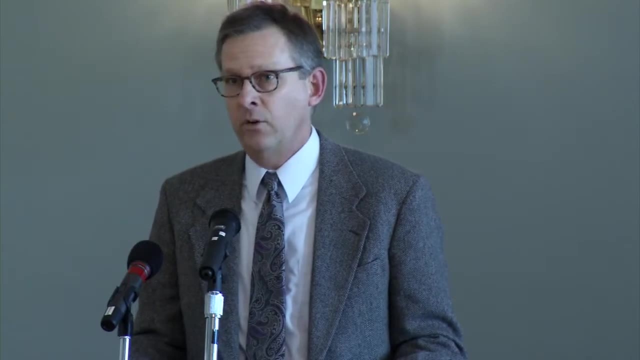 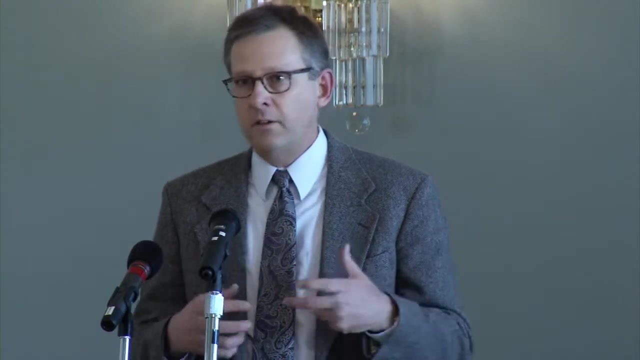 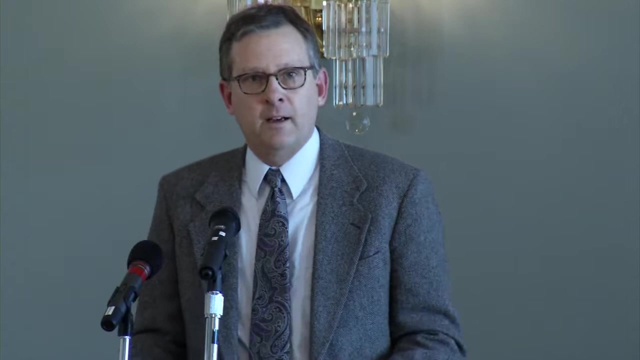 Buffalo Ridge region of Iowa and South Dakota and Nebraska to Illinois to plug into the grid in Illinois and deliver cleaner energy. It's called the Rock Island Clean Line. So wind, hydro-fractured crude ethanol and then also solar. Just last year the Iowa Supreme Court. 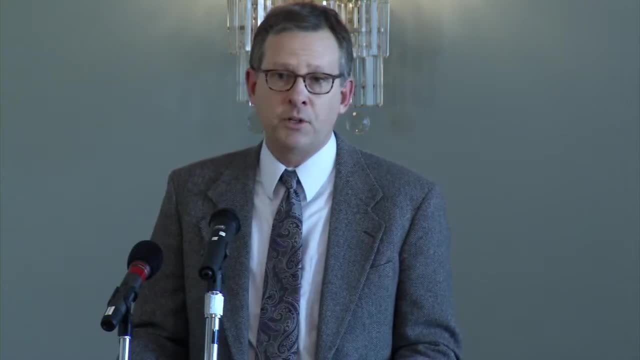 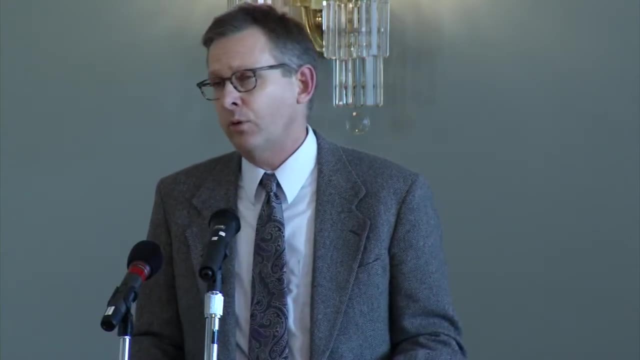 ruled in favor of third party power purchasing agreements, which is going to provide a boon to, and it's called the Eagle Point Solar Case. if you're interested in learning more, It's a pleasure to have an opportunity to come and speak to you today. I want to thank the organizing committee for inviting me. It's my first time to Iowa City And I've enjoyed my interactions with faculty and students, And so I want to talk about climate change and the evidence that we have found from the glaciers. And I want to start out with some graphs, because that's what scientists do. But I'm going to change. I hope to serve as a transition into other disciplines, because I do not believe. I've been studying climate for 30 years and producing records. and if you look at the trends that we're on, we're still on those trends, And so how do we bring about change? And that really is going to take all of us working together. First, I want to say that this is not. a one-person activity. It takes a team. Anything that you do takes a team, And we have a great team at Ohio State. We've had students and post-docs take support from various organizations to make these things happen, And we've now drilled in 16 countries around the world. That could not be. done without the collaboration of people in countries around the world to make that happen. So it's really a team effort, But I think the problem is an extremely important one. So, first of all, the Earth's climate is changing And the world is getting warmer. Even though you might not think that here in Iowa today, But there's no debate about this. This is a scientific consensus around the world. And I want to talk about glaciers as recorders of climate change, And this is when we drill in them. We get an ice core. We can look at how climate has changed through time. And then glaciers also are indicators of climate change. They respond: when it gets warmer They retreat. when it gets colder They advance. So they are also an indicator of how things are changing. And I will show some evidence that in some places these glaciers are smaller than they've been in over 6,000 years. But then I want to go on to the human side of climate change, And about eight years ago I determined that we need a better understanding. scientists need a better understanding of people And why we do anything, And I had an invitation to speak to Behavior Analyst 5000, an international conference Why we do what we do as humans, And I thought this would be an opportunity. But when I was preparing for that talk, BF Skinner was one of the founding fathers of that discipline And he was very optimistic when he was young And middle-aged, But by the time he became 80, he was very concerned about whether we as a species can act in our own best interest, And there were two things he was. concerned about. that relates to climate, And one of our characteristics is that immediate consequences outweigh delayed consequences. When we talk about climate change, we often talk about what's going to happen 20 years, 50 years or in our children's lifetime, And so we, as a species, do not react. we're here now type of people, And then consequences for the individual outweigh consequences for others. We might be concerned about people being displaced in Bangladesh, but we'll be more concerned if we are displaced. And that's just some of the basic. 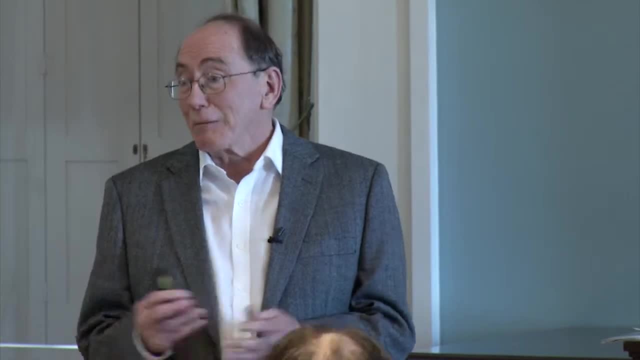 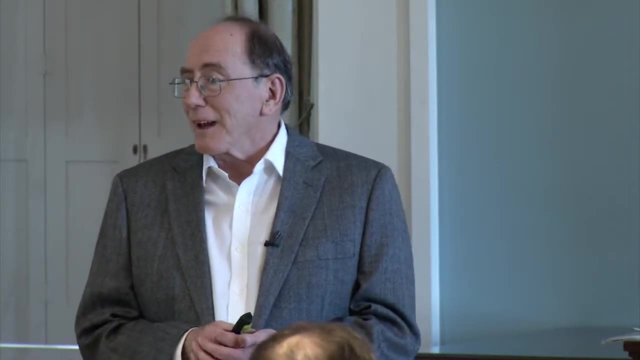 of our characteristics. Then I want to talk a little bit about our options and what I see as the greatest challenges in the 21st century. And then at the end, kind of as a save way to tomorrow's lectures, there's a new documentary produced. 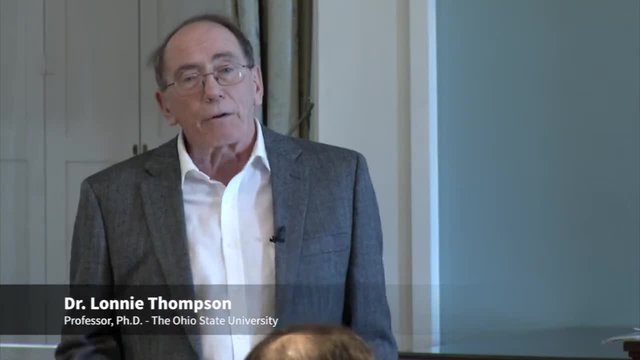 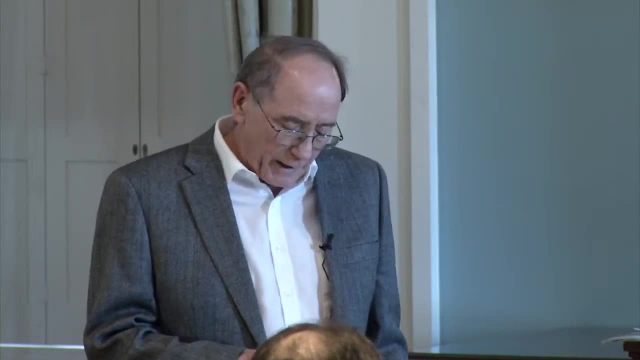 by Ethan Steinman And it's called Glacier Balance, But what he did was to go down the axis of the Andes in South America looking at what's happening to the glaciers and interviewing people that you would probably never hear from that live in these remote parts. 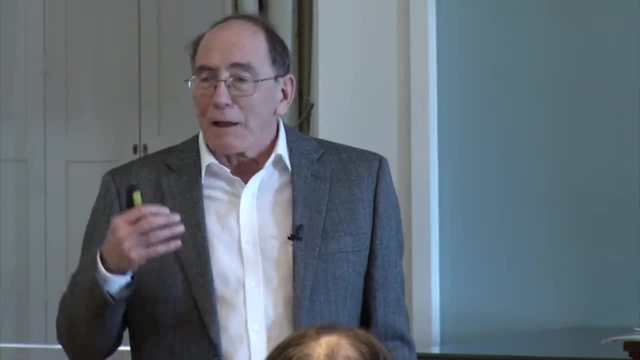 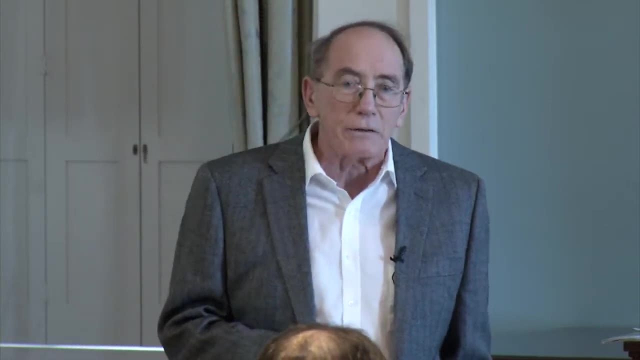 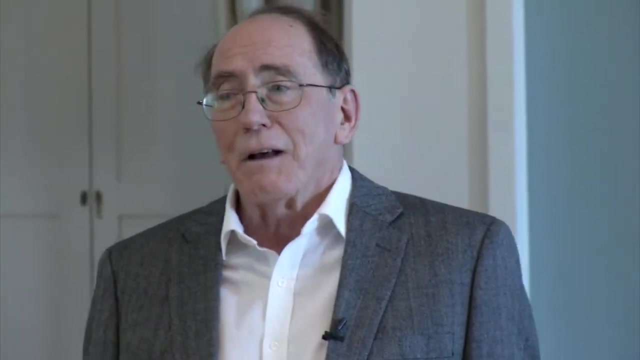 of the world And we're all part of this human species on the planet, And so you get a different perspective from that. He also went up and filmed our last drilling project in that part of the world, So there's a real difference between weather and climate. 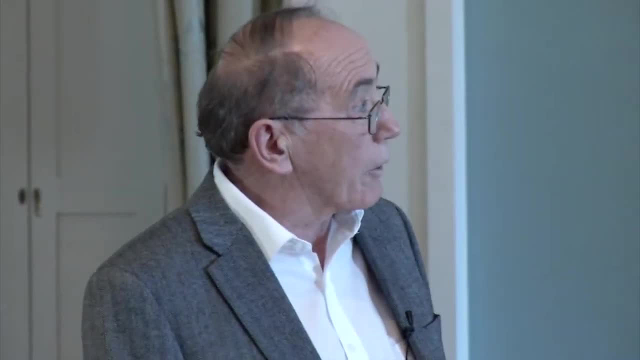 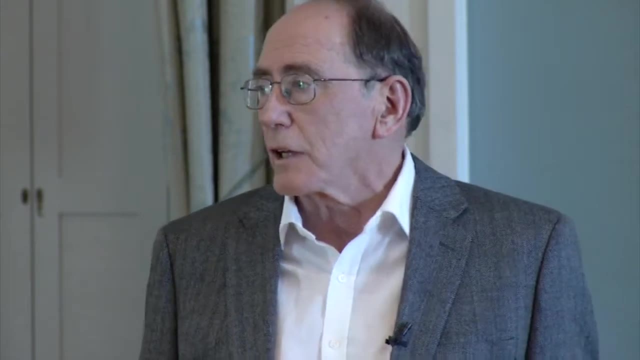 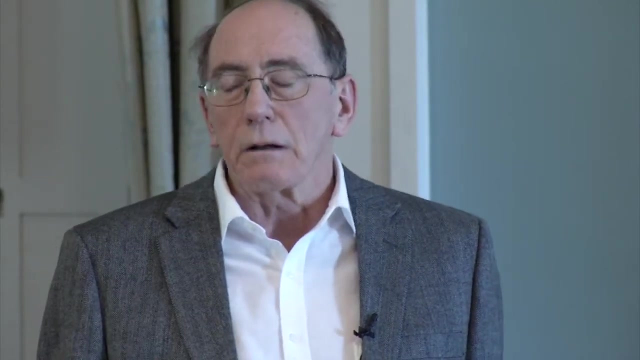 And I want to talk a little bit about that. Global climate change involves many changes. It's not just temperature. We're looking at things like changes in precipitation, sea level, glaciers, sea ice, ecosystems. There are so many parts of our system that are impacted by these. 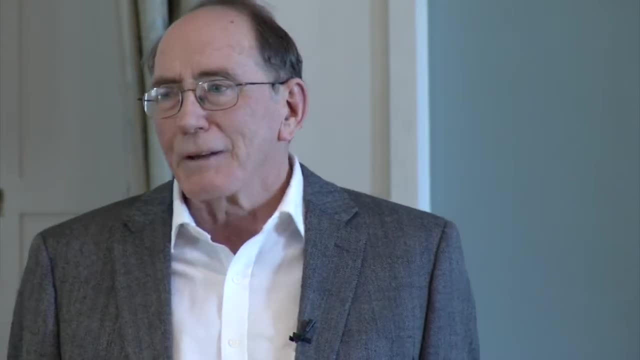 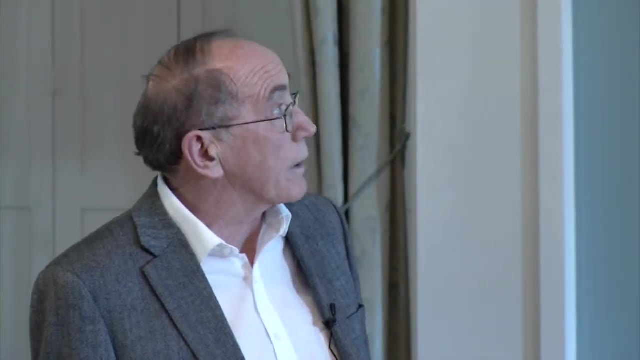 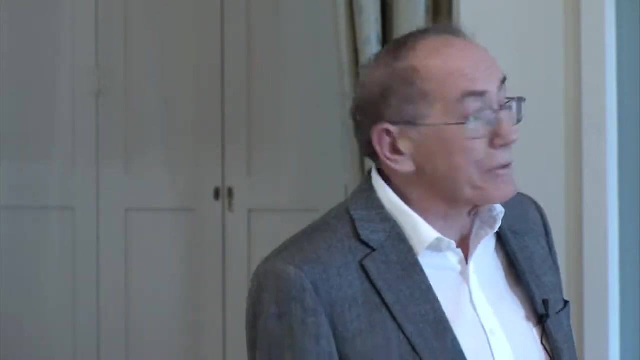 changes. There have been three major scientific assessments in the last year, in 2014,, that concur that carbon dioxide and other greenhouse gases, as well as aerosols into the Earth's atmosphere, are the dominant cause of the warming that we've seen since the 1950s on this planet. 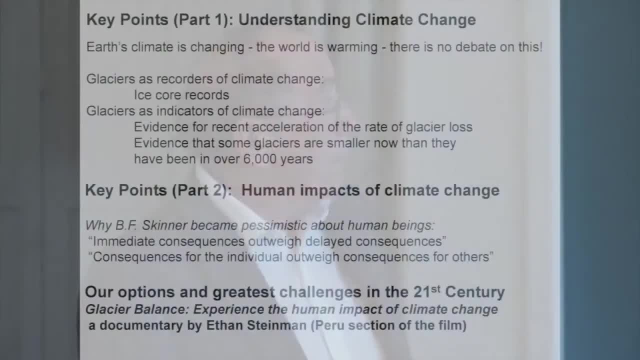 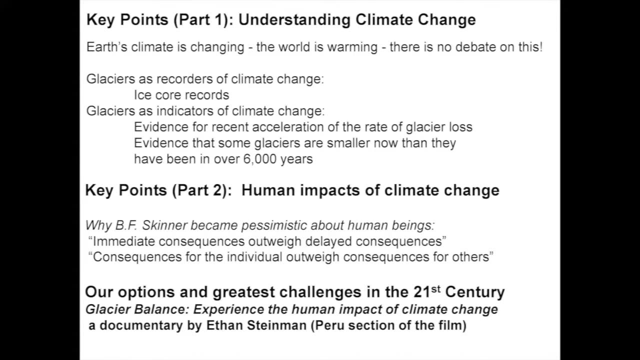 Rise in greenhouse gases And we need to address how we will power the human enterprise in the coming decades and centuries because of that. So if we look at the temperatures, how they're changing, these are our instrumental records And we can see that temperatures have risen. 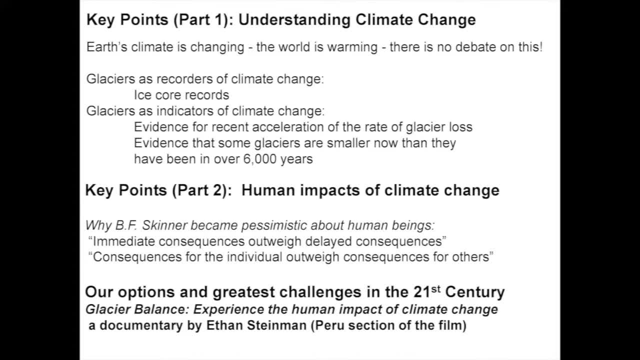 about .95 degrees C, or 1.7 degrees Fahrenheit, for the period for which we have been measuring temperatures on the planet, And our warmest years on record have been 2005,, 2010, and 2014.. And probably the more telling of this is that, if you look at 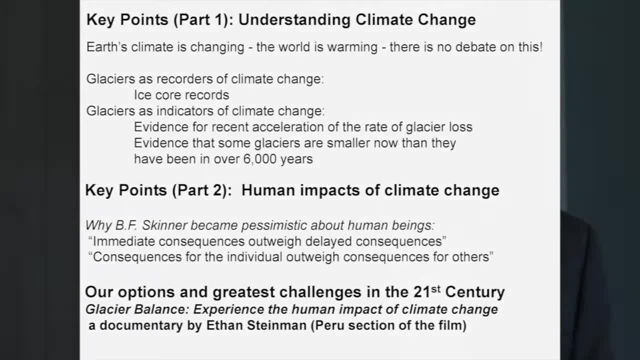 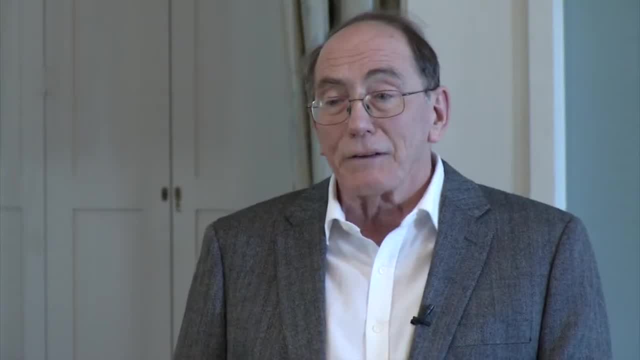 the 15 warmest years on record, 14 have occurred since the year 2000.. So the planet is definitely getting warmer And we can look at where that warming is occurring and you can see that it's centered up here in the high. 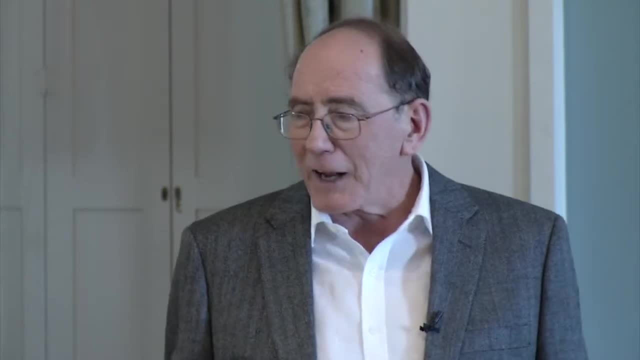 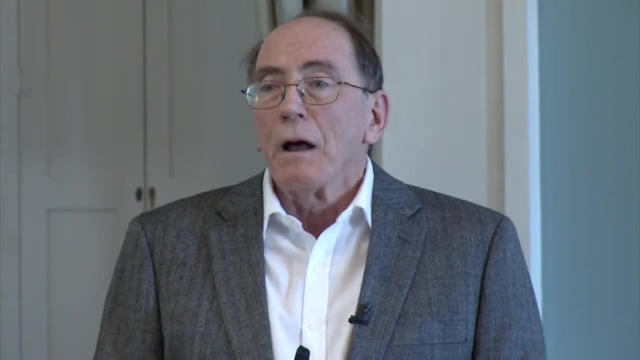 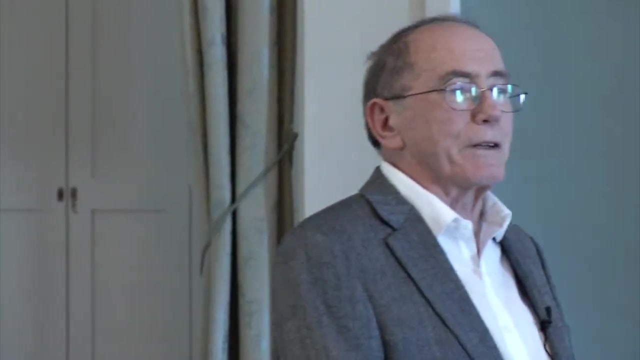 altitudes in the Arctic, And there are reasons for the feedbacks in that region. The climate of the last 30 years has been remarkable. There has been an increase in frequency and intensity of extreme weather events, And there are examples of these, and I'm going to show some of those. 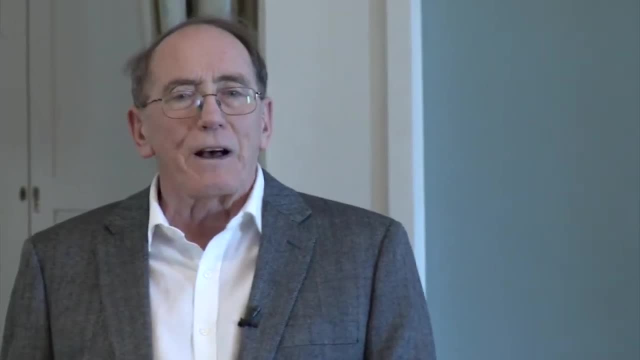 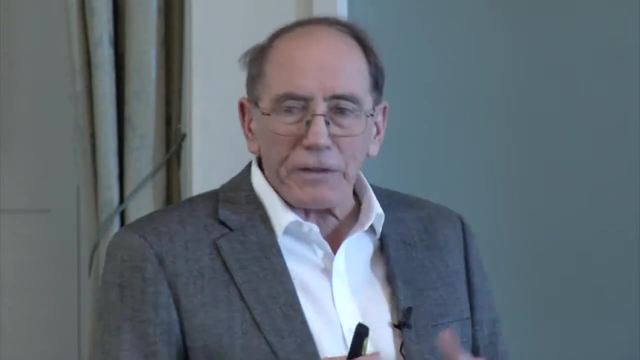 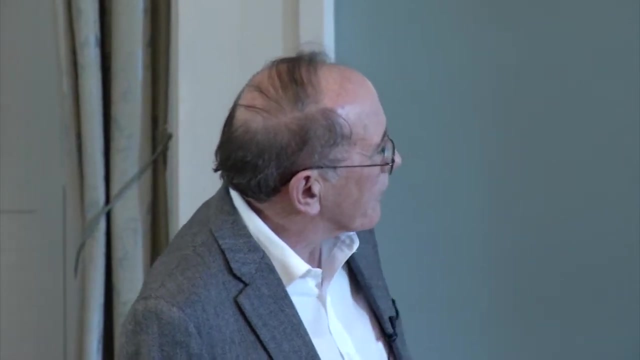 The amounts of droughts and fires that occur on a global scale And the Intergovernmental Panel on Climate Change models predict these types of system responses to global climate change will become more frequent as we go forward in time. If you look at the decade to decade, 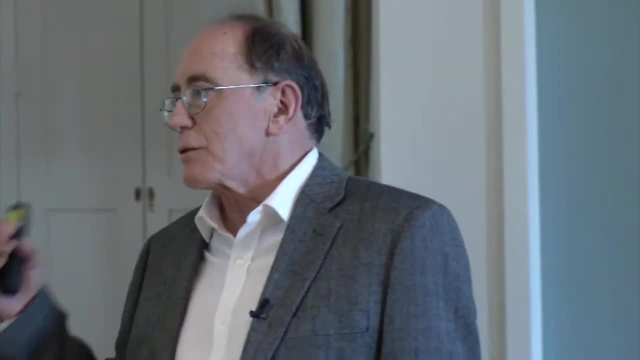 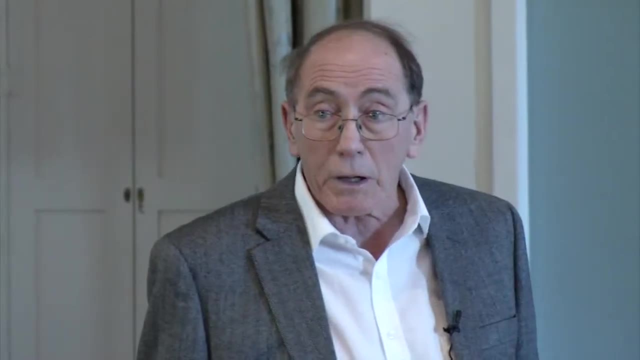 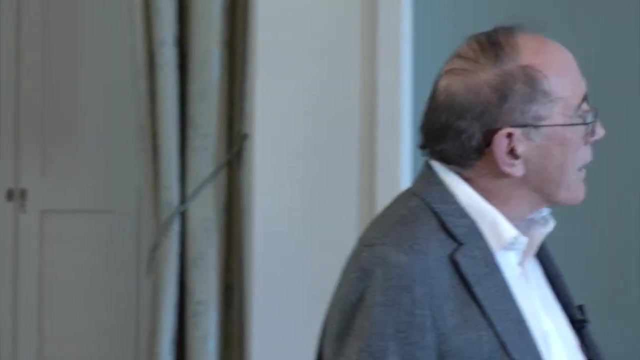 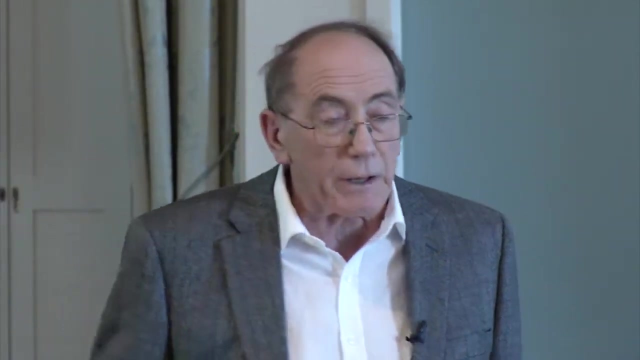 changes in temperatures starting from 1961 to 1970 and coming up to 2001 to 2010,. you can see how these are concentrated in the higher latitudes and on the continental areas of the planet, And particularly this Arctic amplification that is occurring as you melt back as the sea ice. 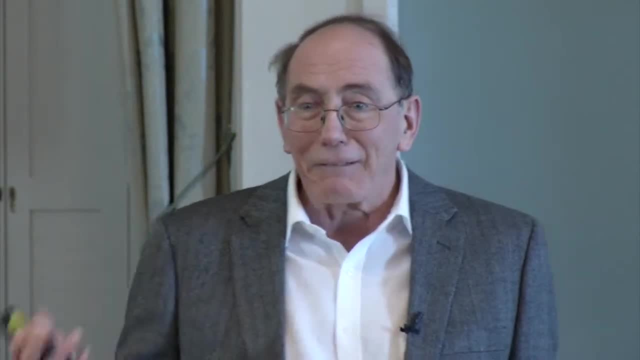 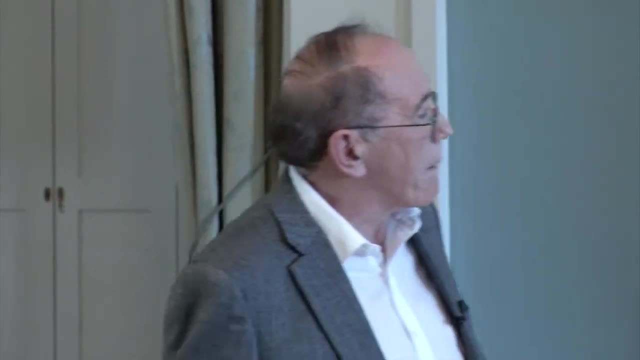 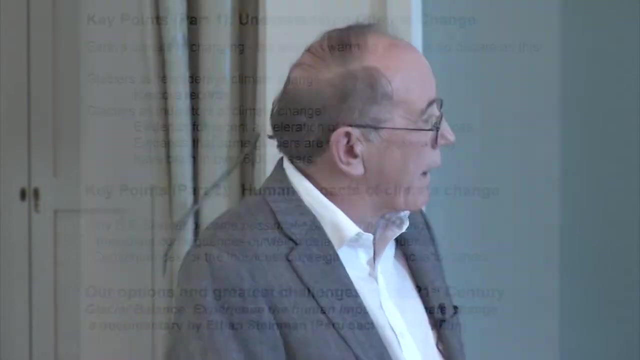 reduce the size of the glaciers. you're exposing darker surfaces that absorb more radiation- natural radiation coming in, And this tends to accelerate this process. This is our record of what's happening to sea ice up in the Arctic. This is a closed basin And 2012 we had 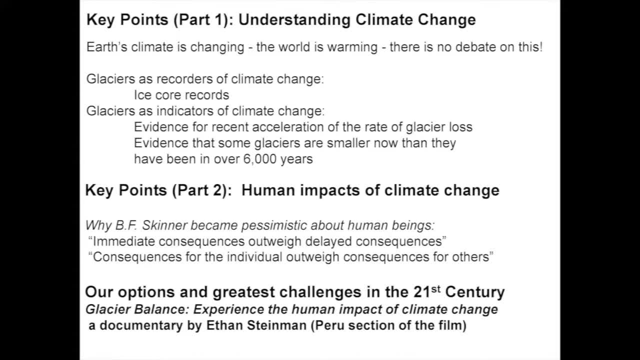 the minimum amount of sea ice, and it was 19% below the previous minimum, which was in 2007.. And when you look at these records, what you're going to see is the timing of when these things are occurring, And this is. it doesn't really matter which record you're looking. 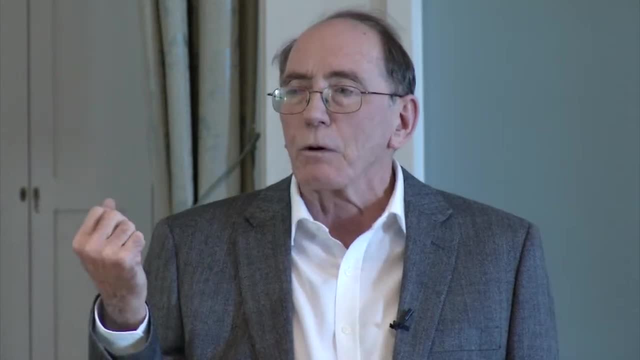 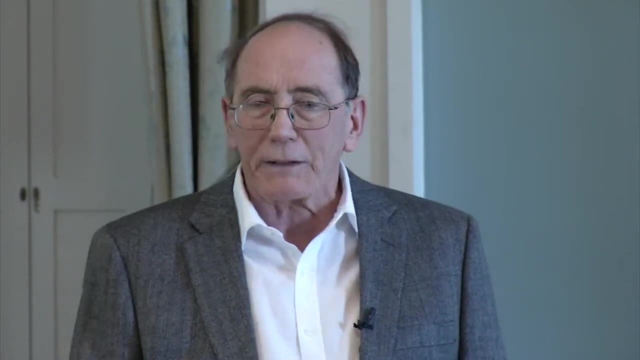 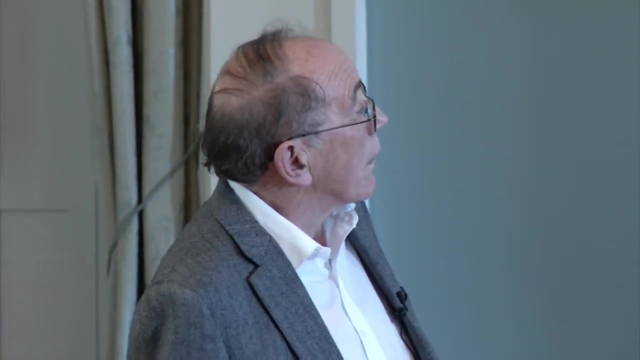 at, You see the same trends that are taking place. So amongst the changes these are northern hemisphere spring snow cover, And this has been decreasing, as you can see here. That's also another indicator of warming. If you look at the change in the global, 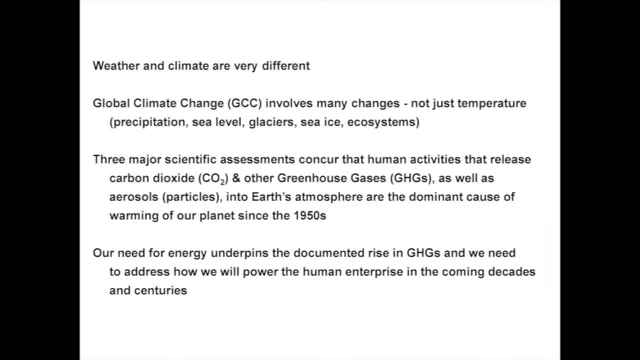 average upper ocean heat content. you can see how that is rising over this same period of time. However, as human beings, we respond to what's happening in our own backyard, And I want to use this as an example. This is: I'm from Ohio. 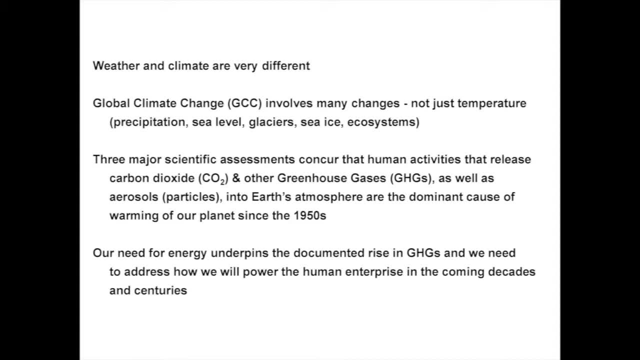 so last year was a very cold year in Ohio and in eastern US, And particularly in January. So if you look at the temperature distributions on the planet in January, you can see that, yes, in our part of the world it was extremely cold, But they were setting. record temperatures up in Alaska, over in southern Greenland and over in the Beijing area in China. And when you look at these temperatures of the planet, you have to look at the global average, And so January 2014 actually was Earth's fourth warmest January since we've been keeping. 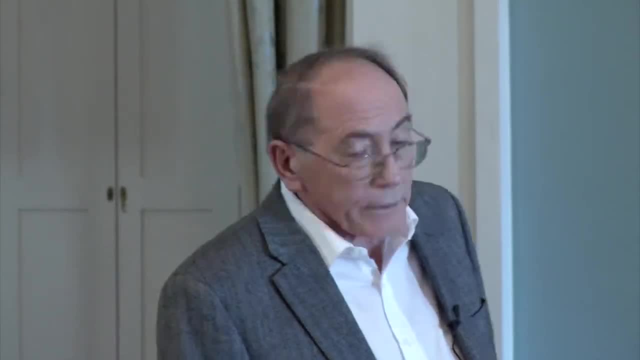 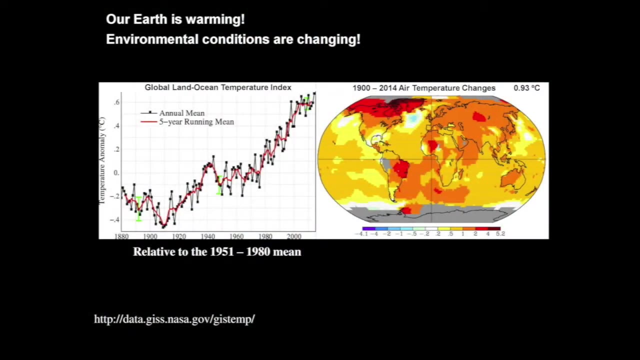 instrumental records, Even though you would never be able to prove it in this part of the world. I like this diagram to show the difference between weather and climate. In this diagram, the man walking the dog is the climate, And if you ever watch the one walking the dog, they go in a straight line. 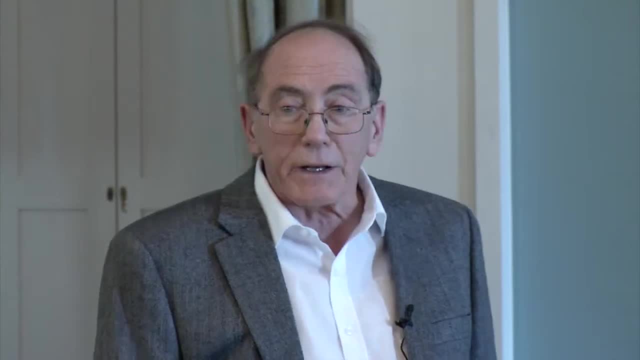 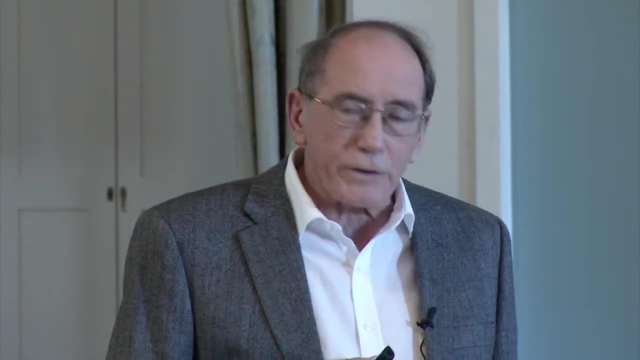 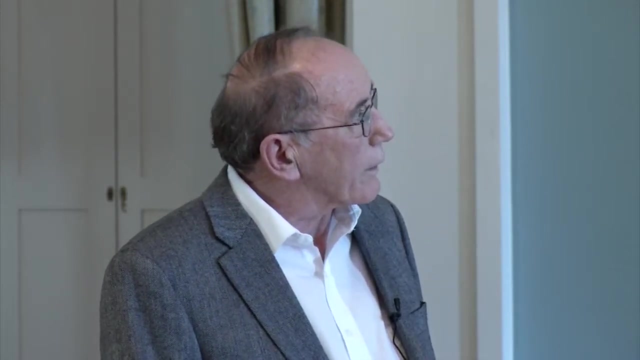 However, the dog is going from fire hydrant to a piece of paper, going back and forth. Well, the dog is actually the weather, And I think probably Mark Twain said it best when he said: climate is what you expect, weather is what you get. And I want to use Iowa City as an example. Last January in Iowa, the 30 year average, we would have expected the city temperature average of 23.6 degrees Fahrenheit Or minus 4.7 degrees C. But what you got? 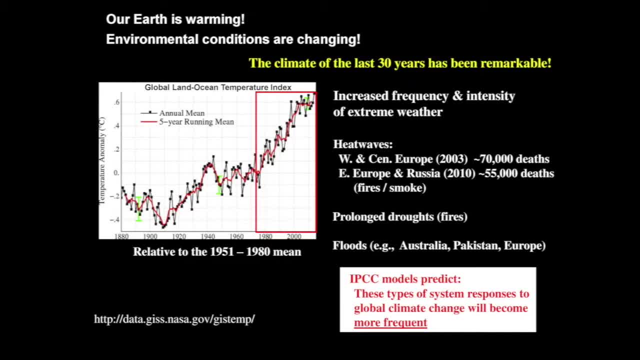 was weather which was 13.1 degrees Fahrenheit and minus 10.5 degrees C. So there's a big difference in taking averages over 30 years and looking at this season to season variability. There's been natural mechanisms changing the climate on this planet through 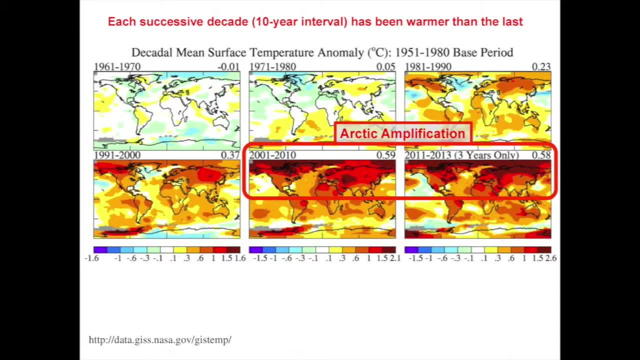 time, and these are a few of them here: Changes in the output of the sun. We have an 11 year solar cycle, We have a 90 year Gleisberg cycle, And the energy from the sun is what drives the climate on this. planet. We have changes in the amount of volcanic aerosols in the atmosphere. Every time we have a major eruption that puts tephra and sulfates in the stratosphere. the temperature at the surface of the planet actually cools for one or two years until that material falls out. 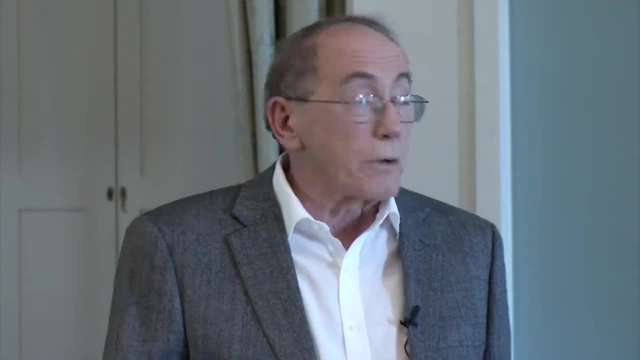 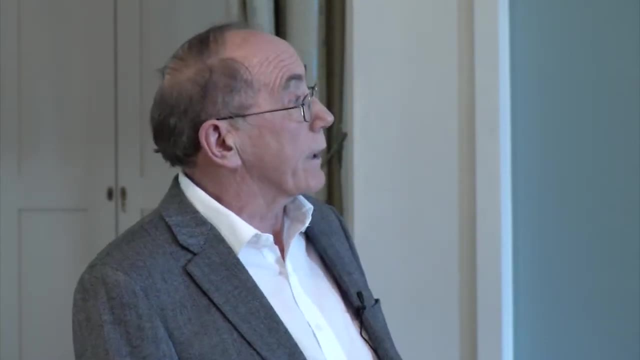 We have internal variability, We have monsoons, We have ENSOs, And these have been with us for thousands of years and they affect the climate. Now, on top of that, we have the human factors, And these are non-natural mechanisms. These are changes in the 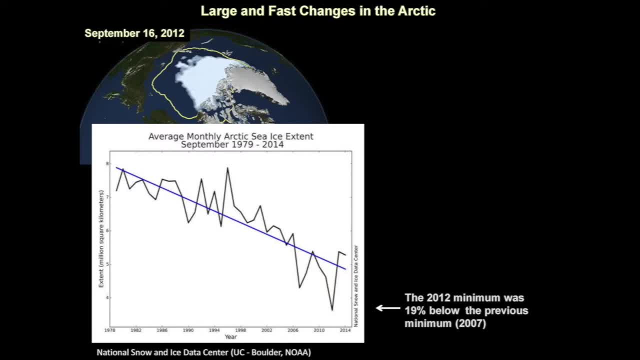 concentrations of greenhouse gases and we can measure that. Our longest record comes from in the atmosphere, actual measurements from Mauna Loa. We measure those gases in the air, bubbles, in the ice And we can take that record back in time to get a perspective. 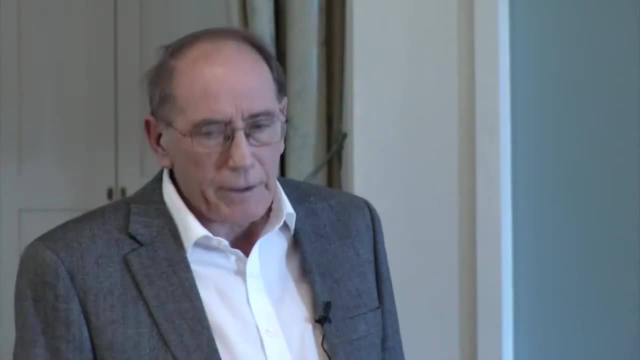 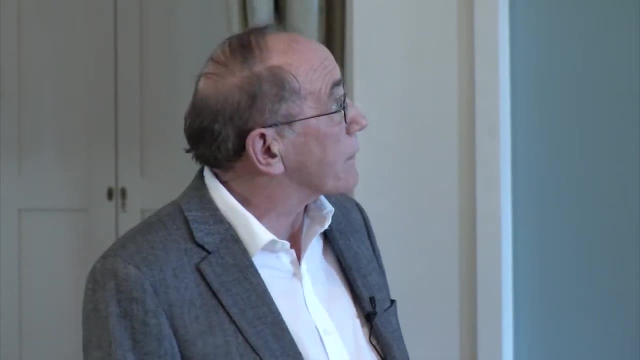 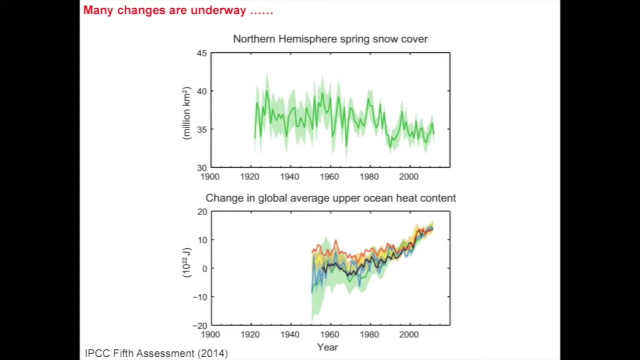 on that. Changes in aerosols and particles also can cause changes in climate. Sulfate aerosols can actually lead to cooling and black carbon can actually lead to warming. So it depends on what types of particles we're looking at. Then there's also changes. 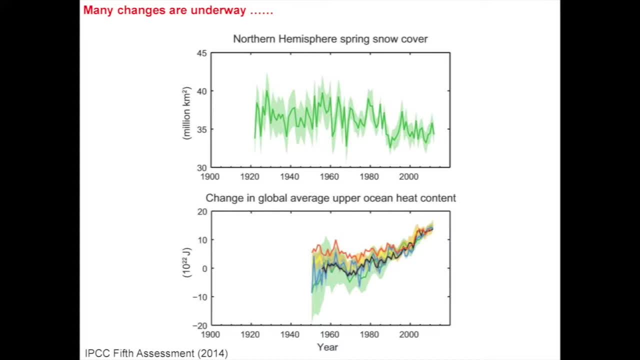 in reflectivity, or the albedo of the planet, as we need more and more land to support what is now 7.3 billion people on the planet, And when you change the surface of the vegetation, you change the albedo of the planet. So there are a lot of different ways. 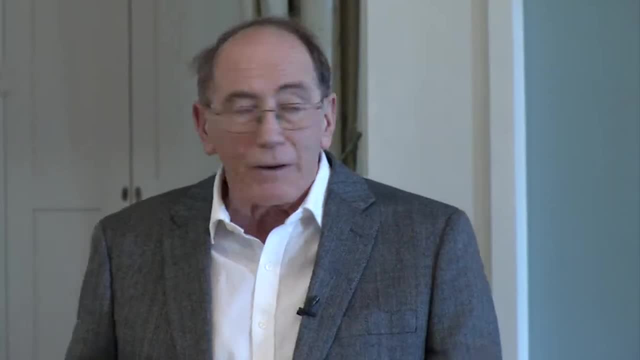 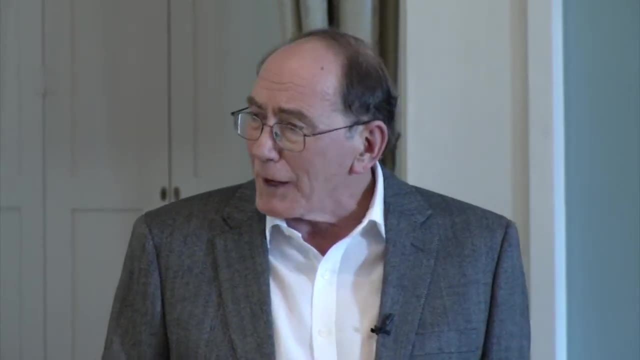 that we are impacting Now. this is, in me, a disturbing diagram. These are the measurements at Mauna Loa that Charles Keeling started. He passed away in 2005.. And if you go to the National Academy of Sciences, when you go into the hall, 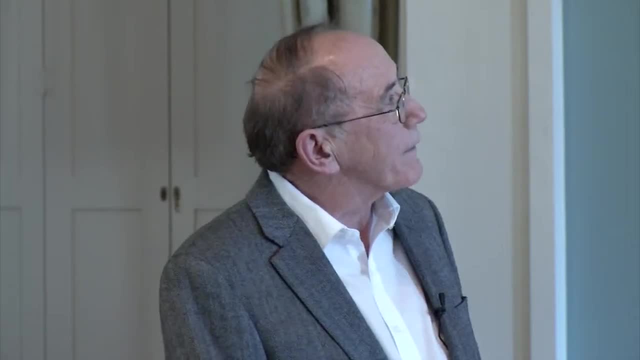 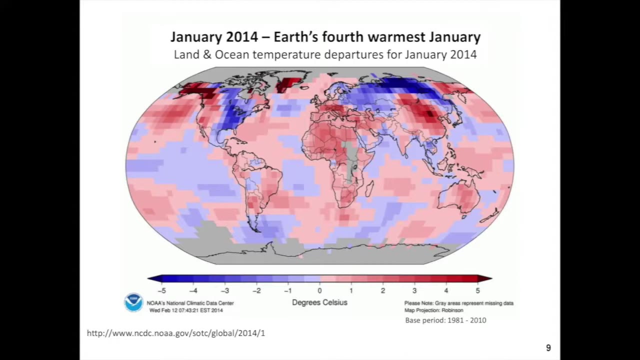 you see this on the wall And, unfortunately, there have been five IPCC reports and if you look at the trend, it's not only increasing, it's actually accelerating, And we first crossed 400 parts- a million by volume- in 2012,, and this year we crossed it in. 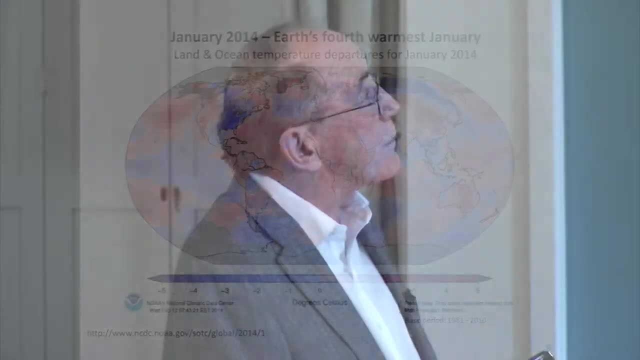 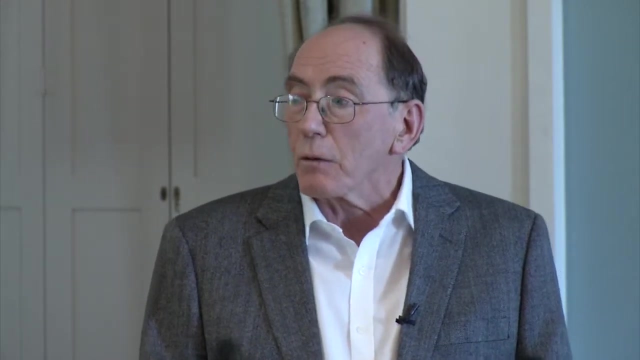 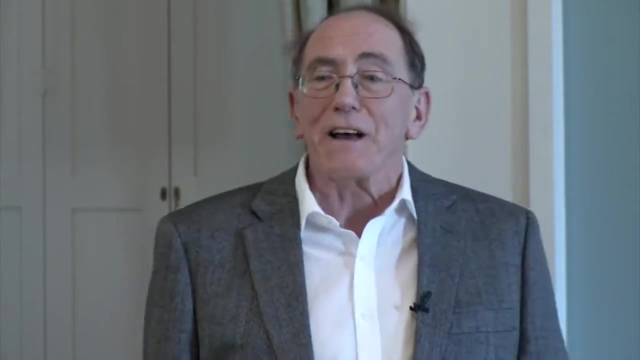 January of this year And we'll probably get up to about 402 parts- a million by volume- later in the spring. Now this is probably to me the most interesting video that I've seen that kind of captures the Anthropocene relative to CO2.. 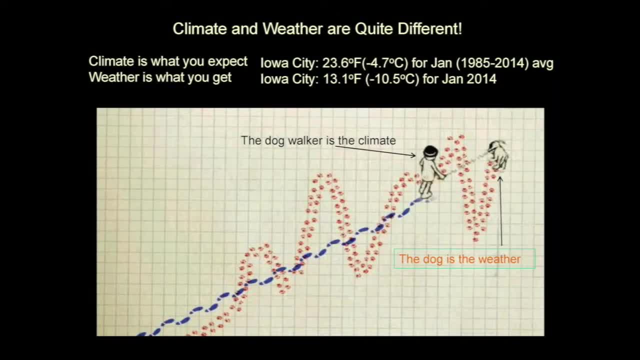 So I want you to take a look at this. This allows you to actually see how CO2 is emitted, where it's being emitted from. This is a NASA video for the year of 2006.. And we'll take a look at that. 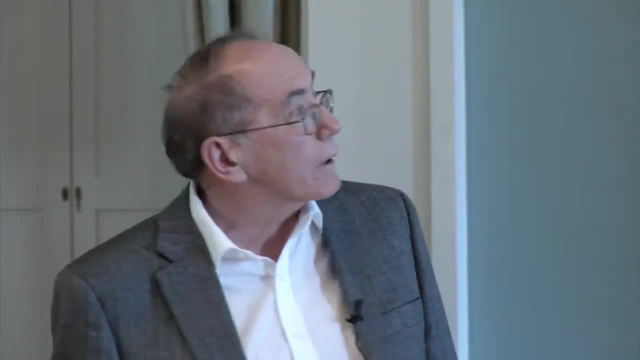 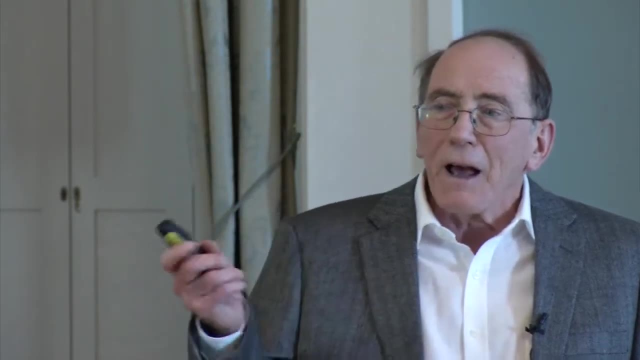 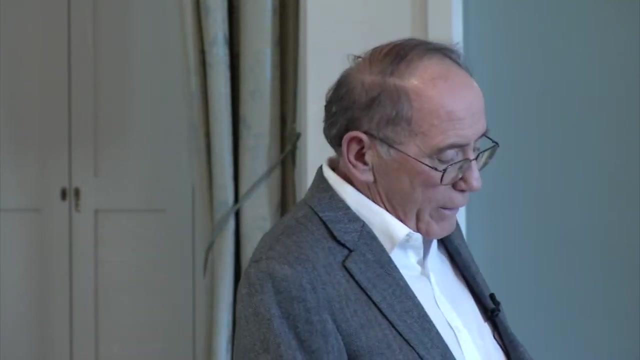 This is Bill Putman. I'm a climate scientist. Two observations in atmospheric models like GEOS-5 will work closely together to better understand both human emissions and natural fluxes of carbon dioxide. This will help guide climate models toward more reliable predictions of future conditions across the globe. 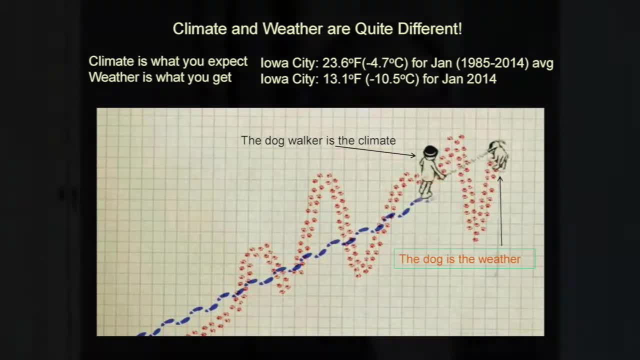 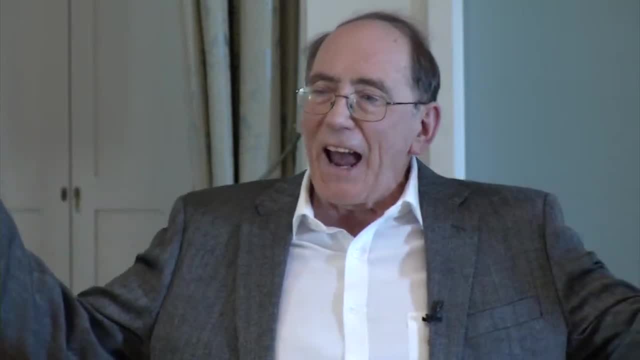 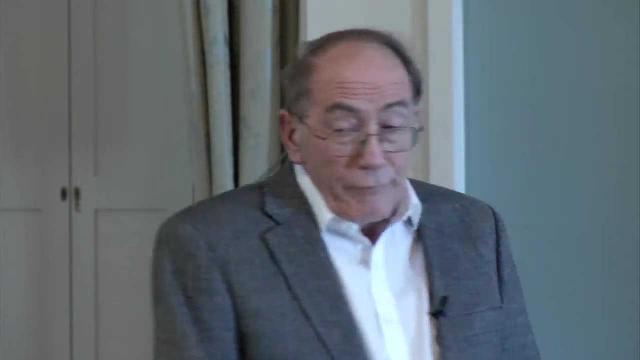 I don't believe I've seen a better video to actually visualize and show you how these concentrations vary and they get distributed and the fact that we all live on the same planet and it's all connected, And to me it's a very telling video. 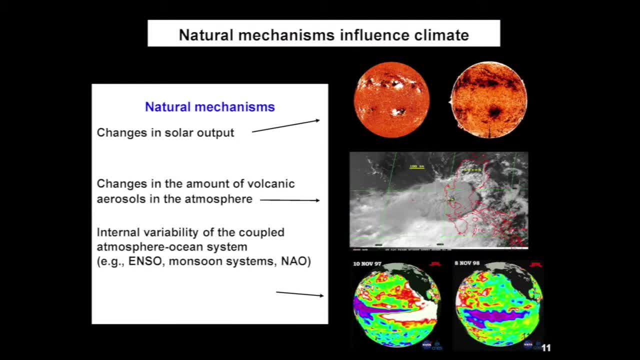 There's always been a natural greenhouse effect on the planet, and that keeps the Earth warm, about 14 degrees C or 57 degrees Fahrenheit, which makes life as we know it possible. So what we're really concerned about is the enhanced, the anthropogenic greenhouse. 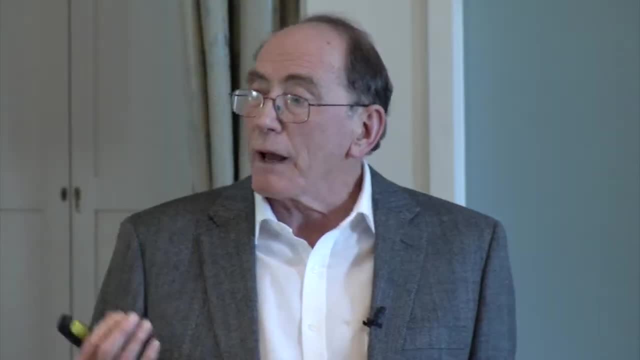 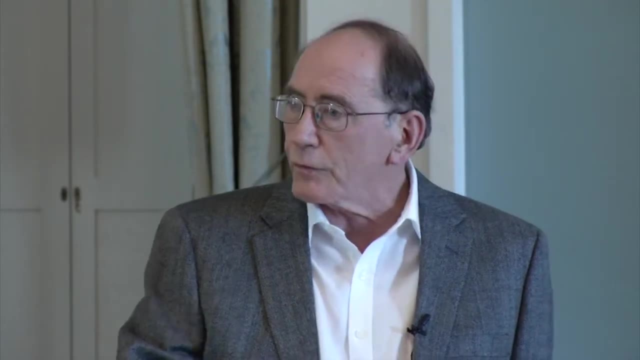 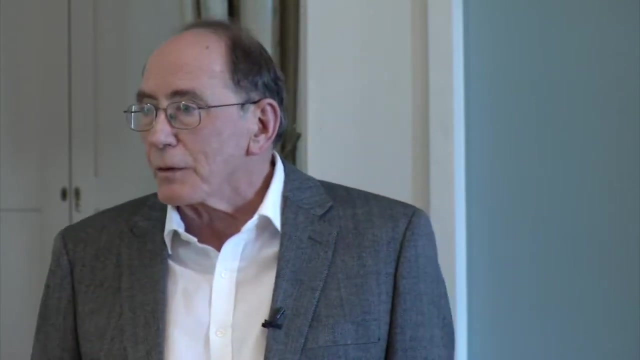 gases that are warming the Earth even more. It's the added effect. This is not new. The science of the impacts of greenhouse gases we've known for over 200 years. But what these earlier scientists didn't know is that we would develop the technology to extract. 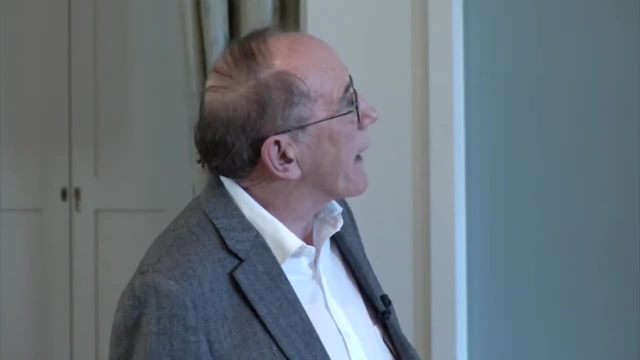 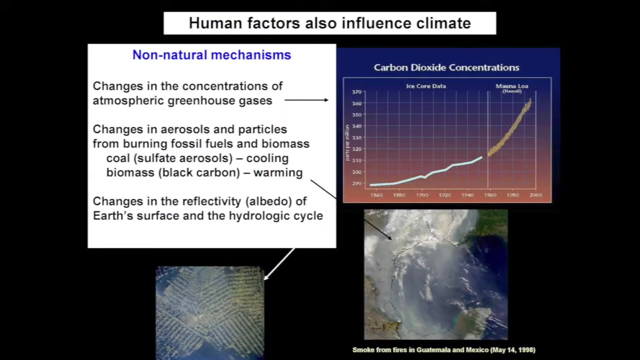 all these fossil fuels, the carbon of the past, and release it so quickly back into the atmosphere. So this is certainly the science is not new. It's based on chemistry and physics. We have models that allow us to look at how any one 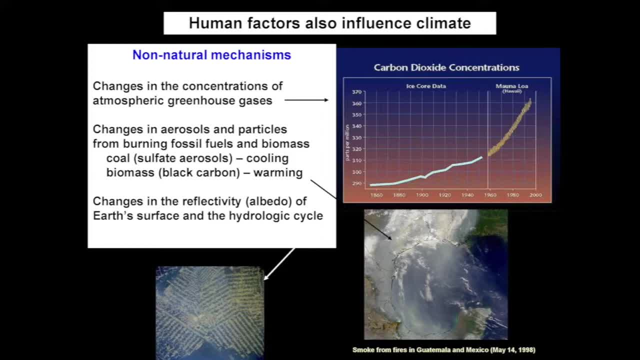 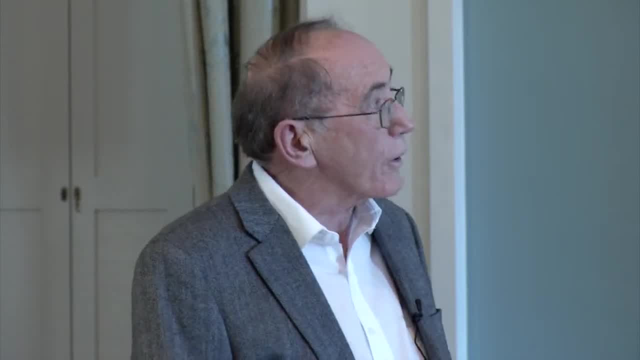 forcing will impact the climate on the planet, And I'm just going to show a couple of these. This is going from the North Pole to the South Pole. This is what you would expect in the atmosphere from greenhouse gases. We expect the troposphere down where we live to warm. But we would expect the stratosphere above to actually cool. If you're looking at changes due to volcanic eruptions, you put material into the stratosphere, tephra and aerosols that will absorb radiation coming from the sun and the stratosphere. will warm and the surface will cool. If you're looking at the driver being the sun, that radiation goes through both the stratosphere and the troposphere. So if you have an increase in output of the sun, a large increase in the last, 200 years. But if you look at the residence time in the atmosphere, you can see that CO2 is 100 to thousands of years. Methane is only 10 to 11 years before it's oxidized into CO2 in the atmosphere. Nitrous oxide is about 150 years. 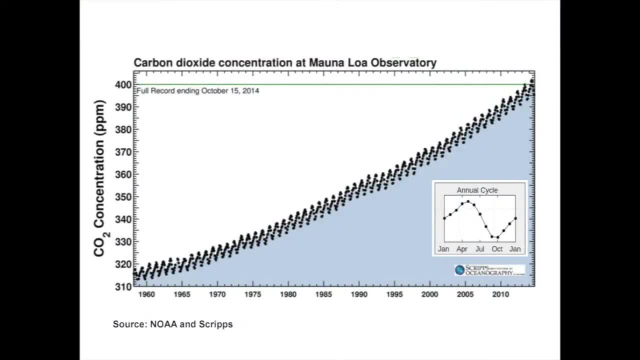 And the CFCs are about 65 to 120 years. So that's why you see a lot of discussions on carbon dioxide And if you say, well, what if we found a solution for our energy needs? We found alternative energy and we stopped. 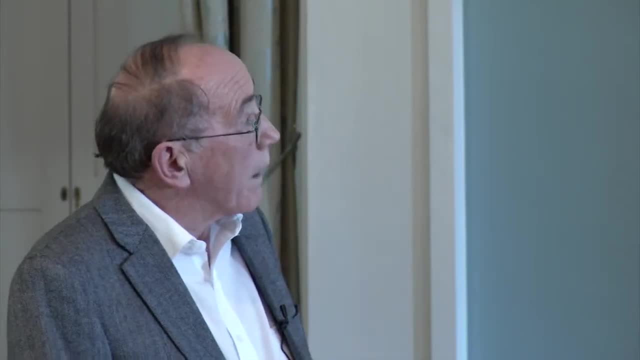 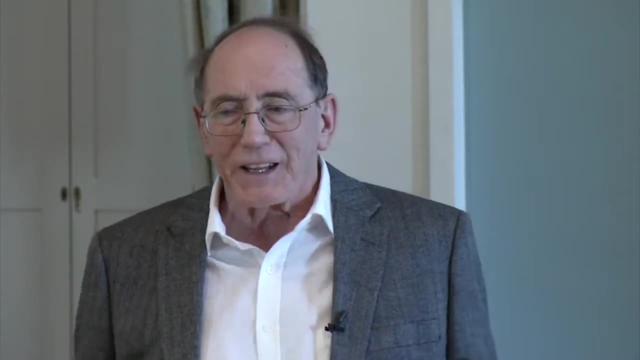 producing CO2 tomorrow, which is not going to happen. How long would it take the CO2 to decline in the atmosphere? And this is looking forward in time And you can see when you're out 100 years you'd still have about a third of the CO2. that's currently in the atmosphere. When you're out 1000 years you'd still have 20%. So it's going to take a long time to turn the impacts of CO2 on the climate system, And it's kind of interesting to look at our best estimates. for when did we have about 400 parts per million by volume of CO2 in the atmosphere And we have to go back in the geologic record to about 3 million years, to the Pliocene, And in the Pliocene temperatures were about 2 to 2.5 degrees warmer. And sea level was 22 meters or about 72 feet higher, And so this kind of shows the shoreline on the east coast during that period of time And that water was coming from. these are the ice sheets in Greenland and Antarctica today, And this is the projection of what they. looked like about 3 million years ago. So those were the sources of that water. So the drivers are really us in a big way. This is the population of the planet. So we're at 7.3 billion, Estimated to be at 9. billion by 2050.. But it's not just this, It's what we need. So if you look at in 2013,- just animals that we needed to feed these people, We have over 30 billion fowl. These are chickens and ducks and things. that we need to support 1.9 billion sheep and goats, 1.4 billion cattle, 1 billion pigs, 400 million dogs- I have three of them- 500 million cats. You know this is a requirement And this doesn't talk about the crops and things that we also need. And you can compare these numbers to the pre-exploitation number of American bison in this part of the world. There were only 60 to 80 million. So humans are having tremendous impact in so many ways. You've probably all seen this picture of the Earth. from the International Space Station. About 65% of the world's electricity today is coming from fossil fuels. But what's really interesting is if you look at what the world is expected to look like by 2030 at our current rates of growth, So that's only about 15 years from now. So this is from General Electric. This is what they expect the Earth would look like at night. on our current rate, We have over a billion people that do not even have electricity in the world today, And one of the aims is to bring electricity, which is very important. to the lives of people around the world. So the real question is: where is that energy going to come from that supports this growth? Well, we've been looking at ice cores for the last 37 years. We have these long records, like the one I showed, from Antarctica going back 800,000 years. 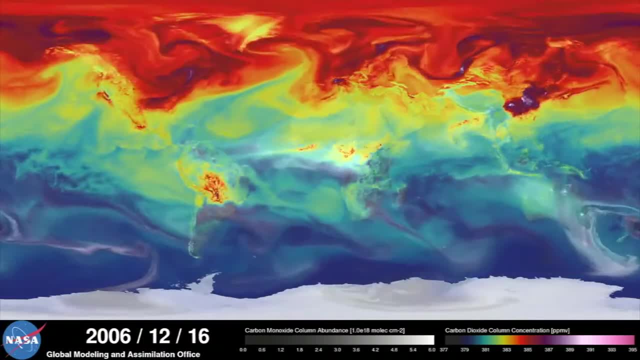 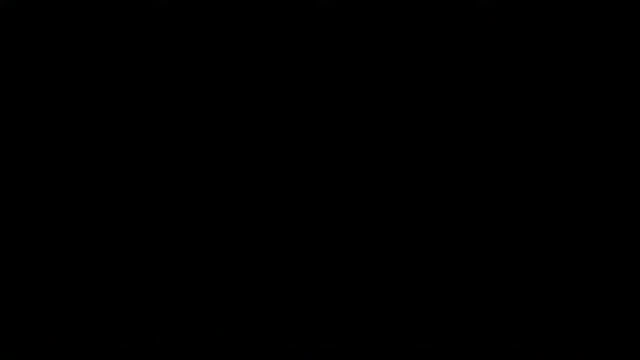 We also have long records out of Greenland, But we've also been looking at the high mountain regions in between. This is a view of the Kilkiah ice cap margin in 1977, back when I was a graduate student, And this is the same place. 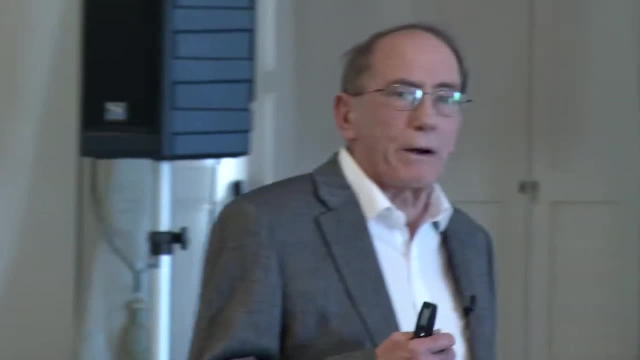 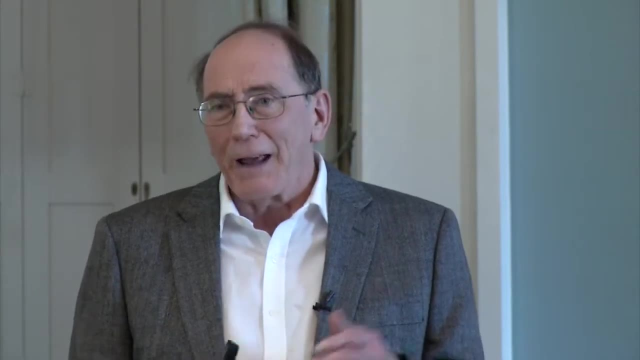 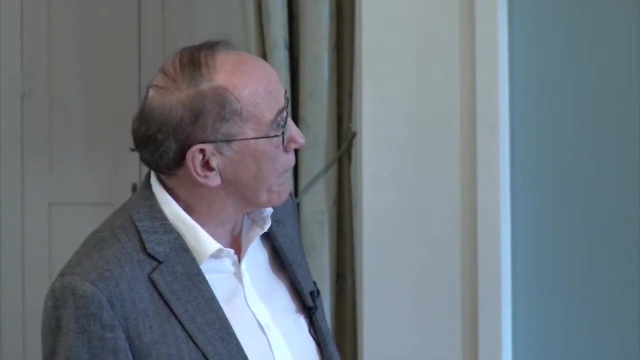 in 2002.. And so it kind of brings home the picture that not only are you losing a very important history of the past, but you're also losing a very important water resource. There are many things we can measure in the cores and where you have very distinct wet and 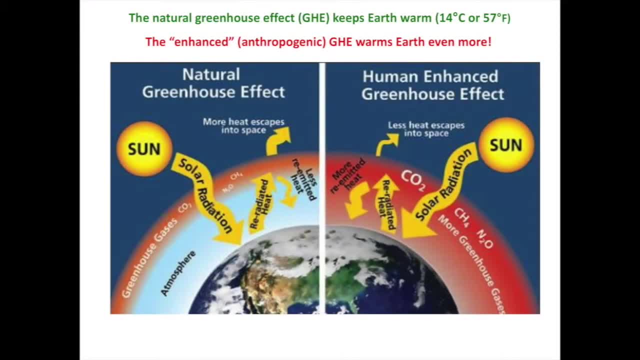 dry seasons, like in the monsoon or down in South America, you can actually see these annual layers in the cores when you're recovering them. And of course, you have to have laboratories. We have class 100 clean rooms, mass specs. We have over 7,000 meters of core stored at. 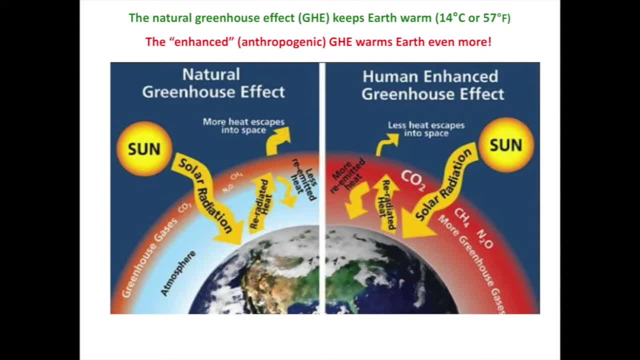 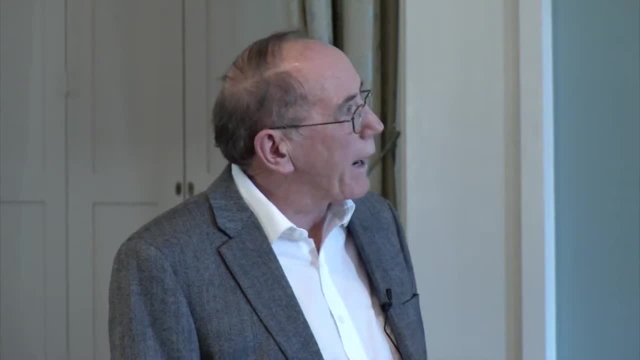 minus 35 degrees C. It's the only tropical collection of ice on Earth And it's becoming more valuable every day, as I'll show. And we also design and build the drills: lightweight equipment that allows us to get up to above 20,000 feet. 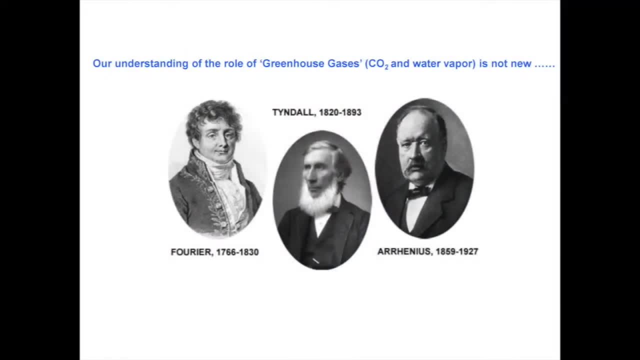 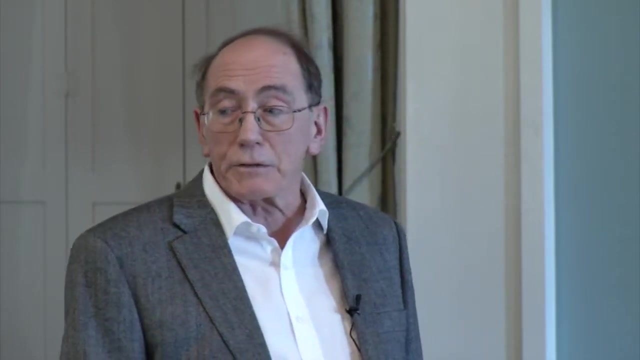 to recover the cores. This is what a typical high mountain drilling operation would look like, And we experiment with different types of energy- Solar power, special diesels that work in cold environments to provide the energy for these, And so we've been drilling at these. 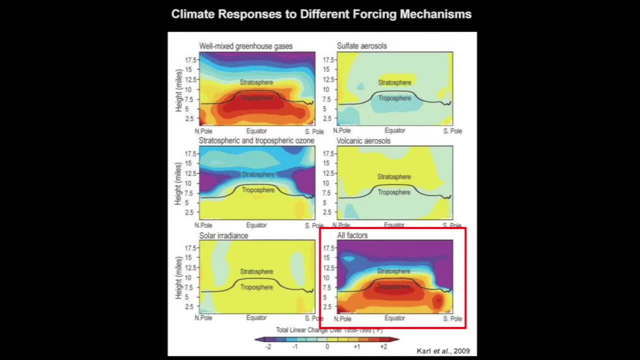 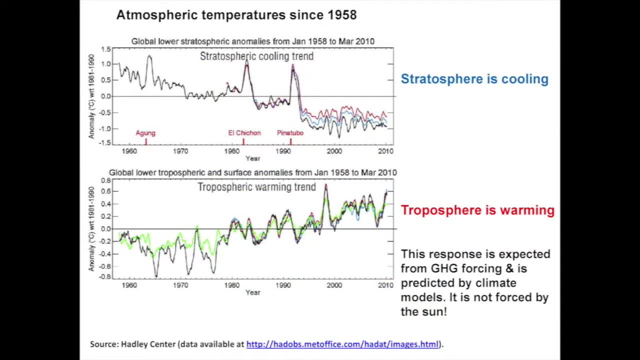 on these mountaintops, And I'm just going to show that these records in the tropics actually span very long periods of time, And when we started, no one, including us, believed that we could get histories that go back into the last ice age from the tropical mountain glaciers. 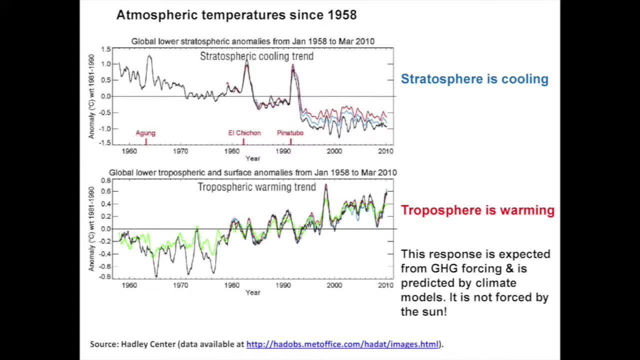 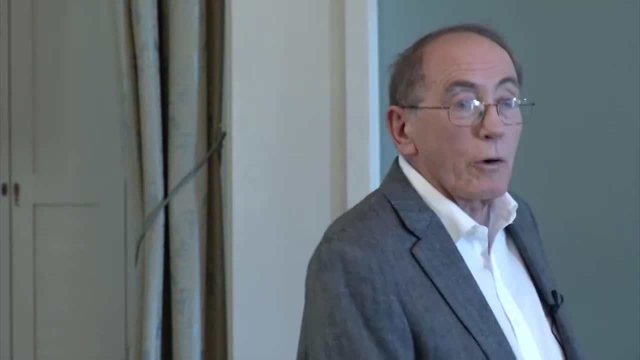 But this is just one. This is Huascaran. It's the highest tropical mountain on Earth And the drill site is right in here in the call, And the reason you need very lightweight equipment is that they have to go across crevasses and you have to use porters. or you have to carry this equipment up: Six tons of equipment, Set up the drill site and, in this case, 53 days later, bring that six tons of equipment plus four tons of ice, frozen ice down and keep it frozen and get it out of the tropics and back to the. freezers at Ohio State. We have through time improved the drills that we use, The power for those. So two cores to bedrock, We always do two so we can look at reproducibility of records. These are 168 meter cores. And you can see that in the upper part. you can see this very, these annual variations since the last hundred years. You see it in the isotopes, You see it in the dust records, You see it in the nitrates which is related to vegetation in the Amazon. So they're very high resolution. records, And this record goes back almost 20,000 years. So it was our first view of actually being able to look at what the isotopic record looked like in the tropics during the last glacial period. Up until this date, they only were found in. Greenland and in Antarctica. We could also look at nitrates, which are very low, which suggests lower vegetation out in the Amazon, in the source areas, And the dust increases a hundred fold, which suggests it was much dustier in this part of the world at that time. So you can reconstruct that history. So over the last 37 years- this is the place where places our team have recovered ice, And the whole idea is to put together a global picture of climate as it's recorded in those glaciers. I think we often forget that we live on a sphere And because of that we have 50%. of the surface area of the planet. actually in the tropics Between 30 north and 30 south. We have 70% of the people that live on this planet in that same zone, So it's an important area to understand. It's also where the water vapor, our most important greenhouse gas. in the system is being pumped into the atmosphere, And these actually show the drill sites in the lower latitudes, where we now have records. I'm going to take you just to one of these down in the Kalki Ice Cap, because it's such an. unusual part of the world. We first drilled this ice cap in 1983. And we did that using the first ever solar powered ice core drill. And back in 1983- solar power, the technology was not very well developed And we got a lot of pushback that this would be impossible. But it was the only way that you could get a power source into this remote part of the world. It was a two day journey by horse. So all these horses and these bags are the panels And you can see the drill cable here. And this was the setting, And this was the first solar powered drill that was developed. And not only did we drill one, but we drilled two cores of bedrock from this ice cap, 168 meters, using solar power. This is an unusual ice cap. You can see the drill site here. This is in the tropics. We're only 14 degrees south of the equator, 150 kilometers to the east. you're in the Amazon basin. You wouldn't think there would be so much ice at this latitude, And if you look down the crevasse on this glacier, you can see those. annual dust layers every dry season. If you go into the crevasse, you can actually see how uniform these layers are, And if you get an ice core, you can actually measure the thickness of the layers and reconstruct what precipitation has been in the past. And so this is what an ice core looks like when it's recovered And the records are brought back and they're analyzed. and these are isotopes. These are a temperature proxy And they show the annual variations at this site, And every dry season there's a dust layer. And so you can go back in time, And this record actually goes back 1,800 years. This is the last thousand years. This is the isotope record, decadal averages from the 1983 core, which was brought back as bottled water samples, And then we went back 20 years later in. 2003 to bring back ice cores. We had developed a technology to keep the ice frozen, to get it back so we can preserve an archive for the future. And if you look at these first of all, you'll note the reproducibility of the record over a 20. year period And you can see in this record that it was warmer in this part in the medieval warm period- Little ice age- And then you can see the warming in the 20th century. You can look at those annual layers and reconstruct the. precipitation, The net balance record. The browns are dry periods. So this period is warm and dry. The little ice age starts. wet Becomes dry. You get into the 20th century. Precipitation has been above average. So you can reconstruct these histories back through time. 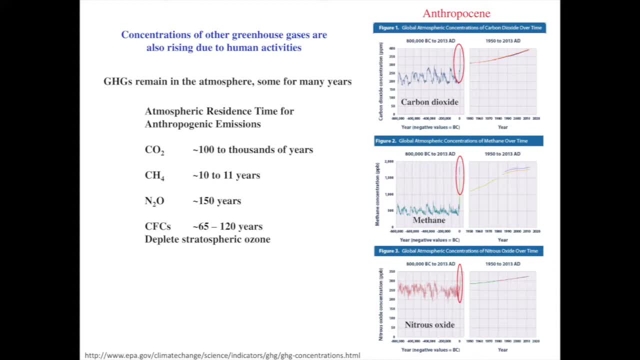 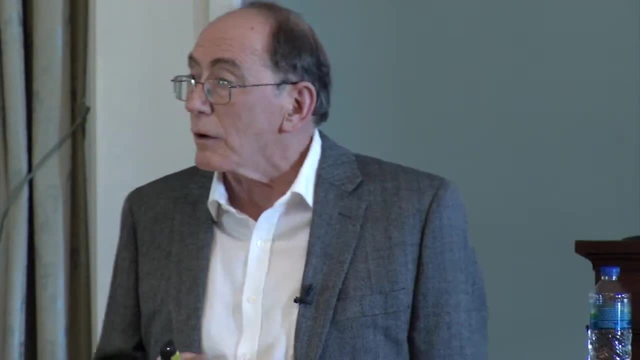 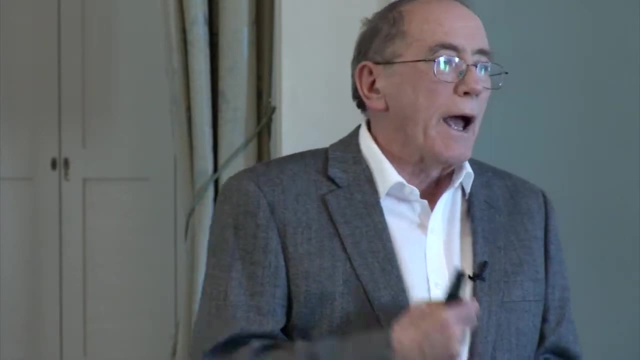 This part of the world is impacted by El Ninos that have tremendous global impacts on precipitation patterns, And if you're in South America, the northern Peru and Ecuador are very wet during El Nino periods. Southern Peru is very dry And what we found is that, if you look, 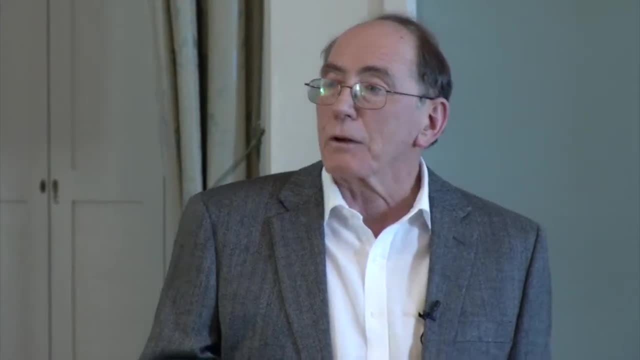 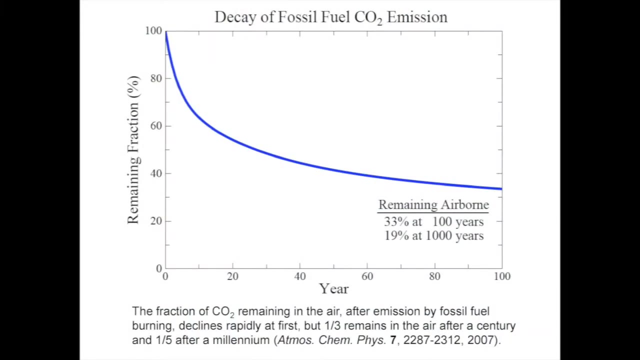 in this part of the world, If you go to pre-Spanish time, there have been many cultures and empires. This is the Inca Empire And with this annual record, we can work with archaeologists and anthropologists and actually look at how precipitation and temperature was varying during the times of rise. 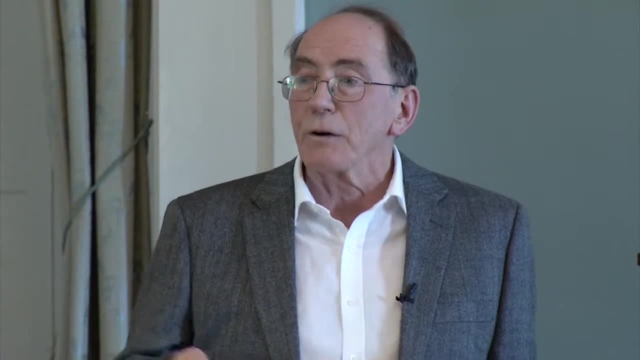 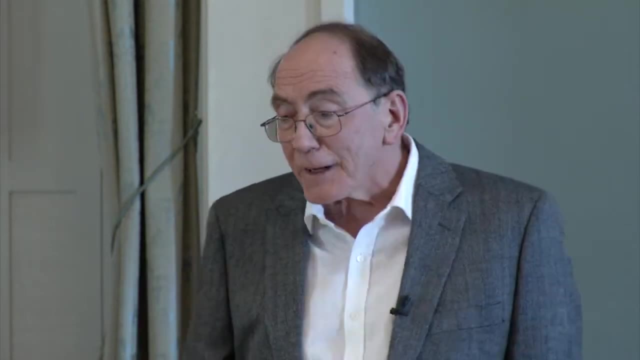 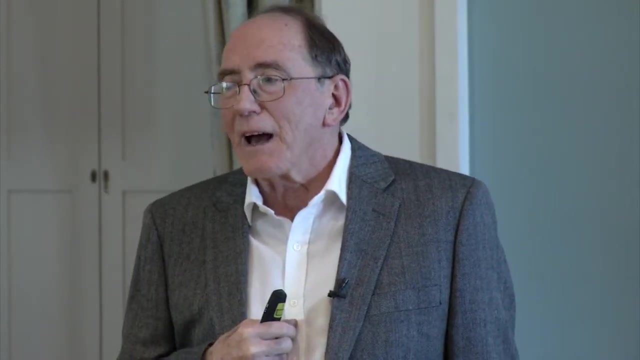 and fall of those cultures. And if you do that, and these are the blue curve, here is precipitation. The high precipitation is blue. The droughts are indicated here. When you look at that through time, these are cultures. The Moche culture was a coastal culture. 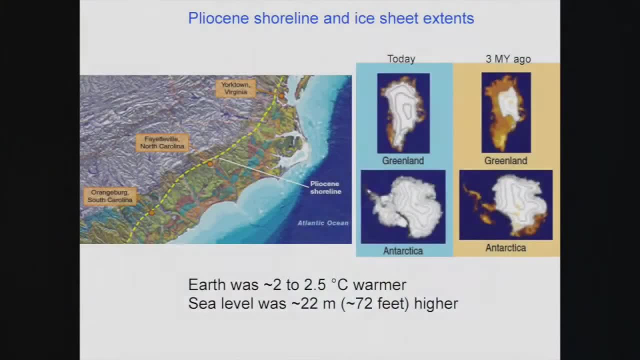 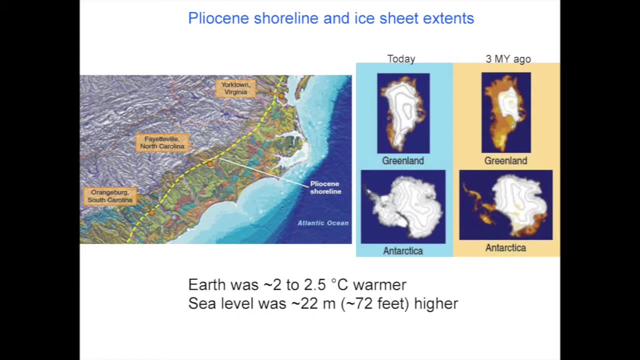 And the capital was on the coast. When you get into the wet period in the highlands, we have the development of the Tiwanaku and the Awari cultures And the capitals move to the highlands. When it becomes dry in the highlands again. 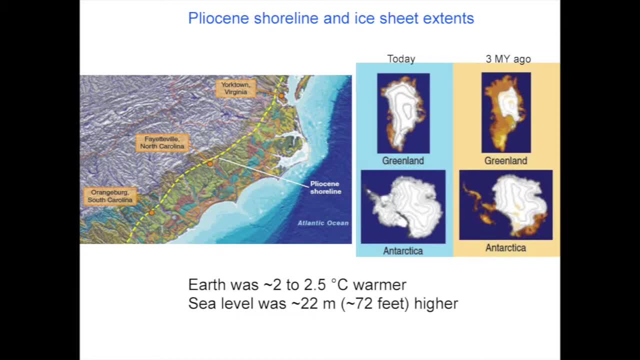 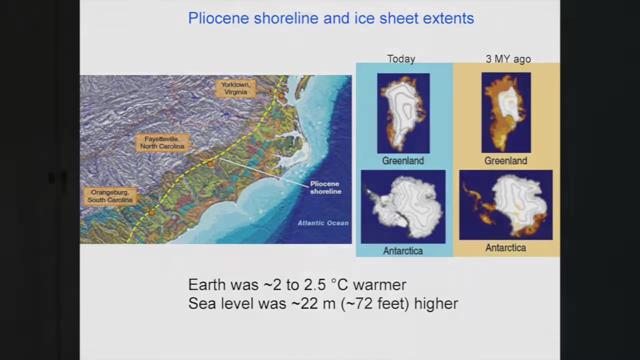 these cultures- in this case it's the Chumu culture- and the capitals move back into the coastal area And then, when the rise of the Inca's is during this period, when it's getting wetter again- And this was the largest empire developed in that part- 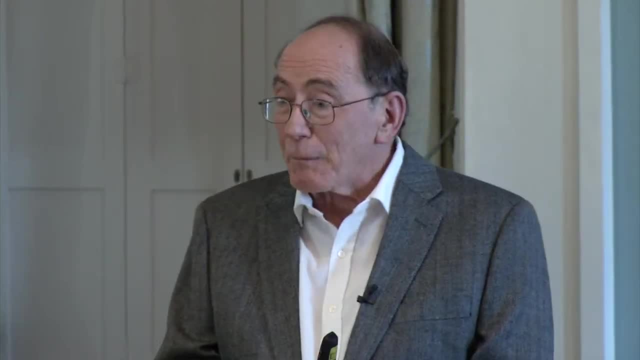 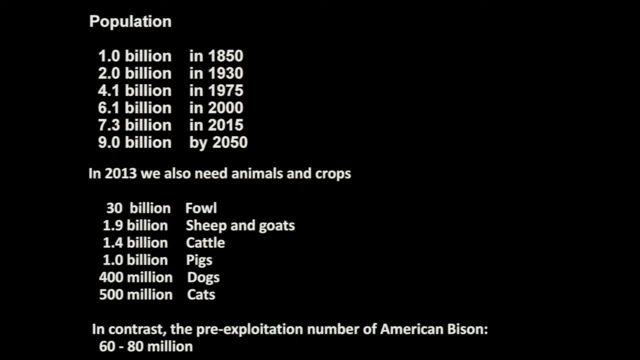 of the world And of course it came to an end when the Spanish arrived in 1531.. But what is interesting is if you take that history of how people have moved through time and you look at where we are today, In the last hundred years it's been wetter. 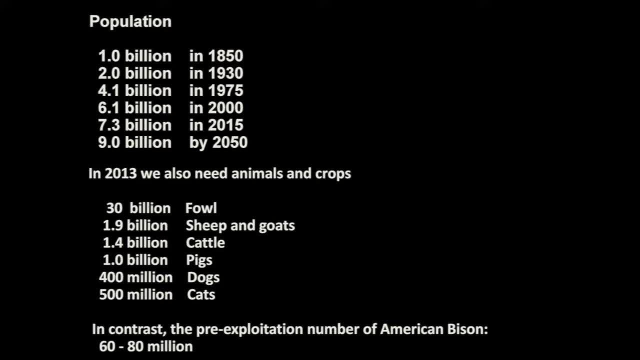 than average up in the highlands. Based on the past, people should be moving to where the water is, But since 1947 people have been actually moving from the highlands to the coastal desert, To places like Lima, Peru, looking for a better way of life, education for their children. 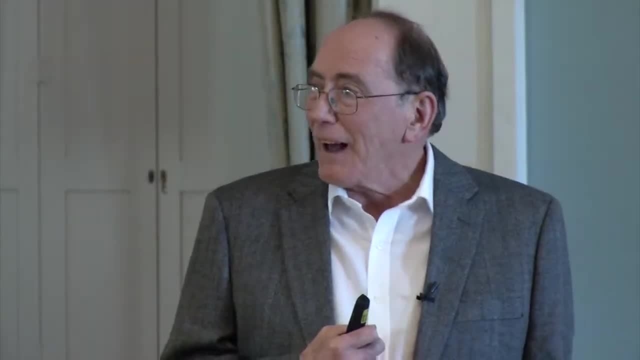 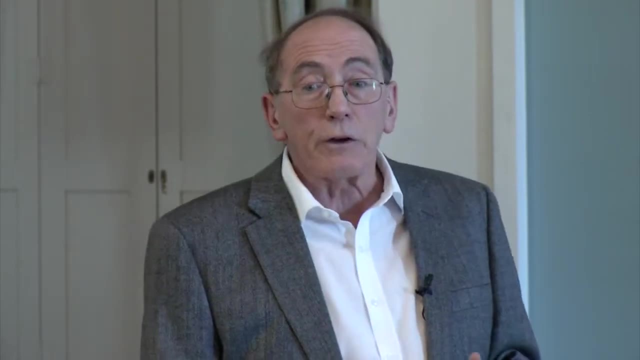 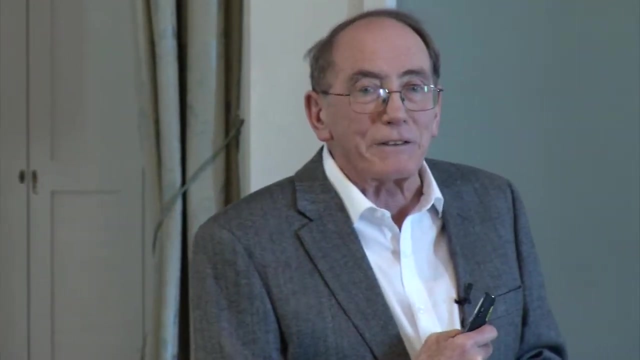 And now over 50% of the population in Peru is actually in the coastal desert And they have huge water shortages In that country. 86% of their electricity is from hydro power. That water also is used for irrigation. It's also used for municipal water supplies, And Lima, Peru, has severe 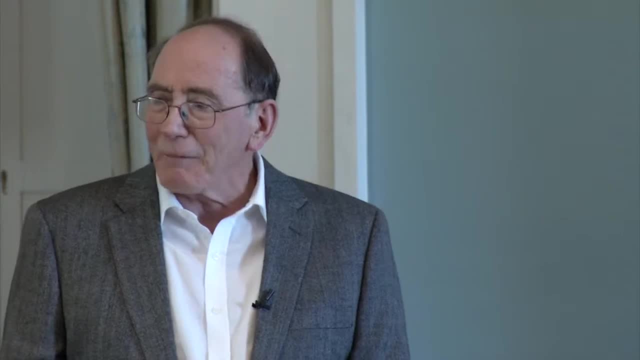 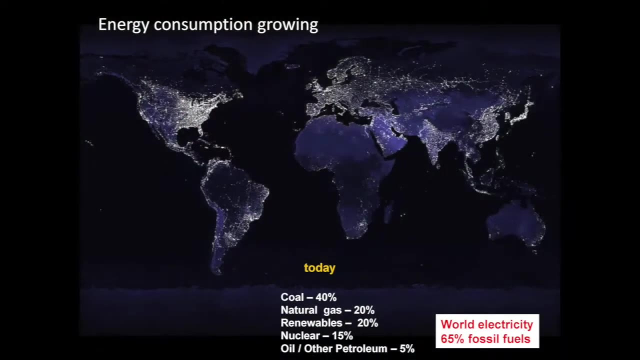 water shortages today And now they are talking about putting in tunnels through the Andes to capture water that goes into the Amazon and bring it across for their city. But it's a lot of policy. Peru is the biggest asparagus producer on earth. now They produce asparagus out in the desert. 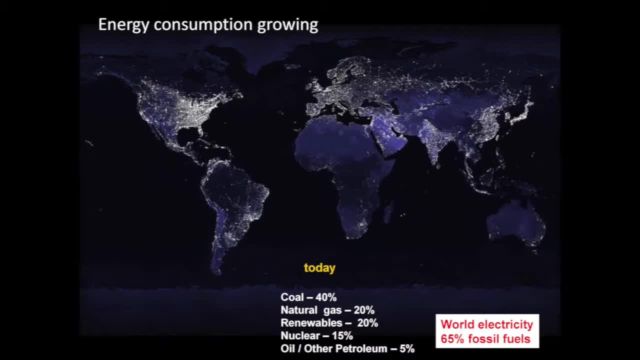 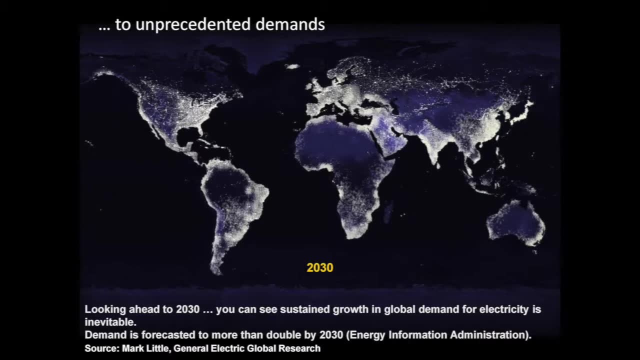 So they have to divert water from the Santa River in order to do that, And the question is whether these things are sustainable, And there certainly we can raise similar questions here in this country. If you look, you can look at the impact of climate on people. 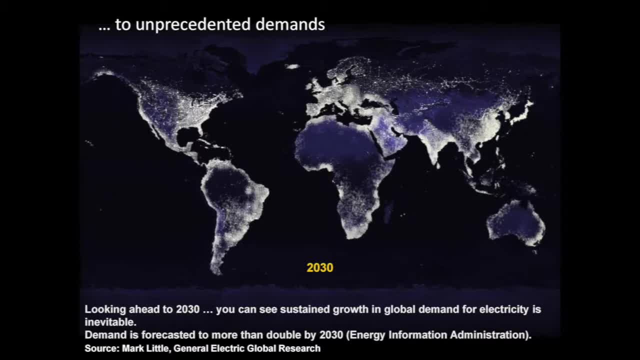 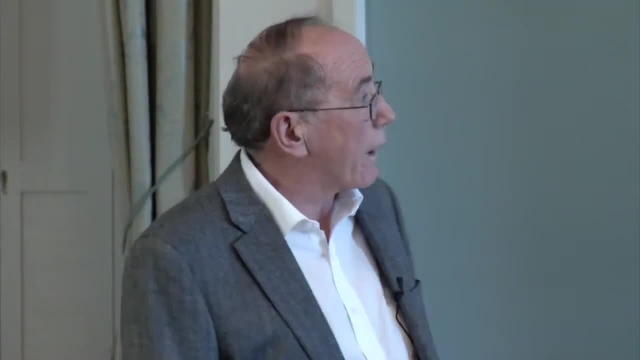 But you can also look at the impact of people on the environment And in this part of the world mining has been a big issue. It was developed in these pre-Spanish cultures, But it really took off when the area was colonized. 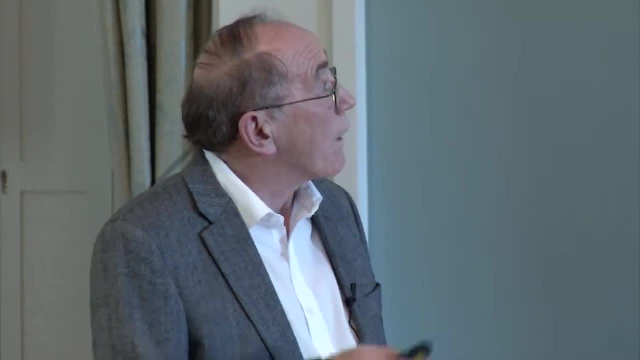 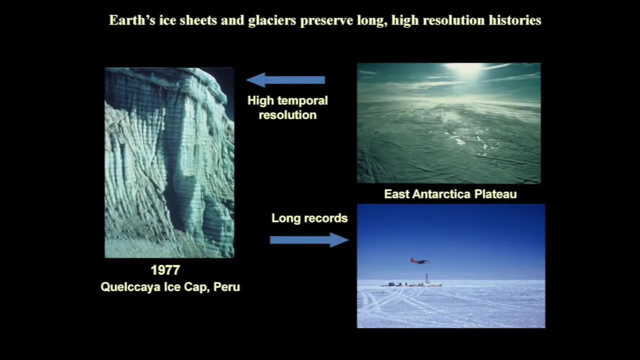 And this is actually a silver mine that is underneath a glacier They're actually going in. So just two weeks ago, in the proceedings of the National Academy, we had a paper that looked at lead in the ice core as an indicator of mining activities. And so here's the Calcai ice cap, and there are 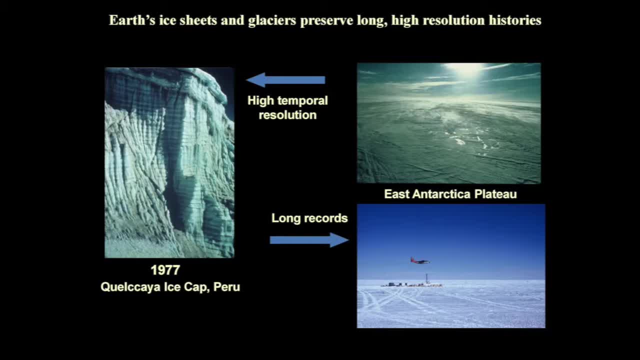 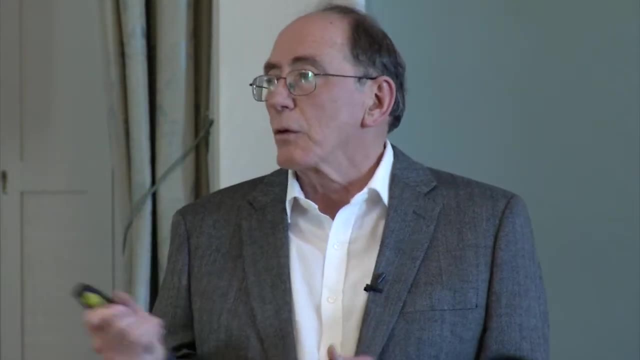 three lake records here, And this was Potose was a huge mining operation down in Bolivia And if you look at these records you look at the silver production from the New World, from Peru, and Potose miners were losing jobs because they were being 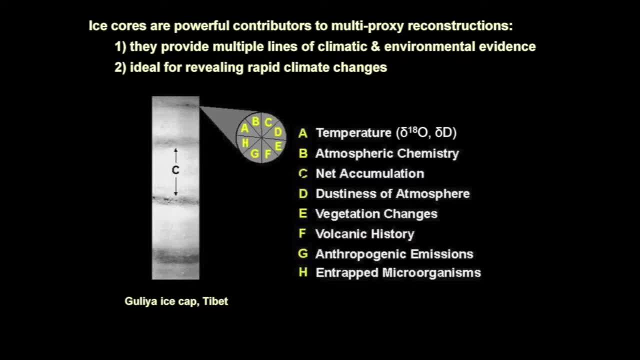 replaced by technology and machines and the like. So I go back and I talk to the young people: If you want to have a future, you look at the alternative energies. This, to me, is the growth area for the future. But humans being what we, 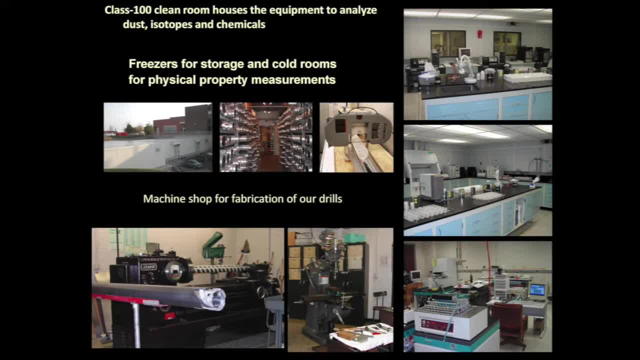 are. it's these extreme events that actually get our attention, And I'm just going to go very quickly through the last couple of years. In 2011 in Ohio, it was the wettest year on record And we had many floods. These are very expensive when they 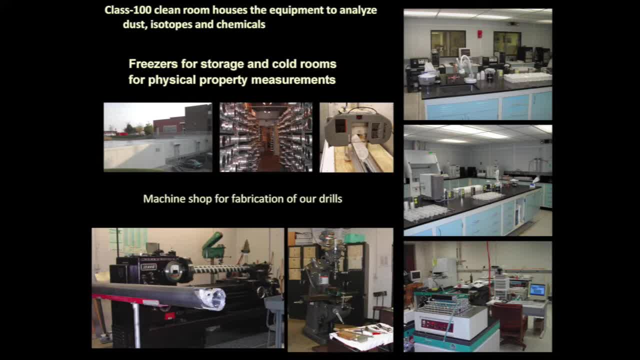 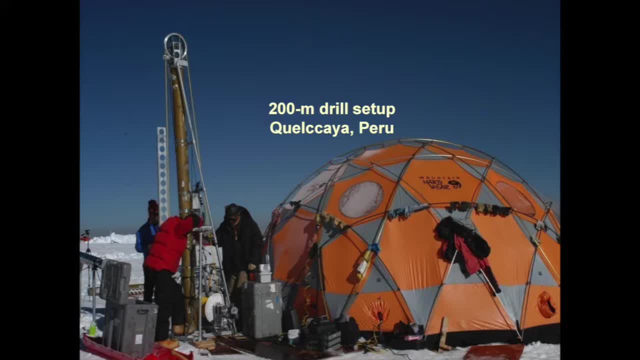 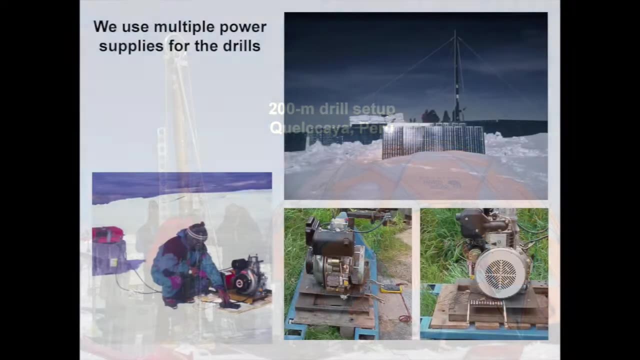 occur, But this is a global. This is 2011.. This is in Pakistan, And Munich Re, who is one of these companies that insures insurance companies and distributes the risk globally, actually sees the impacts of these changes. So the overall losses in 2011 were 148 billion. 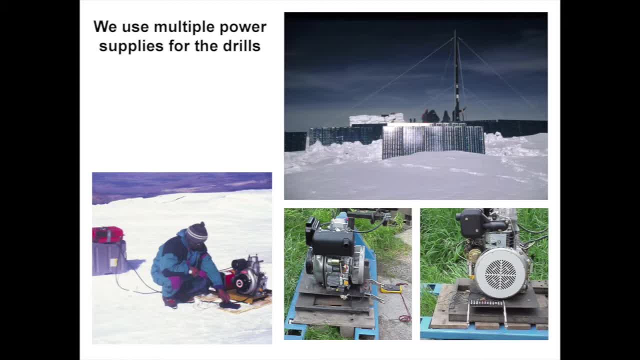 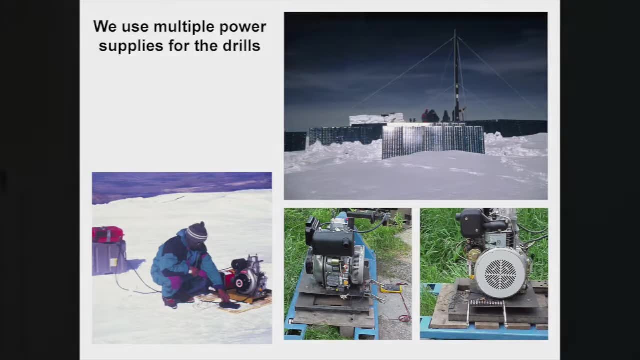 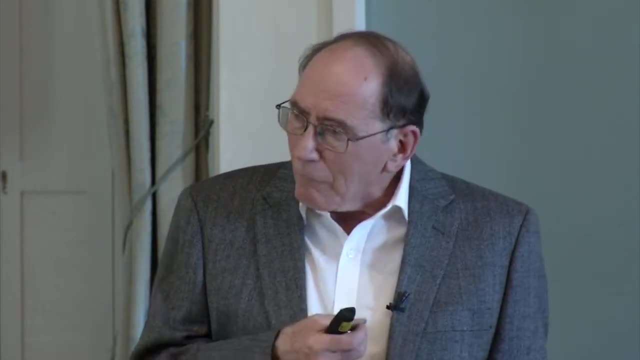 weather related losses, of which 55 billion was actually covered by insurance. The rest was picked up by taxpayers or individuals of those costs. In 2012, we had super storm Sandy And you see super in front of typhoons and things now. And they're still trying to recover from this. It's cost over 60 billion dollars, But some things you don't often note is that there are 45 super fun toxic waste sites within a half mile of the coast in New Jersey and New York And these become at risk. 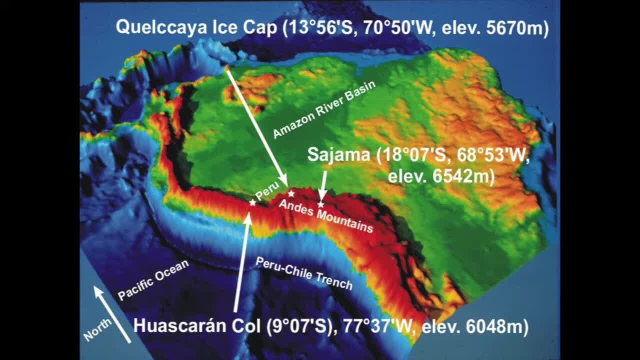 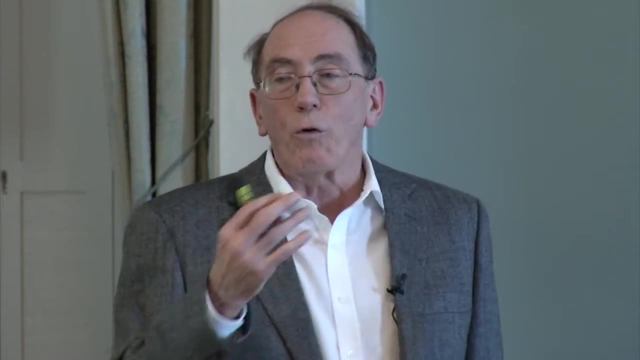 when sea level rises and you have potential higher and higher storm surges coming in. You look at fires in this country. These are record fires And what again is so compelling is the timing of these. We're talking about areas burning the size of Massachusetts and Connecticut combined. 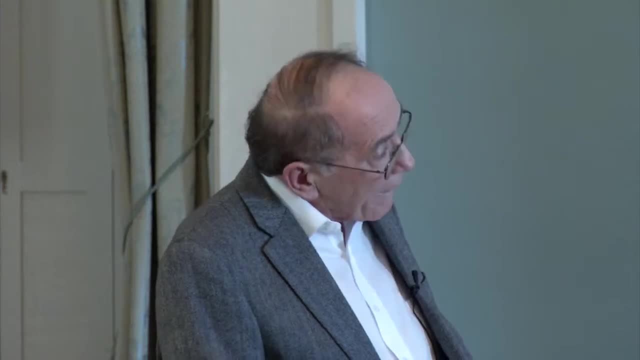 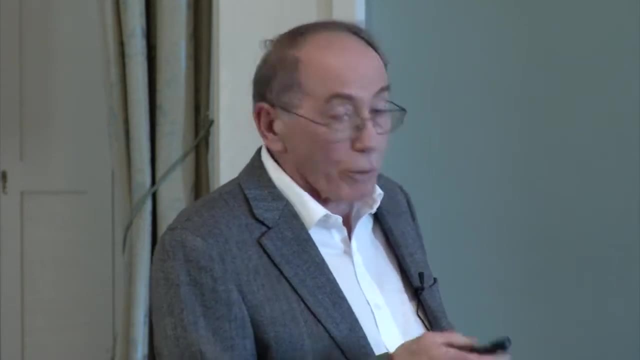 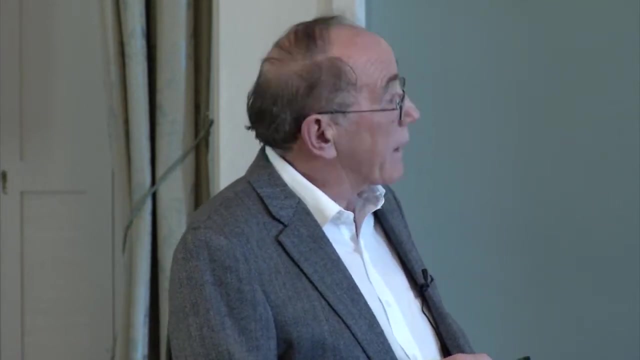 2006,: 9.8 million acres. 2007, 9.3. 2012,. 9.1 million acres. These are tremendous impacts. The flood in 2013 in Boulder, Colorado. It doesn't flood in that part of the world And most people did not have flood insurance. 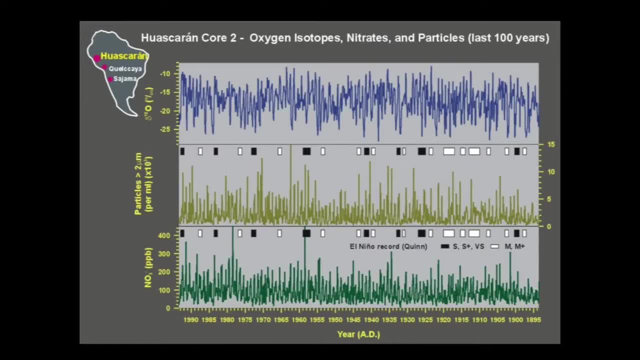 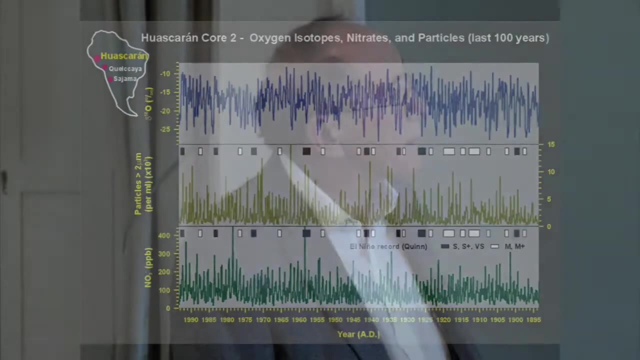 because they haven't needed flood insurance. And this brings up one of these characteristics of human beings: The fact that the consequences for the individual outweigh consequences for others. If it's your home that's going into the river, then you become very concerned about these changes. 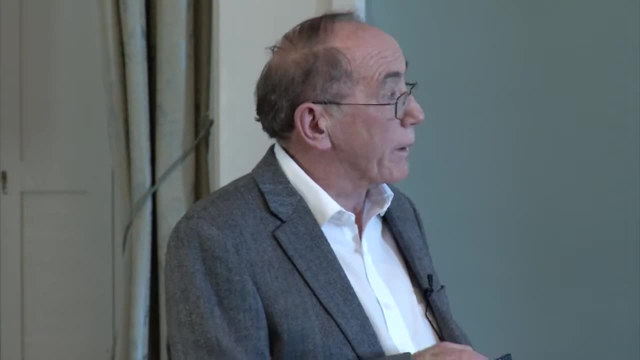 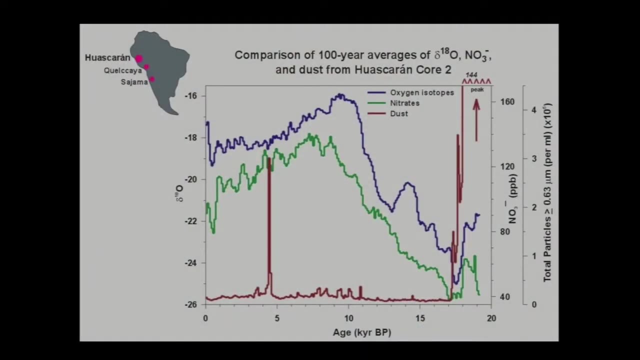 This is super typhoon hiding. The death toll was in the thousands and the damage is 14 billion. Only about 2 billion was actually insured in the Philippines. This is a poor part of the world. Most people don't have insurance. Then you come to last winter. This is: 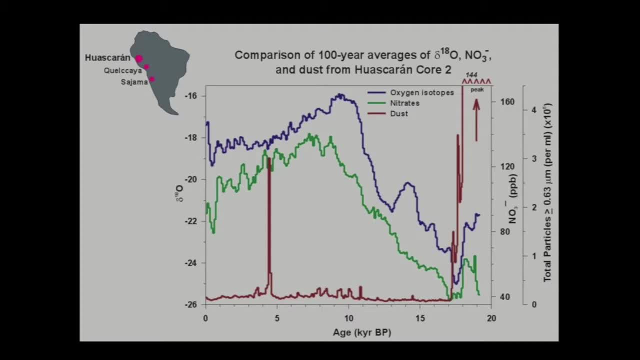 ice and freezing rain in Atlanta, Georgia, Very unusual in this part of the world. But at the same time, if you went to Australia, record temperatures were being set in the summer there, And this is why you always have to look at the global picture. 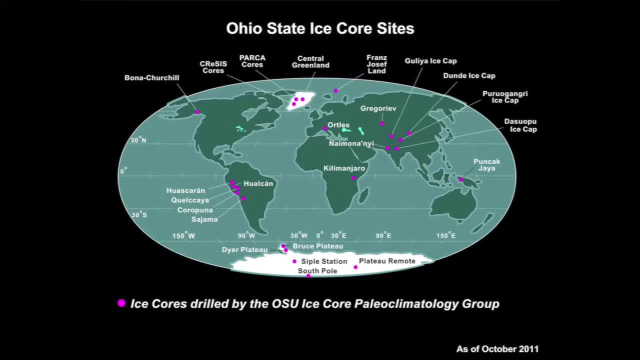 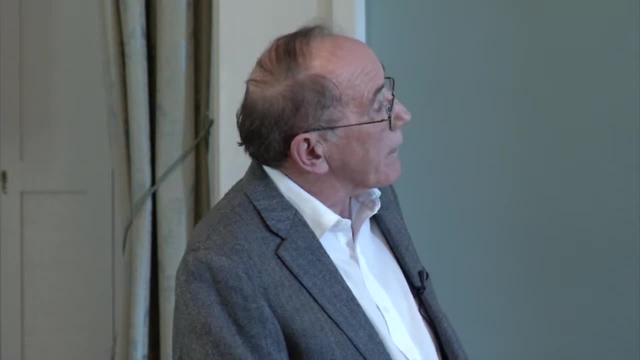 And the floods in England in 2014.. The losses were 1.7 billion. The winter of 2014 was the wettest on records since records began in 1910 in that part of the world. And then you come into this winter. 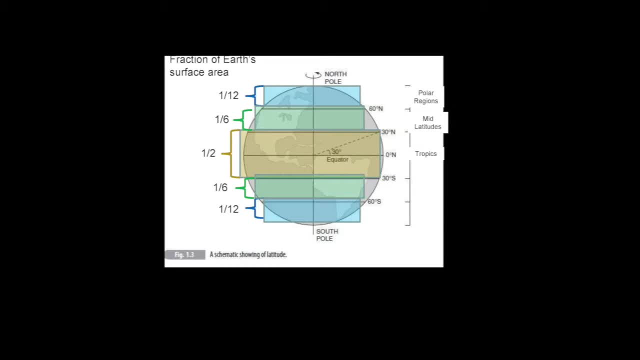 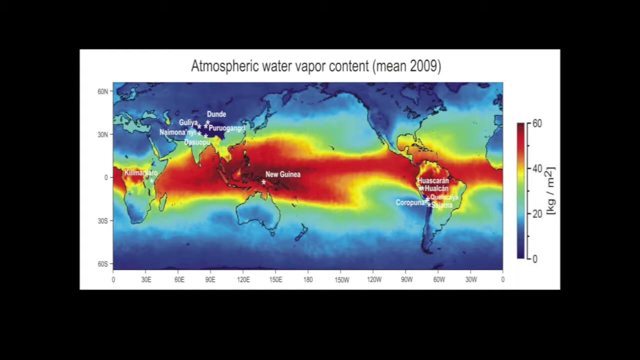 and the snows in Boston. Chances are they're going to have a record snowfall, since they've been keeping records in that part of the world And the impacts of these are tremendous on infrastructure and people. Last seven feet of snow. I mean that's a lot of snow. 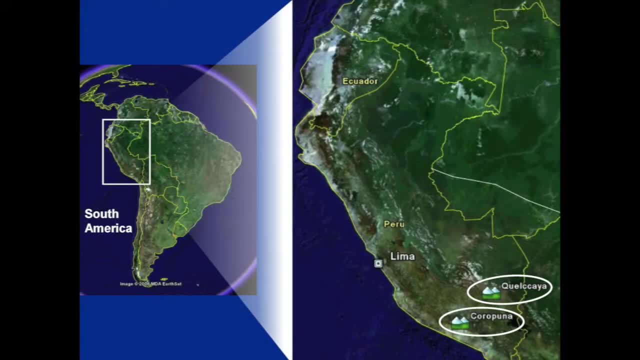 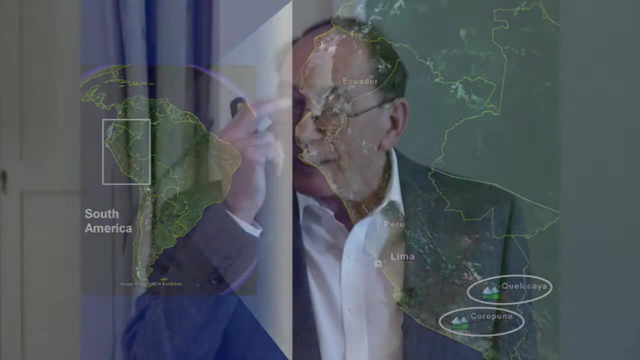 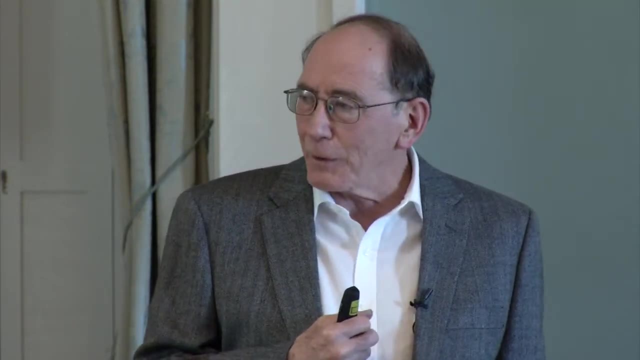 Um, So and then, if you look in California, the drought out there It's now a 500 year drought And this is what the drought situation looked like in 2012,, 2013, and then last week and now. And if you look at the snowpack up in Sierra Nevada, it's only one-fifth of 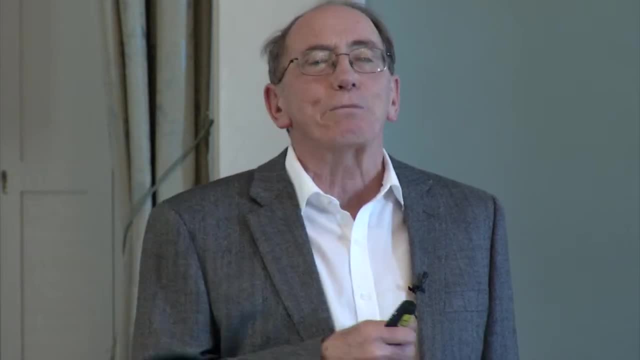 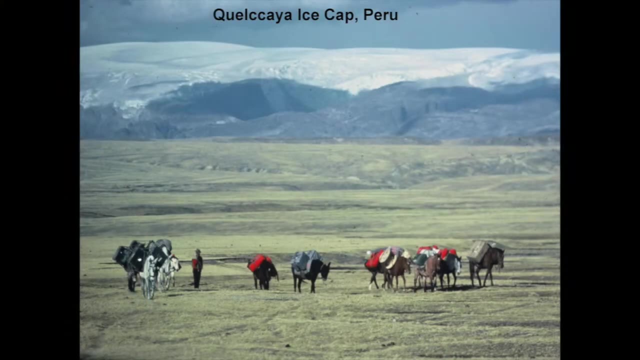 what it should be at this time of year. So even though they've had some storms there, it has not alleviated that drought. If you look at weather catastrophes around the world from 1980 to 2012,, you can see these are storm related, weather related catastrophes. You can see how they're increasing And if you look at the cost of those, in the last ten years that's averaged about 184 billion dollars a year, of which 56 billion was covered by insurance. There's a lot of variability from year to year, depending on. 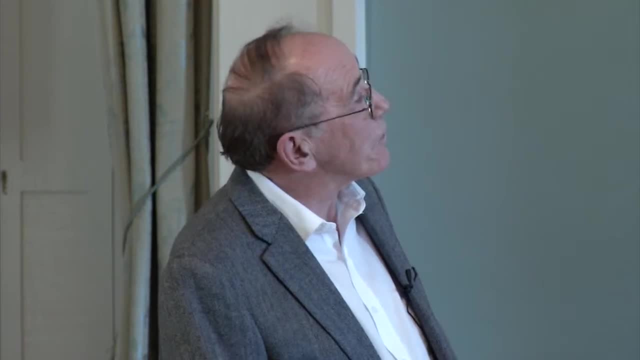 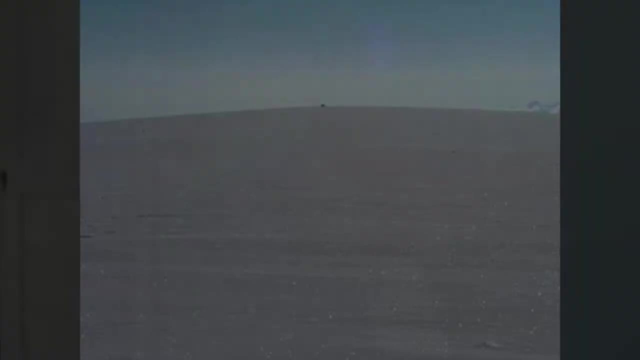 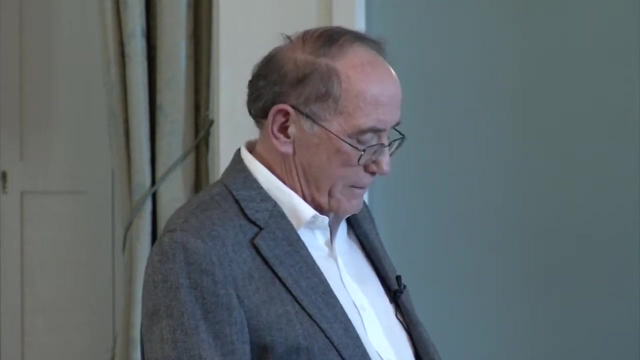 what storms and where they hit, as to what that actual cost is. But it brings back another human characteristic: Immediate consequences outweigh delayed consequences. When we start seeing these changes and the cost of those changes in the here and now, then the opinion on the climate change issues will. 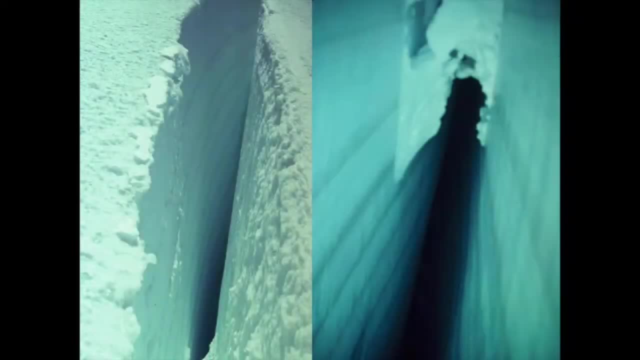 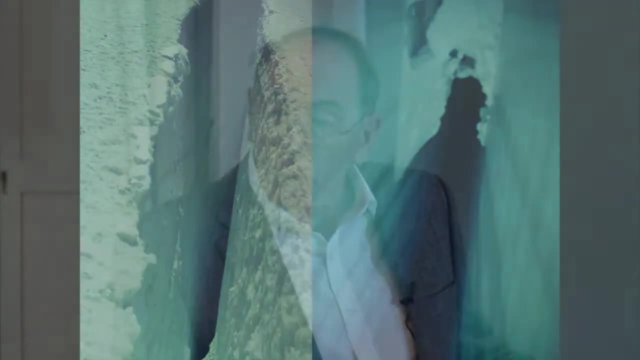 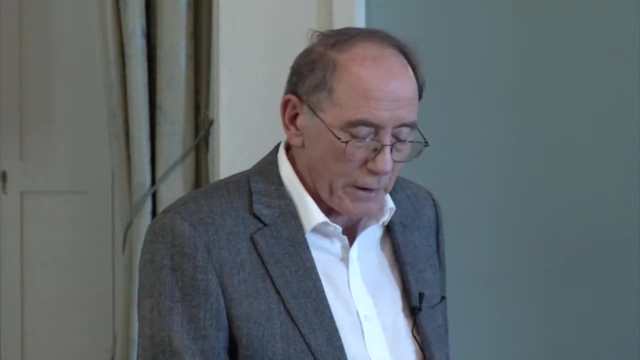 change. So, looking forward, I think there are three options out there. One of these is mitigation, which means taking measures to reduce the pace and the magnitude of change in a global climate that are caused by human activities, And here you can talk about reducing greenhouse gas. 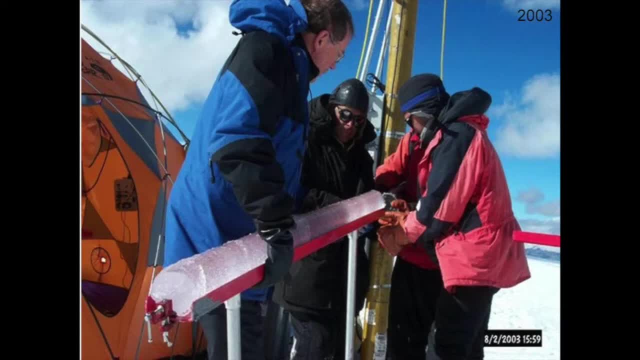 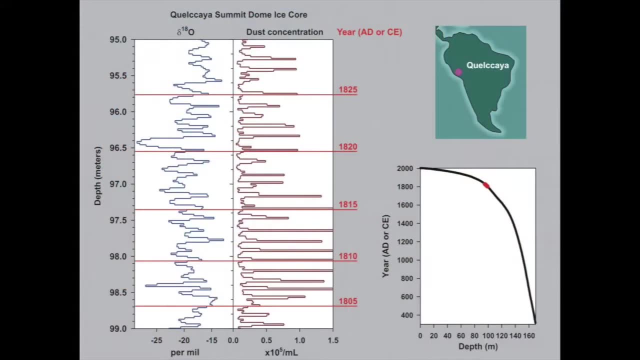 emissions. You can talk about enhancing the sinks for those emissions, taking them out of the atmosphere. We can actually talk about geoengineering to counteract the effects of greenhouse gases. We can talk about adaptation, which means taking measures to reduce the adverse impacts. 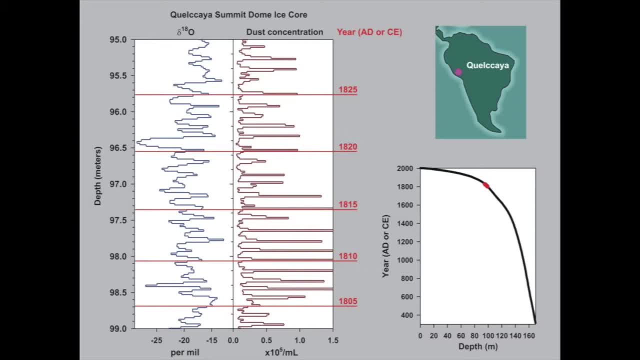 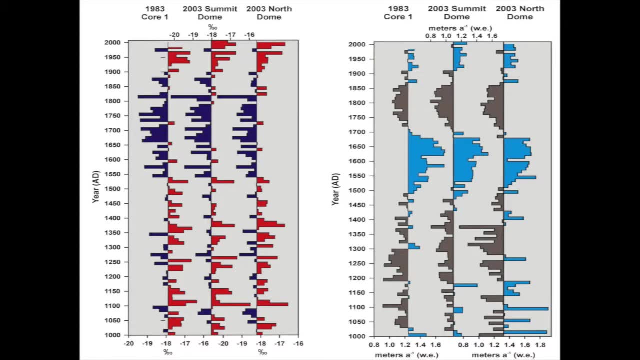 on human well-being that result from climate change. that do occur, And examples of adaptation include changing agriculture practices, strengthening defenses against climate related diseases, building more dams and dikes, But this is a moving target and we're not very good at regional prediction of changes. 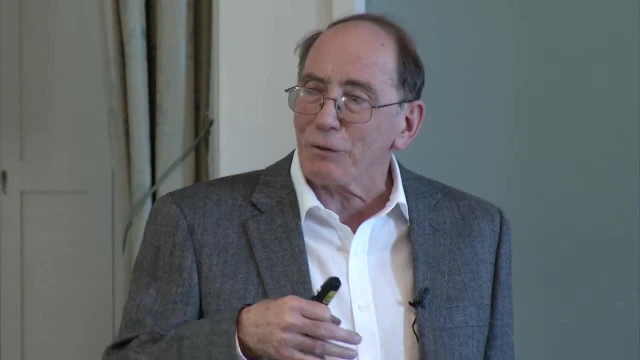 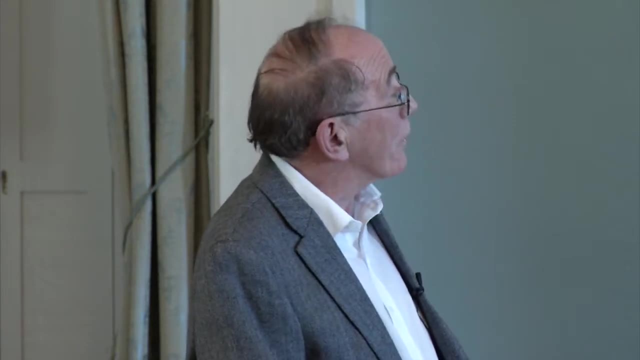 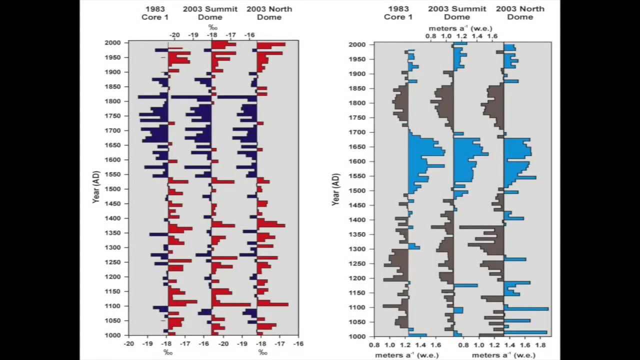 Then the last is suffering. This is the adverse impacts that are not avoided by either mitigation or adaptation, And I think these will be the options as we go forward. But there are positive things, and you mentioned this at the beginning and I think this is absolutely true. 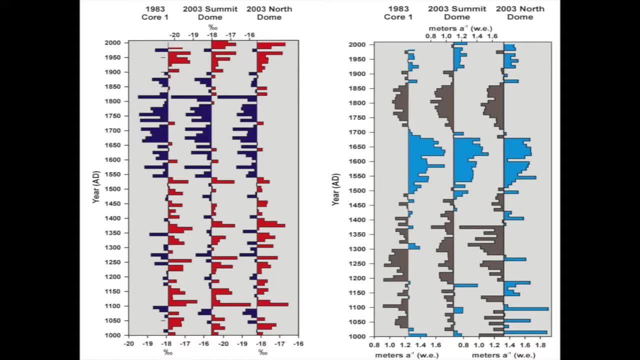 And I've been really impressed with the changes that are underway: Conservation, increased efficiencies, four-cylinder hybrids, cars, electric cars: We have Tesla, Google is going to produce an electric car. You have technology: we're going to have to. 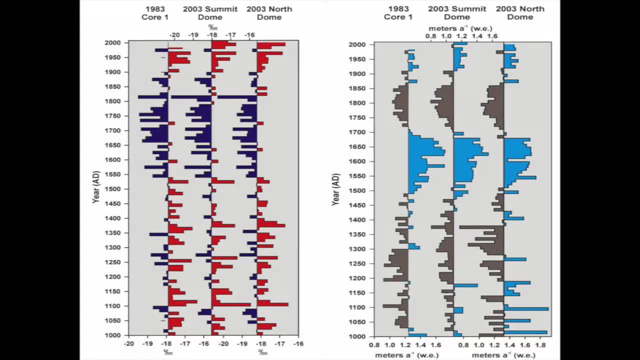 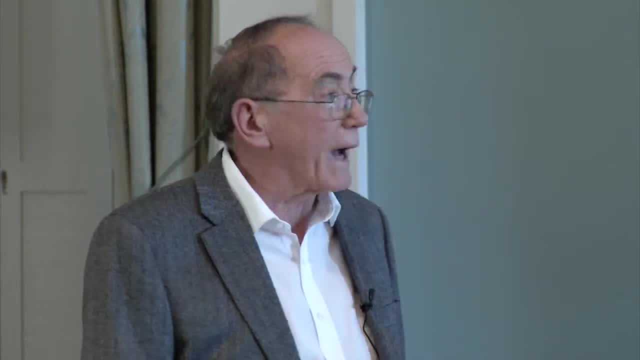 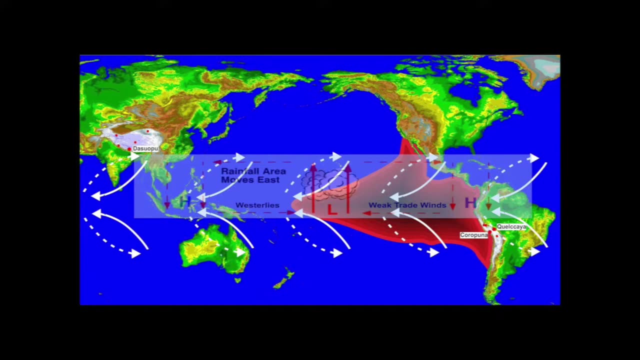 build a car, And I think this will be one of the answers to these changes: Fuel cells, zero emission coal burning power plants, solar, geothermal, ethanol, wind powered plants, Mass transits, light rail systems, buses, housing, design toward more. 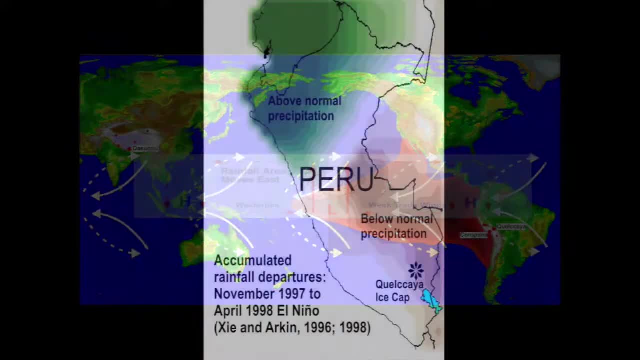 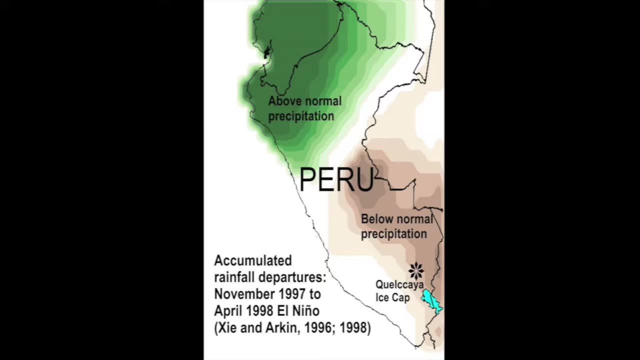 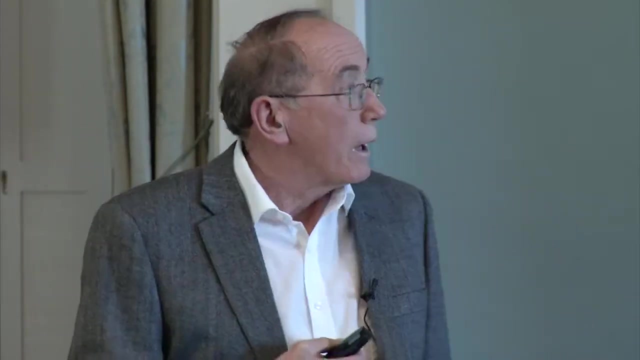 compact cities, development of nanotechnology, LED technology, But it doesn't mean too much if you just make a list of this. It's what we're actually doing that counts, And I come from Ohio State University- We're one of the largest public universities in the US- And 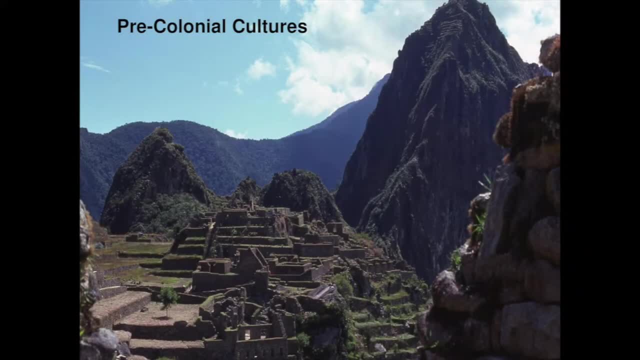 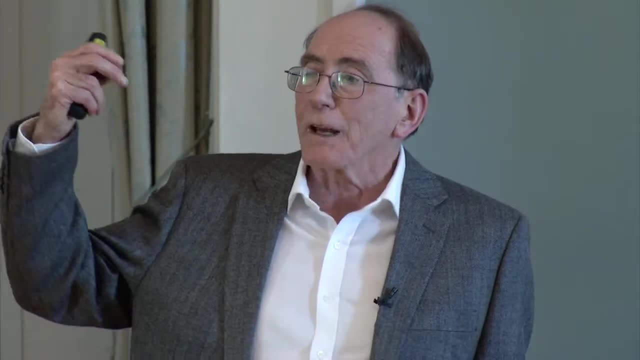 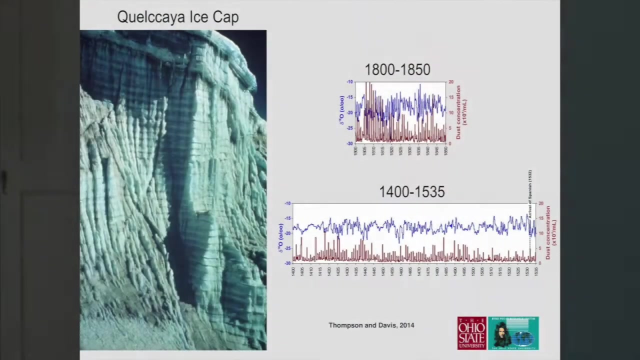 we have a very strong campaign for sustainability at the university. We have over 70 student organizations that are focusing on sustainability. We're ranked number three by EPA and the 20 largest universities are using green power. 25% of our electricity comes from wind. 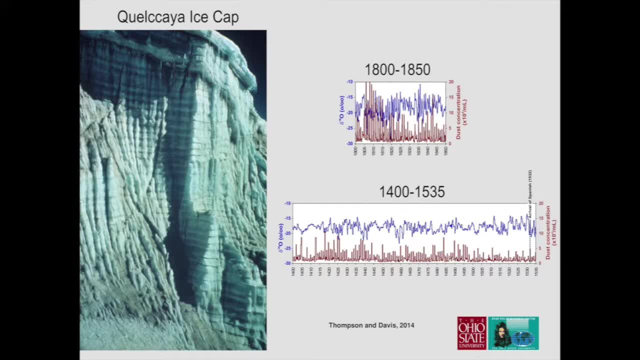 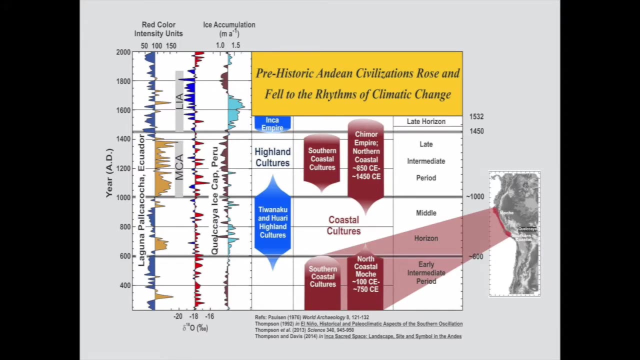 We recycle in that big stadium where we play football games, 98.2% of the waste that's generated. We put 7.1 million dollars into increasing efficiency and conservation infrastructure in our existing buildings And we have 37 alternative energy buses on campus. We are putting in these. 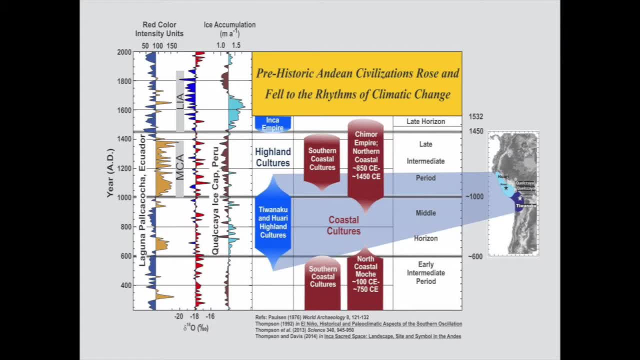 electric car charging stations. We hope to recycle 90% of the materials generated on campus by 2030. And in 2012, we planted 916 trees on the campus. So it's what we do, And the thing that I am really encouraged about is this is something that's coming from. 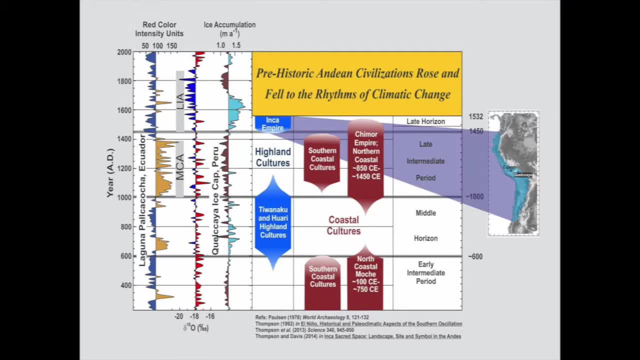 the bottom up. It's not coming from the top down, And I think this is the way the change will come. I want to tell a personal story that happened in 2011. And I think I understand skeptics much better after this. 20 years ago, I was 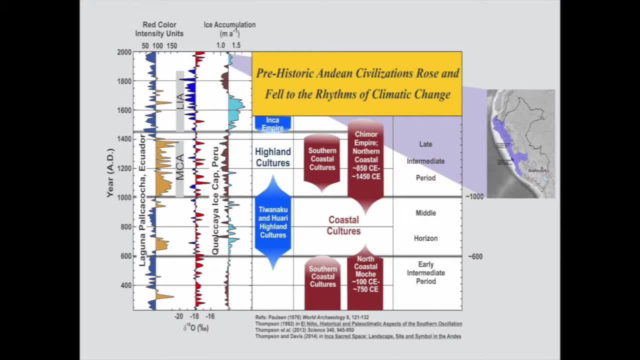 diagnosed with exercise induced asthma. And as I climbed these mountains, I noticed it was getting harder and harder. But the beauty was there was a medicine for that And you could take that and you could continue to do what you were doing. And in 2009, 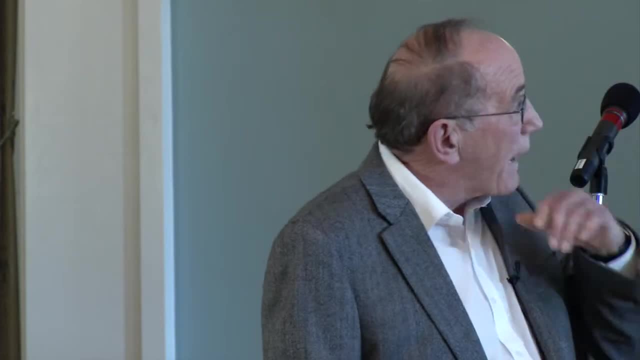 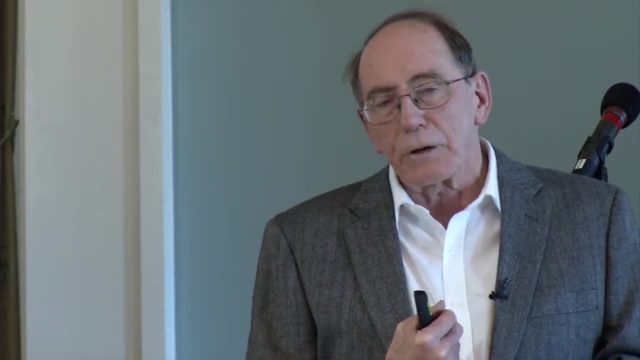 I was diagnosed with congestive heart failure And my cardiologist at Ohio State he said: Ronnie, this is what's going to happen. He said: you're on a threshold, You're going to drop to another threshold, But out here in the future you're going to have to have a heart transplant. 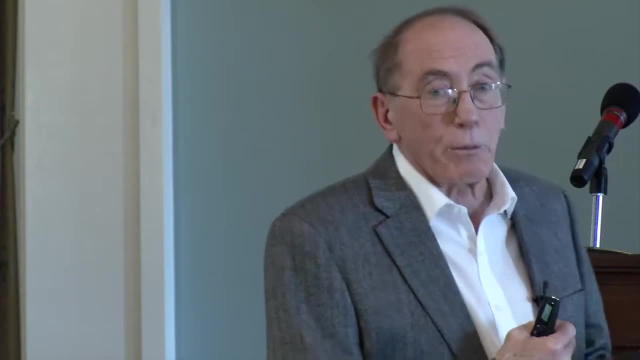 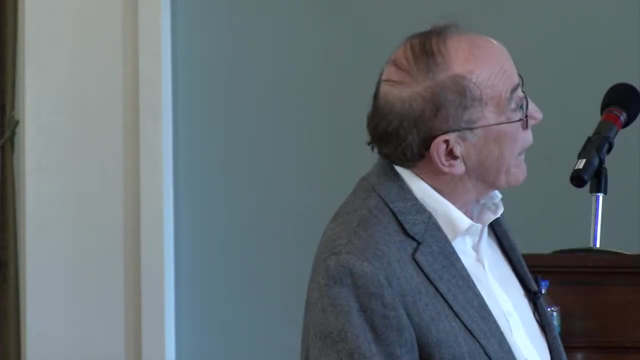 And I looked at him and I said: you're crazy. I have climbed the highest mountains in the world, This old heart works pretty well And you're going to tell me that I have to get a heart transplant. So I fought this for two years. 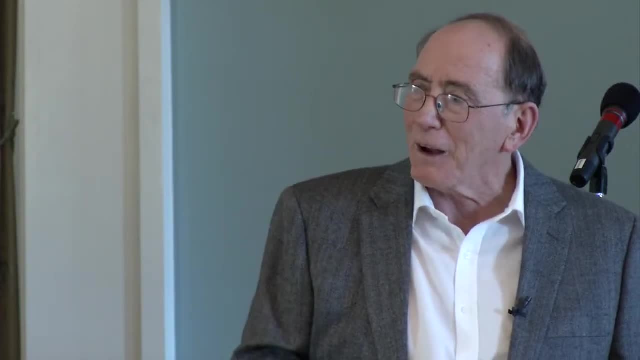 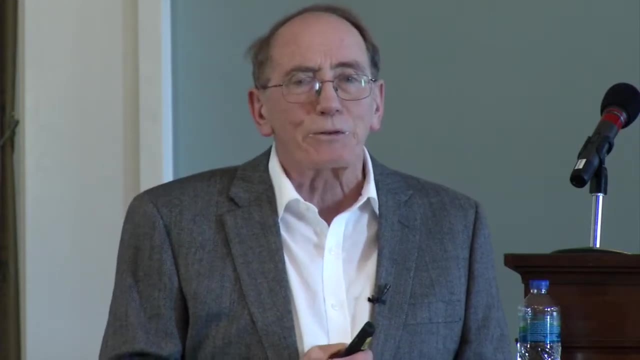 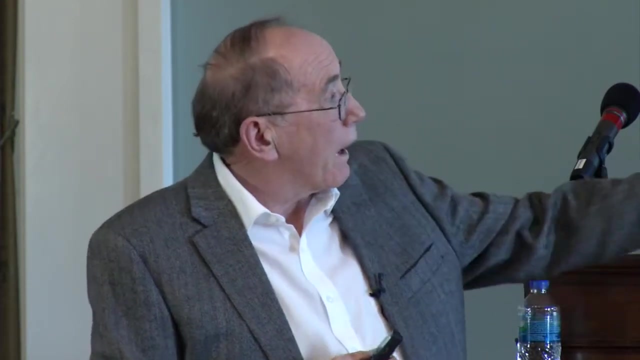 And I was on this drill site in 2011.. And I couldn't breathe to get from the tent to the drill site And when I got back home I went directly to the emergency room. I was on a heart pump, Then I put in an LVAD. 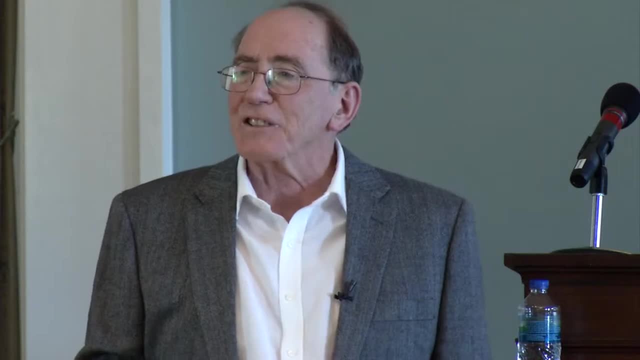 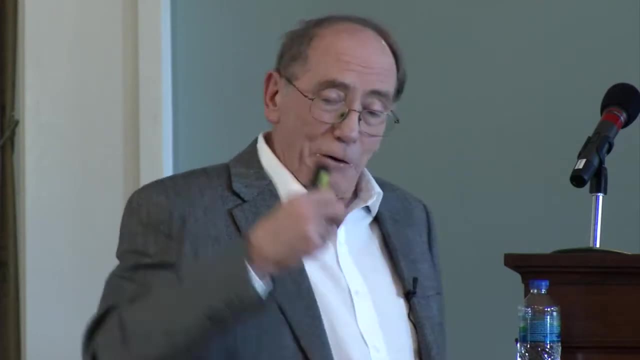 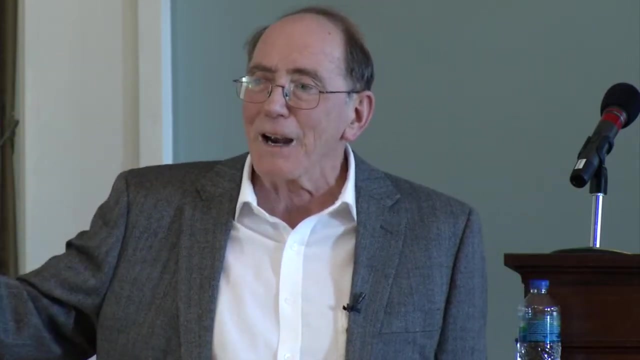 An LVAD is a turbine they put in your own heart that runs on electricity. You have batteries, you run in the day and at night you plug into the wall And it really gives you a new meaning of sustainable power, And this was in April of 2012.. 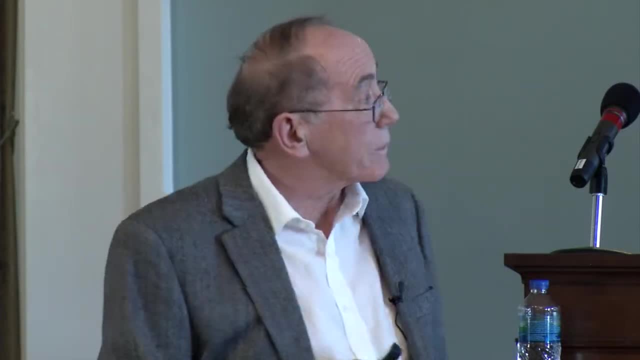 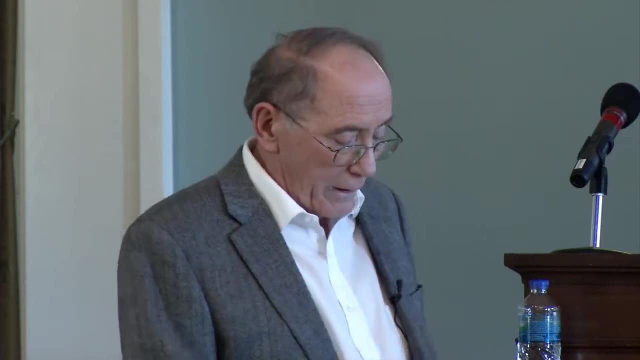 Ellen and I received the Franklin Medal for science- environmental science- And to go there I had to go off the transplant list, because you can't be more than two hours from the hospital if you're on the list, But this was going to take four days to go up. And so they took me off the list. I came back on a Saturday, And on Tuesday I got the call that they had found a match, And I went in in the morning, and by the next day I had a new heart. And then, one year later, I was back at 20,000 feet on the Zangsar Glacier in central Tibet. Now, the reason I tell this story is that if you think about climate change issues, there are a lot of people who we've been producing fossil fuels for a hundred years. And a lot of people are making money from this, And there's infrastructure and investments. And then when suddenly we realize that this is harming the environment and we're changing the climate of the planet, our first reaction as human beings is to deny it. But I think at the end of the day, it really doesn't matter what I think or you think. It's only what is, And what is is a matter of physics and chemistry, And at the end of the day, we will deal with it Because we'll have no choice. So when I look at the 21st century, I think our biggest challenges are learning how to get along with each other on this planet, And you can question how well we do that today or even in the past, But the other part is learning how to get along with the planet on which we depend. for our life and the quality of life, And these two challenges deal with human behavior and therefore they're very closely related. So let me close with this view of the world, If we've learned anything from our international space programs, how special this planet is for life as we know it. And when it comes to global climate change, nature's really the timekeeper on that, And none of us are wise enough to know how much time we have to make a change. But we do have good evidence that that clock is ticking And we need to get on with bringing about. these changes. So I want to conclude with this And I would like to. I have a very short, 16 minute video just was produced And it's by Ethan Steinman And it's about people who live in the Andes, And I'm just going to show you a very small section from Peru, But it's very important to understand that we share this planet with a lot of other people whose lives are also impacted by these changes. Thank you, Okay, thank you, Lonnie. You've done a really great job of sharing your personal research and what it's meant. to the climate record And giving us some very powerful images and information about how rapidly climate is changing in the last couple of decades And accelerating and also putting a human face on this climate change, And it certainly sets a great tone for this meeting. I think this meeting is all about those conversations that will take place around this. I think it's been a long time here, But we certainly want to entertain. I'm sure there's lots of questions, So we're going to take about five minutes or so. for questions And then people can come up maybe afterwards and ask any more. Yes, It takes time. I mean these smaller glaciers in the mountains. they respond first to change. They're not that big, But you talk about a Greenland Ice Sheet or Antarctic Ice Sheet. it takes a long time to warm them up, get them moving and see the change taking place. So every glacier, depending on its size and its thickness, has a different response time to these changes. But because they're so big once you get them moving, it's very difficult to reverse that trend. It's an important question. Other questions. Thank you for a brilliant presentation. I'm a city councilman here at Iowa, City Manager Jim, Three years ago, four years ago, when I was running for office, I was talking. to a local developer And I expressed to him my concern about climate change. He basically said: I don't have time to think about climate change. Besides, I don't trust anything coming from the federal government. One of the things that makes me think about is how developers and others who are really focused on operating successfully in the market economy do not face. they don't see prices that reflect the consequences of burning CO2.. It's the biggest negative externality there is in markets. So I'm wondering about that You really didn't mention. market economies or a deeper level of capitalism. You didn't mention that- about how it's a real primary driver in terms of the production and use of fossil fuels, et cetera, and taking us down this road. So I'm wondering what you think about what needs to be done in terms of affecting the markets, so that the developer and others like him that I talked to will actually adapt, change their behavior to reduce our carbon dioxide emissions. I think it's a very important question. I have issues with market based economies. We see this now in universities. What happens in a market based economy is that things that can make money prosper and things that don't make money don't. There are a lot of very important things about human history that we need to know, that need to be supported, and the people that do those type. of research need to be supported. But when you look at the marketplace, it's the real cost: understanding the cost that if you're a developer and you lose your development because of an extreme event, when these extreme things happen and you spent your life working for making this profit and growing and in 15 seconds, a couple of hours, it's all gone. then your view of the world actually changes And as we have more and more of these extreme events, more and more people get impacted and they question: is this a sound way to move forward? I mean, I showed that we have 7.3 billion people on the planet and that's growing, but consumption and consumerism is growing 10 times faster than that as new countries come online. and can we sustain that? I think we need to start thinking about. sustainability. How do you have a good lifestyle and you maintain it for the maximum number of people on this planet? If you ever end up in a hospital bed and you're on this edge between life and death, what you realize is all the resources, all the money, anything you've accumulated. in this life really doesn't matter. What really matters are your family, your friends and your colleagues And the difference that you were able to make in the lives of people in the life that you lived, And the rest of it to me is. I think our value system needs to be adjusted. What's important- I think that's a good point to maybe take forward from this lecture today, and I think the other thing we can think about is that, Lonnie, you've done a really great job. in informing us, empowering us, and I think we can keep this in mind. Iowa's pretty special. We're going to have a whole bunch of people tromping through this state wanting to be president of this country and wanting our votes. I think this is one of those questions. that we can be asking: Are they informed? Where do they stand? We can help ask them those questions and it can help shape our opinion. So I think that what you just said there is. we can carry that forward. It's probably a good time and